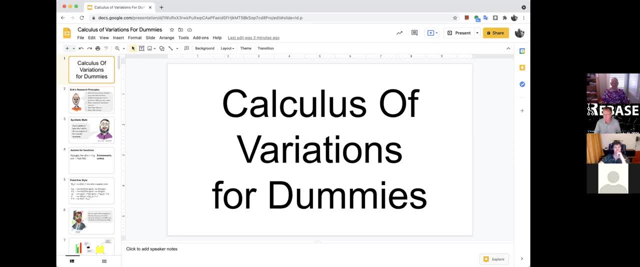 chicago with splash again. um, it's a great pleasure to have eric and alex here. so, um, eric has done an amazing amount of work in computing. he started in 86 with a paper on petri net models for the lambda calculus. i'm sure that not everybody knew that i like his paper paper. 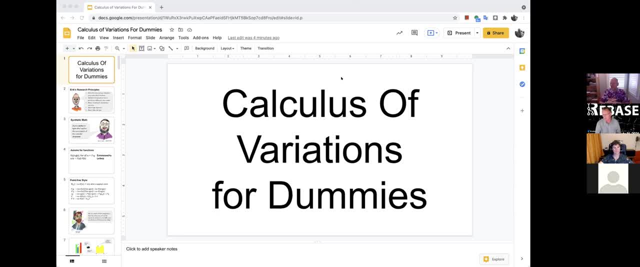 titles: bananas in space, one of my favorites, his work on haskell um, his work on links, link on rx, and now apparently he is all in machine learning, aren't you um? and alex. alex got his phd at epfl, i believe, with martin odersky, works on concurrency for scala, on reactive programming, and now he joined oracle. and 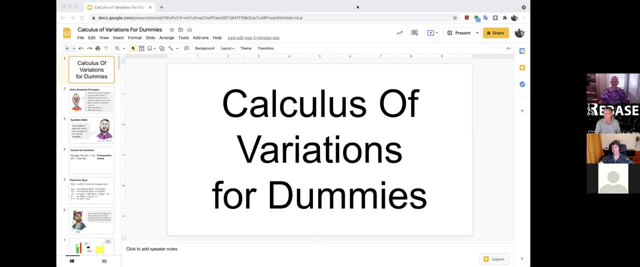 he's working on with the crawl vm and on all sorts of interesting lower level topics that we'll hear more about later. so a few words about the format of those two hours we have. um, what we'll do is we'll start with a talk by eric and then, once eric's talks finishes, we'll- uh let alex give a few words of. 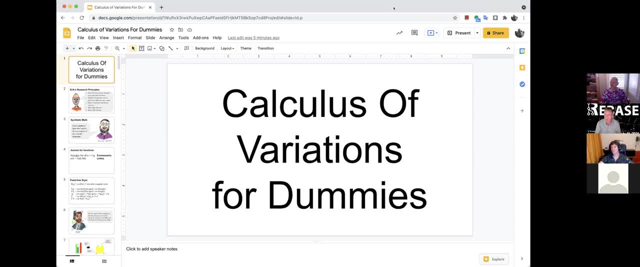 you know either a position statement or response to what he's heard and then we will have a discussion that will intermingle audience questions and you know just our two participants duking it out. if you have questions during the talk, put them in the chat. i will read them as a when appropriate. 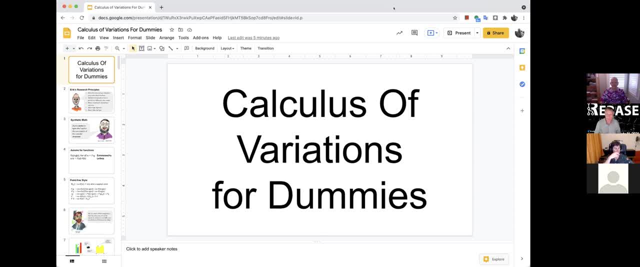 and maybe some of them. i leave for the discussion. if i forget your question, just repost it, because it can get a bit jumbled up on on the chat part, and i think that's all i have to say. so, eric, the floor is yours. uh, thank you, um, can everybody see my screen? i don't see my screen on the. on the. 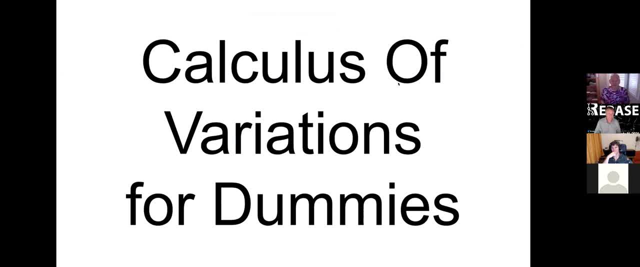 screen. but just okay, that's good. so, yeah, um, today i want to give you a little bit of um, a sense of the calculus of variations, um, and in particular i'm going to get related to functional programming and machine learning, um, so here are, like, the principles behind this talk and behind my work. 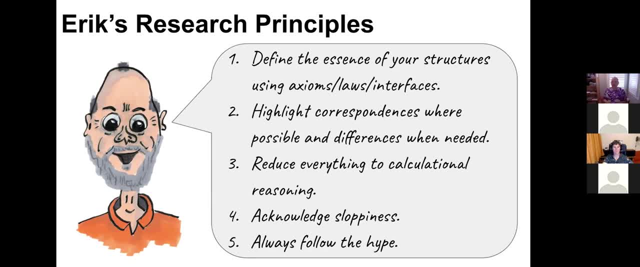 in general, um first is you define the essence of your structures using axioms, laws and interfaces. um second, you get, like you know, i like to kind of highlight um similarities and differences where needed, but mostly i like to highlight um correspondences. and the third principle here is i want to reduce everything to calculational reasoning, making it. 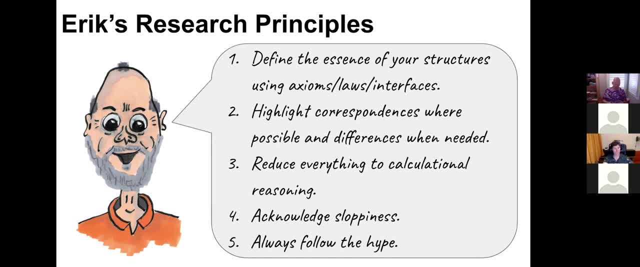 super simple, that even a, a kindergartner, can do these things, and that means that there should be no intuition involved, just applying calculations to the structure of the structure of the structure, as well as over 계산 with, etc. which means they can stop doing it. they can still use. 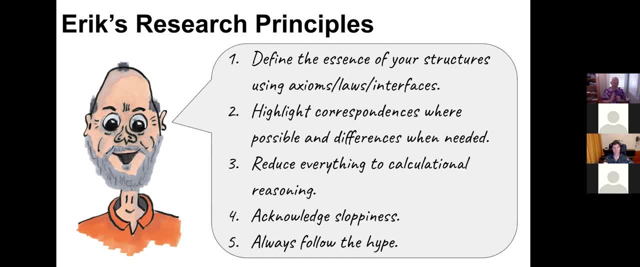 the calculus ofравn Crush and practice computational rules. that's my goal. so whenever you see a calculation in this talk, don't try to understand it, just try to look at it syntactically, where we're just kept like doing equational reasoning. um, i love being sloppy and 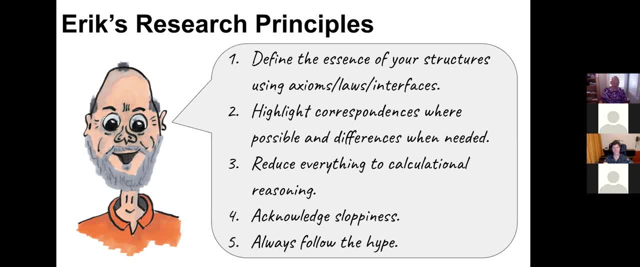 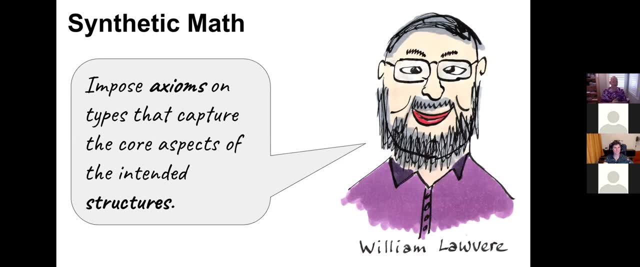 i'm going to acknowledge where i'm sloppy and, of course, this is got like you know. another thing always follows the hype. that's why i'm doing machine learning now, because that is the current type. um, all right, so, um, this thing of like defining your intentions using acsiums, it's not in this. 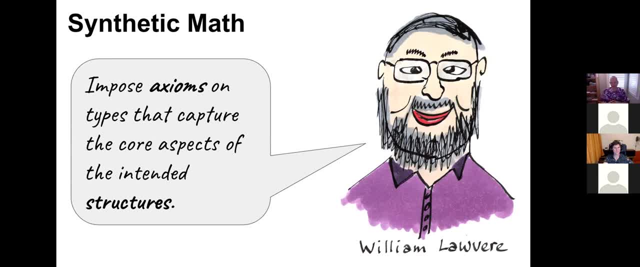 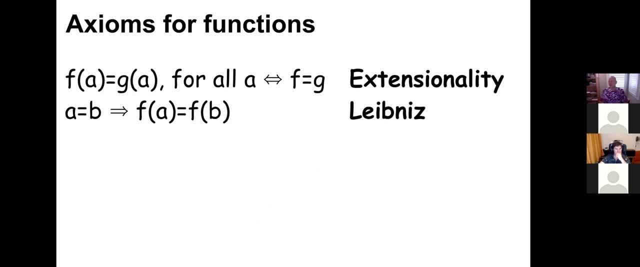 new. It's called synthetic math And William Lover is one of the category theorists that's doing a lot of that. So there's nothing original here. And in this talk we'll be talking a lot about functions, And here are some of the rules I'm using for functions. So two functions are: 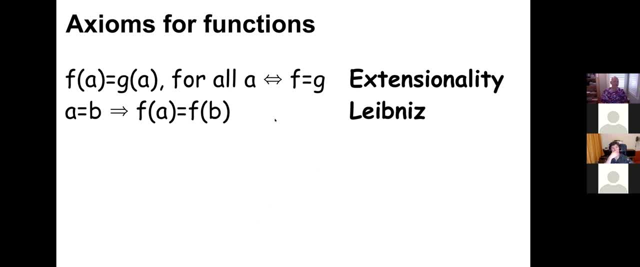 equal. If you apply them to any argument, the results are the same. Of course, that's not a definition of function equality. that will work when you define it in a programming language, But since we're doing math, this is perfectly valid. And then the other thing that's sometimes called 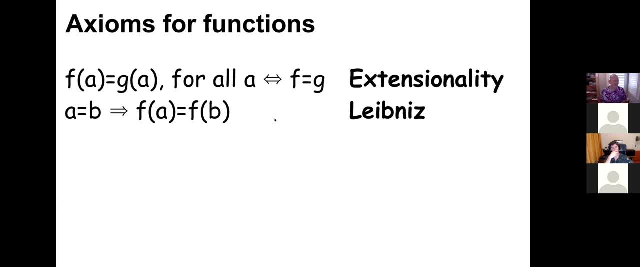 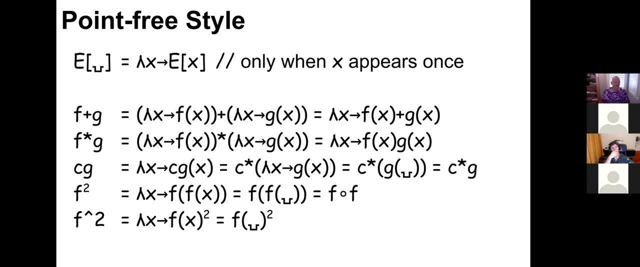 Leibniz rule by folks like Edgar Dextra is: if you apply a function to the same arguments, then the results are the same. Another thing that we're going to do is to use point-free style, So that means that we're trying to avoid lambda expressions but overload, say addition and 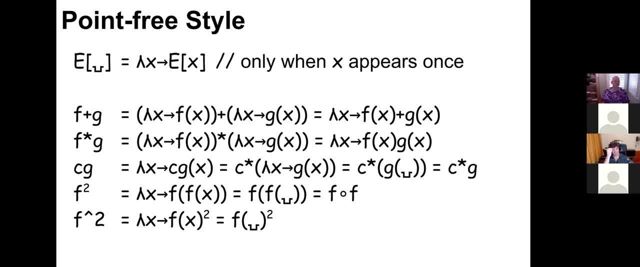 multiplication over functions, And then we'll also use here- I think it's kind of like Scala convention, where we got, like, you know, if we have an expression, we can leave like a placeholder in there, And that is kind of like, you know, an implicit function, So we don't need to name. 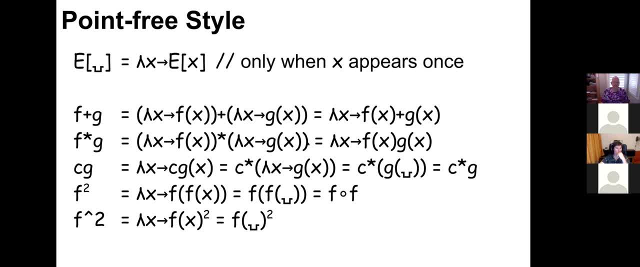 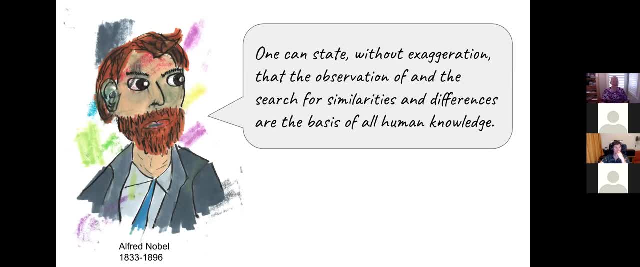 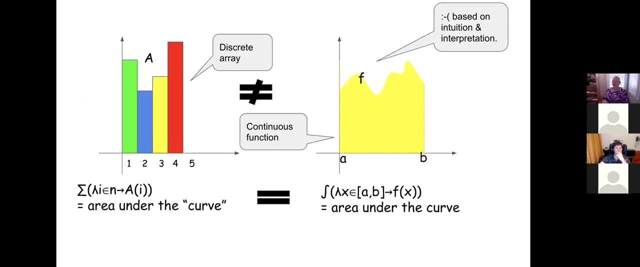 that parameter. So these are kind of like things that we'll be using as we go. This idea of kind of like you know, looking for similarities and differences is also nothing new, And this is a quote from Alfred Nobel. Let's look at an example of things that look like you know. 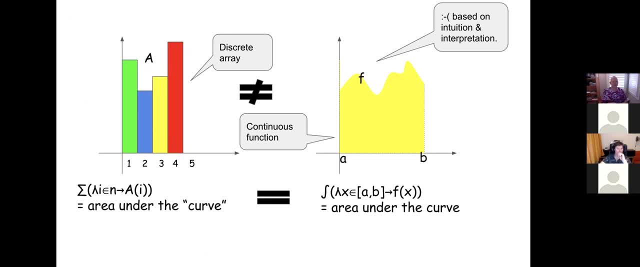 different but are really the same, And later in this talk we'll actually make this formal. Now it's based on intuition, which I don't like, And the goal will be to get like, just make this formal. So on the left here, you see a discrete array of numbers, And on the right, you see a 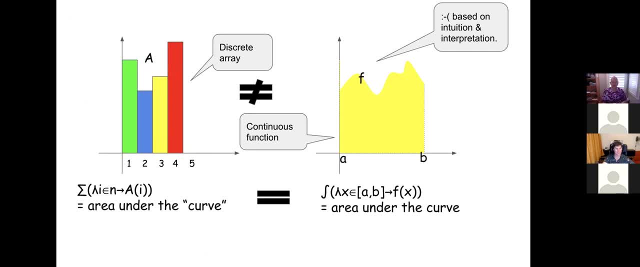 continuous partial function defined in the interval A to B, And if you sum up the bars, you get the area under the curve. And if you integrate in the interval, you get the area under the curve. And so these things are the same. They both are. 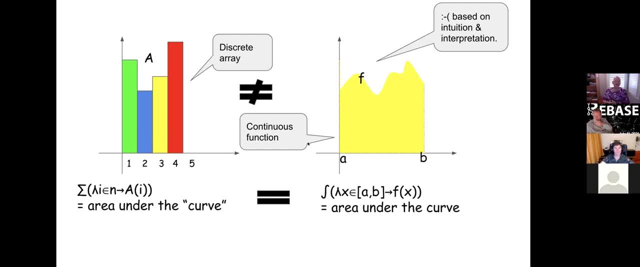 kind of like area under the curve where they look very different. right One is a discrete array, The other one is a continuous function. So we'll later we'll see that, like you know that we don't need any intuition, but this will follow by kind of like defining the right interface. that 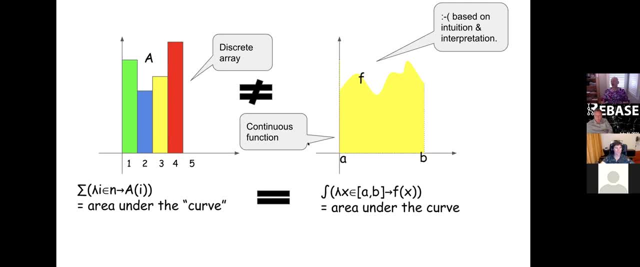 captures both of these structures, And then we'll see that, like you know that we don't need any intuition, And then this thing will fall out. So then like because I don't trust my intuition, because I'm sloppy, So and that's a great thing- that when we don't need that, 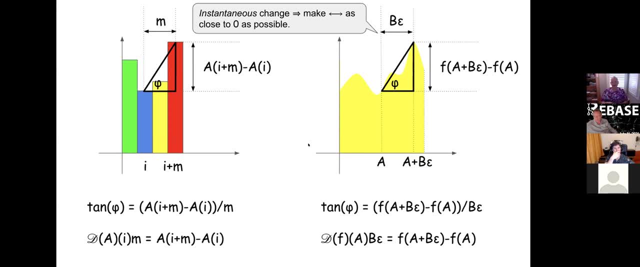 intuition. Here's another thing- And we're going to be talking a lot about this- is derivatives, And derivatives are often defined as the tangent on a graph, like a tangent line, And if you look at the discrete case, we're drawing the triangle there. The tangent of phi is: 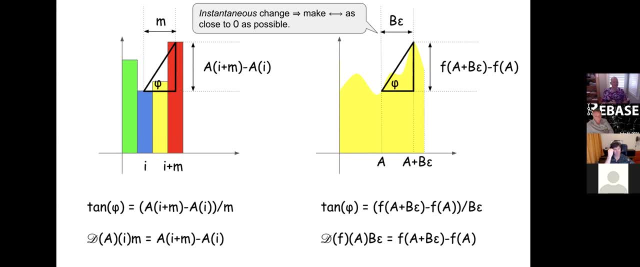 like this term there, And then we can define a notion of derivative, like discrete derivative, as follows: And then on the right, we're defining the tangent of the triangle there And what we're going to do is we're trying to make this get like. you know, the width of b times epsilon, as 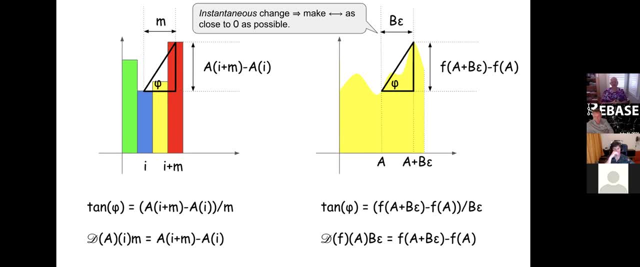 small as possible, And right now that's also defined intuitively. What does small as possible mean? Well, we're going to make that the tangent of phi, And then we're going to define the tangent of b times epsilon as small as possible. And what we're going to do is we're trying to make that. 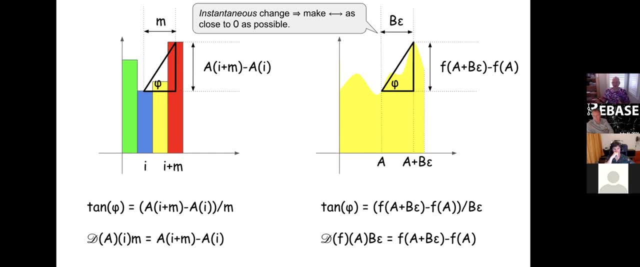 more precise later. But here again, like we can define a notion of derivative, that's like defined on the bottom, right there, And then later we'll make sure that, like all intuition is gone, We don't really want to get like think of these things in terms of graphs, We want to 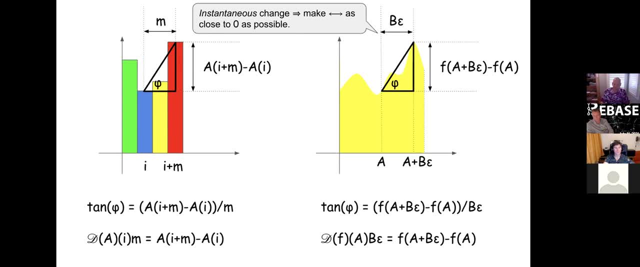 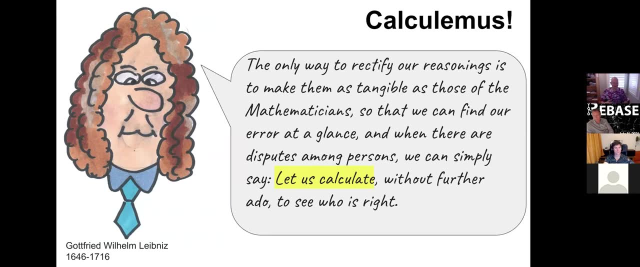 think of them in terms of equations like the one at the bottom. And again, this is not a new thing either, And Leibniz, in somewhere in like you know, 17-something early 18th century 1800s, already said this: like you know, we should just calculate in order to get like. 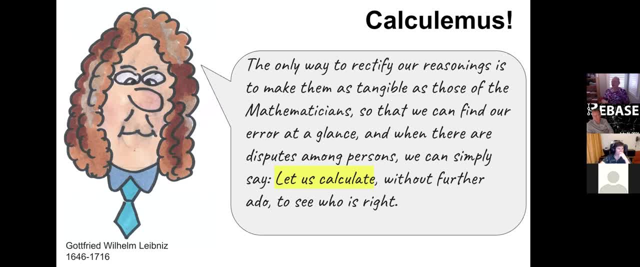 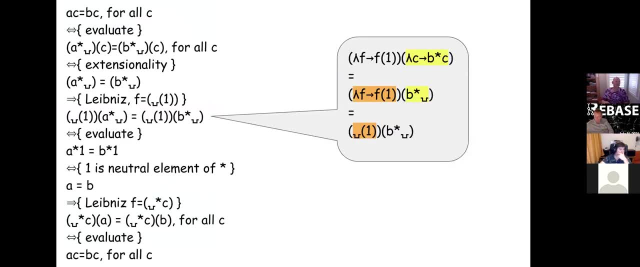 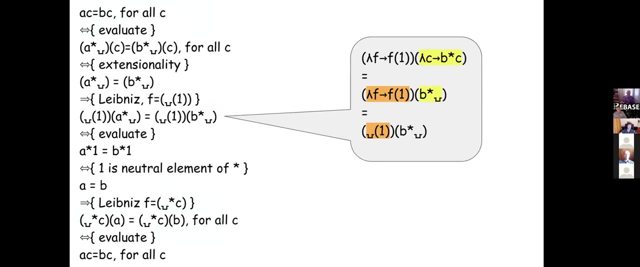 show stuff, And so in some sense I'm really old-fashioned. I'm just following Leibniz's proposal here. Here's an example of a derivation. I want to show that if a times c equals b, times c for all c, then a equals b, And you don't need to follow this reasoning at all, Just. 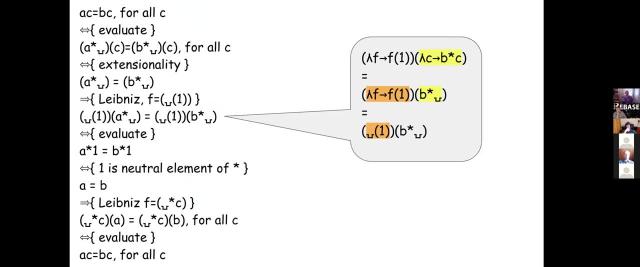 look at the derivation And you can see that the derivation is the derivation of a times c for all c, And you can look at it, It's like all just applying rules And then, like you know, I show here my circular implication that it's if and only if, because Leibniz's rule only has 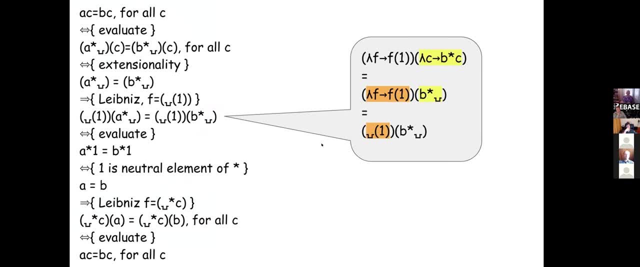 a simple implication. But this is the kind of reasoning when I mean like calculational reasoning, right, I just want to kind of, like you know, do syntactic transformations that require no thinking. I just want to apply them like mechanically over and over to prove stuff. 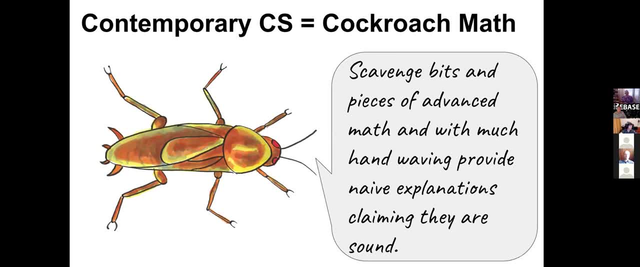 Then the other thing here I must say is that when I talk about sloppiness, I think most of contemporary computer scientists is sloppy. I call it cockroach math, where you scavenge bits and pieces of advanced maths And with much hand-waving you provide naive explanations and 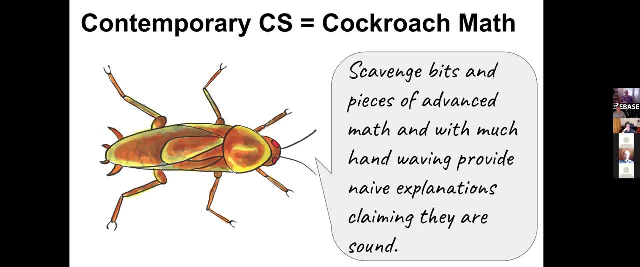 claiming that they're sound, And I won't be any better than that. right, I will be better than that. I will be doing like cockroach math here. And what do I mean by this? Let's make this a little. 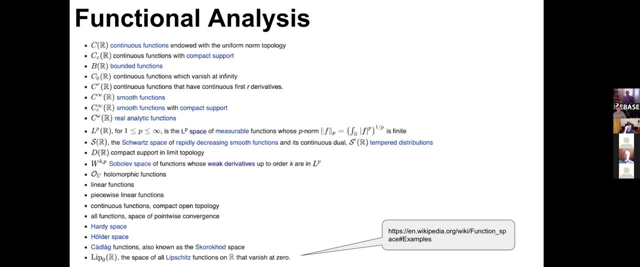 bit more concrete If you look at functional analysis, which is really what this talk is about. mathematicians distinguish between all kinds of functions. They're really precise about the notion of function space that they're working on. And here's like I don't know. 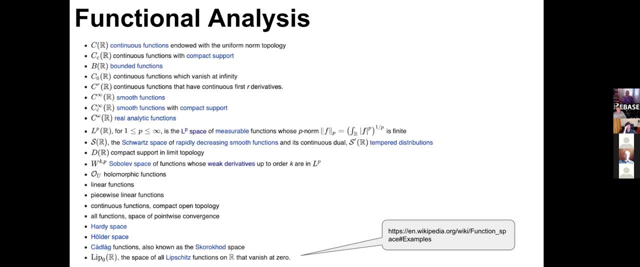 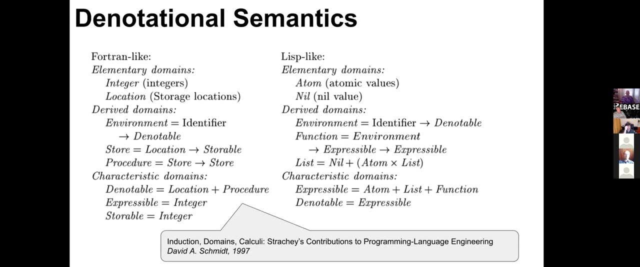 there's like 20 or 30 here that they distinguish. And in the early days of computer science, when denotational semantics was still in fashion, people did that as well. Like, if you read Strachey's original work, he was saying: tell me your semantic domain and I can like you know. 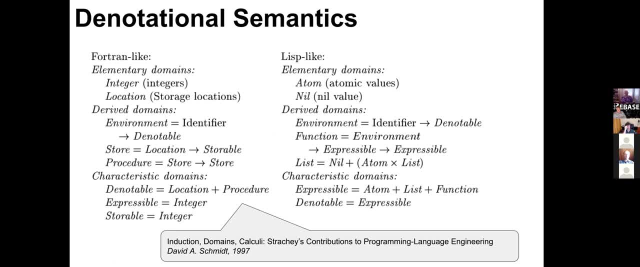 know everything about your language. The syntax doesn't matter. These days people are not at all precise anymore about their semantic domain, Or maybe. I think Jan maybe is when he talks about R, where it's like linear, And I think that's a good way to put it. I think it's a good way to 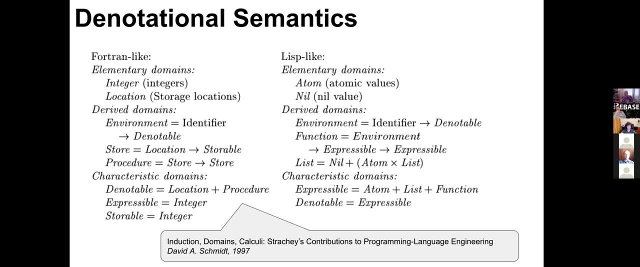 put it, I think it's easy or strict or whatever. But a lot of people say: oh, F-sharp is a functional language, It's much better than C-sharp, But if you look at the semantic domain, it's exactly the. 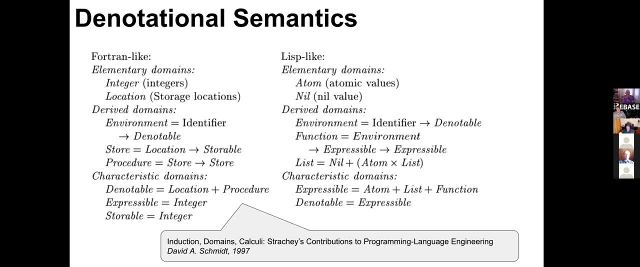 same because they run on the same VM. So there's really no semantic difference between these languages, It's only syntactic. If people look at Java, they don't really understand what is the function space that your Java programs live in, And so people are very sloppy. But it works. So 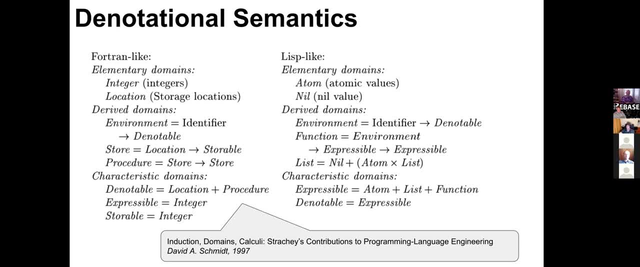 I'll be sloppy, But again, I think probably it's better to be way more precise. But what we'll do here? when I talk about functions, I'll wave my hands and say it's appropriately, like you know, picked from the. 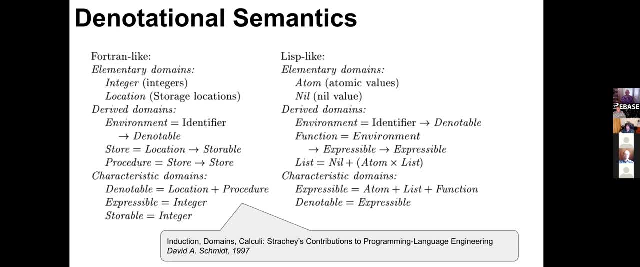 right set and it has all the properties that I like. But I'm not going to be precise about it, just like every no computer scientist is precise about the function space their programs work in. And then, lastly, talk about hype. 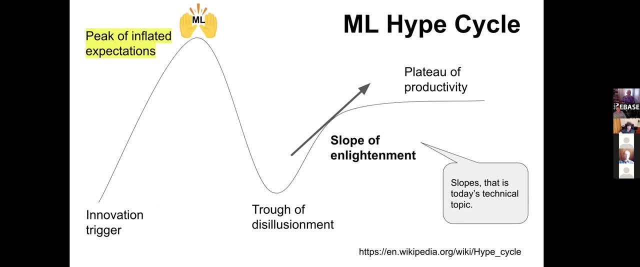 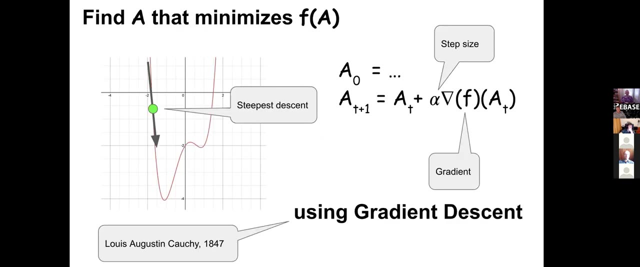 And well, ML is at the peak of inflated expectations, And so we'll be talking about machine learning today, And, and one of the things here is, like you know, we see here slope of enlightenment. well, slope, that is today's technical topic. So what, what we want to do, what is? 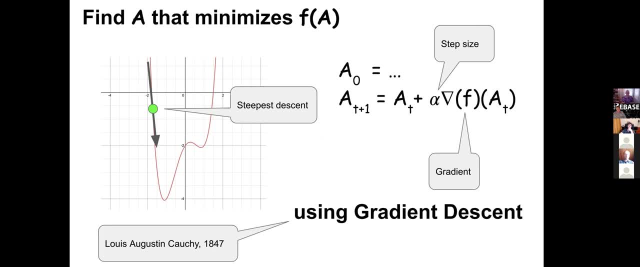 really machine learning. it's finding its function, minimization. And how do you find the minimum of a function? And we have here a little function here on the left, And what you do is you get like are at a point on the graph of the function, then you look at the. 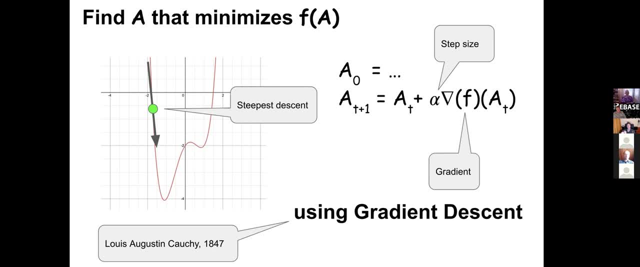 direction of steepest descent. you take a step and then you repeat that all over again. So that's the kind of little algorithm that's here on the right And this was invented by Gauci in, like you know, 1850, something. So this is really old. So a lot of the machine learning hype that we see today 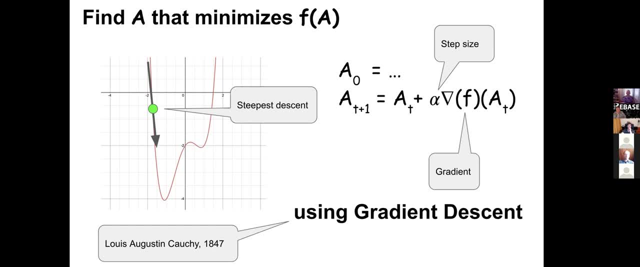 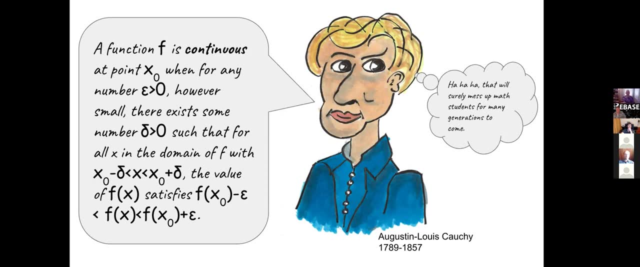 relies on ancient math from, like you know, from the 1900s And- and, by the way, Gauci is also this devil that gave us epsilon delta definitions of continuity, And this is something that we won't follow because we have something like much better. 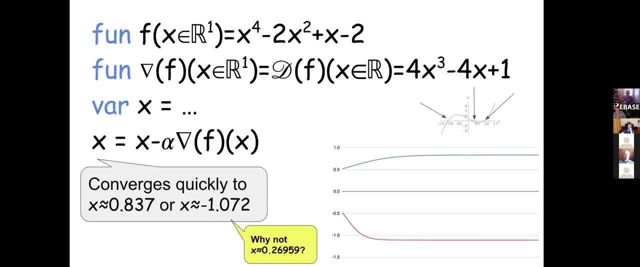 as we'll use. And so here's some kind of- like you know- full Kotlin code that shows how to do gradient descent and for the function that we had before. So there's the function and here's the derivative, And then we 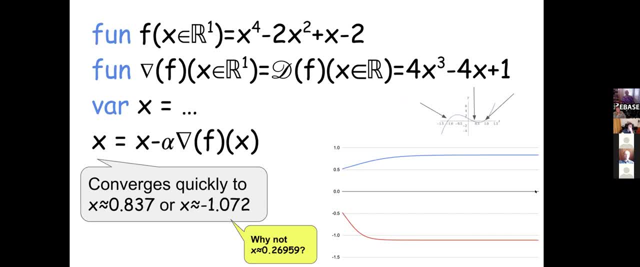 go in a loop and just update the value x And then you see here in the graph that, depending where you start, it either converges to 0.8,, which is this one, or it converts to minus one, like here, but it doesn't find that one. And then you 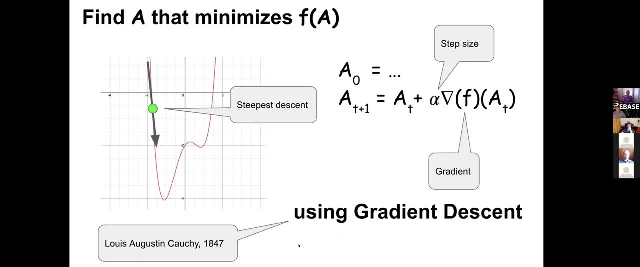 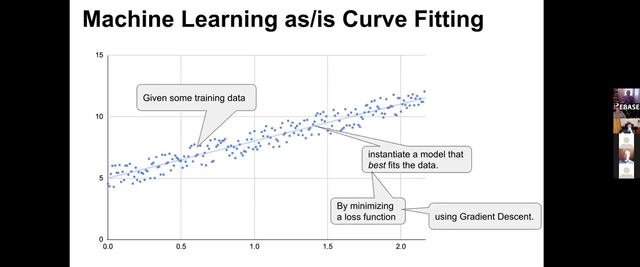 can ask yourself why not. Well, if you look at the graph here and where is it? It's, I forgot where it is, But anyway, here and that doesn't, it doesn't find it. So you can ask yourself why. that is where I leave that as a homework exercise, Anyway. 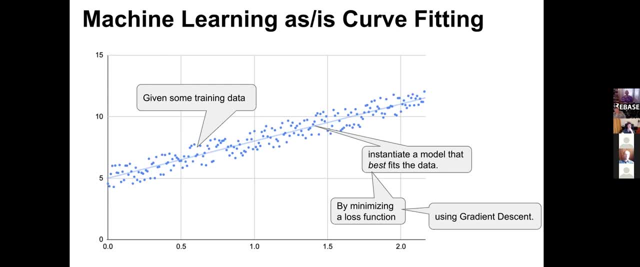 let's look at like machine learning now, And really I think machine learning is kind of like curve fitting: You have some training data and then you want to find a model that best fits the data. How do you do that? By minimizing a loss function that describes the distance between you. 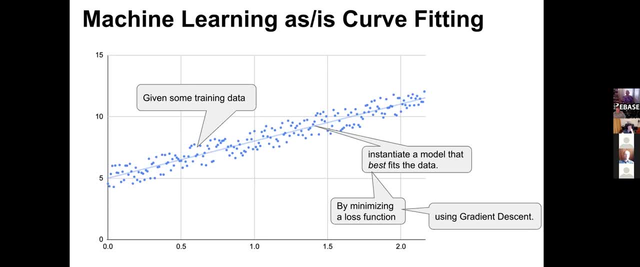 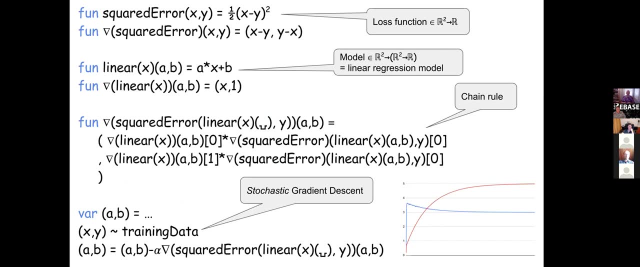 know your model and and the what you're computing and you do that by gradient descent And of examples you can use. what we did before was to use a square loss and then a linear regression model and and if you, if we do that here, we should see the code and then you can get like you know. 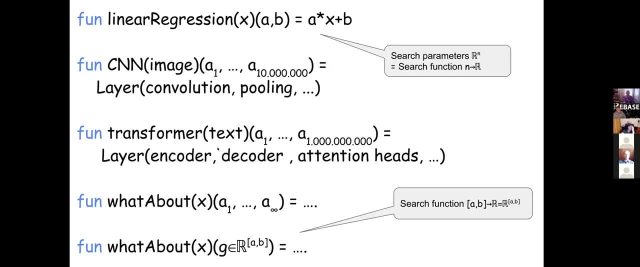 run this thing and it will find the values of the parameters here. now what people do is like: in this case, we have two parameters for linear regression. if you look at cnn's there people have, like you know, 10 million parameters, whatever, and they have like more complicated models that use convolution. 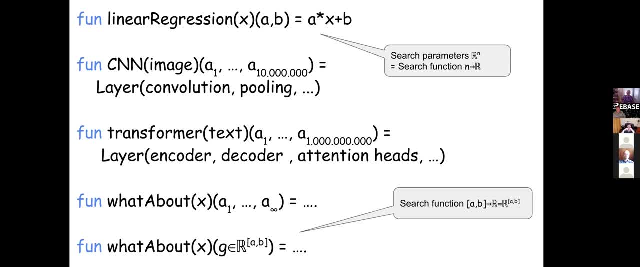 and pooling. then there's transformers that use a trillion or more parameters and they have like encoders, decoders, attention heads, and if you get like look at this and say like if we just increase the number of parameters, we can look at models that have an infinite number of parameters. 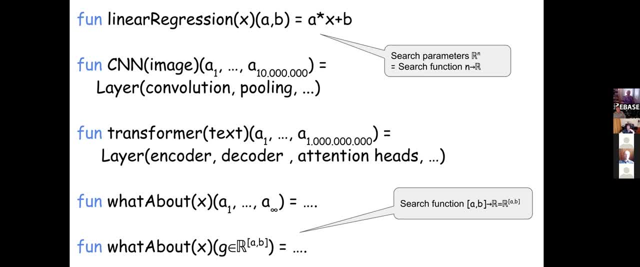 or, if we can like go even further, is: well, what is like? you know what is a? like a, a tuple of parameters, that's really a function from integers to values. what if we just replace that by a function from real numbers to real numbers and in some sense, now we're going from a parameter space of tuples or vectors or tensors. 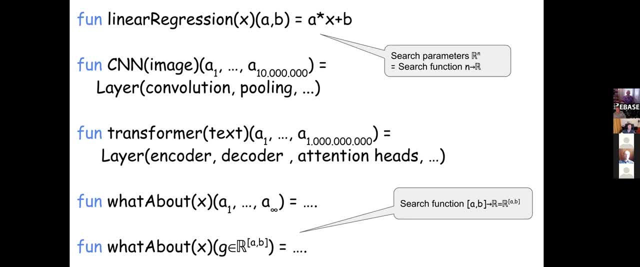 to a parameter space of functions, and that's really all what the calculus of variations is. so, again, it is focusing on what is similar, right like, if you look at it, and a finite tuple. that's a function, and now we generalize that to functions, not with integers as indices, but real numbers as 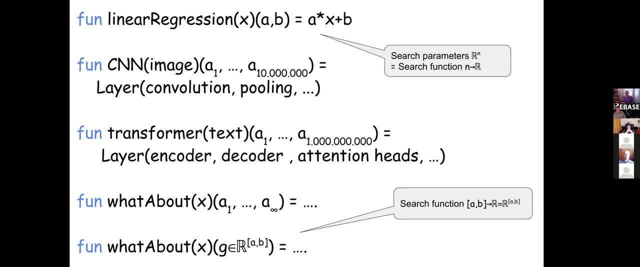 indices, and then we want to do exactly the same thing. so i think that's pretty beautiful, like focusing on what is similar instead of what's different. and now, why is it useful to get, like search for functions, um. so let's look at a few examples: um. 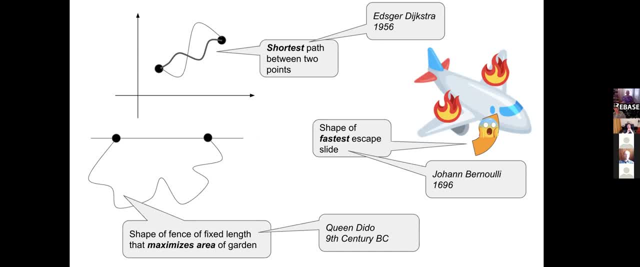 if i have two points and i want to find the shortest path between these two points, well, that path is described by a function, so i'm looking for the function, the minimum function, and that describes the path between these two points. um, of course, it's Tongue and Cheek that TeXtra had like invented that. 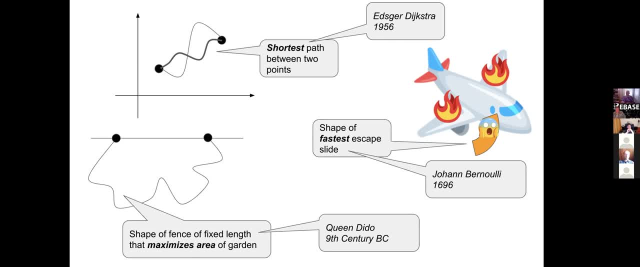 um, now, if you look at another one is, say that you want to design the shape of the slides to leave an airplane. what you want there is you won't have the shape that when you slide down below the çaqon it should stick in midway. it's as the same thing, this slide. now you need to release it to leave an airplane. 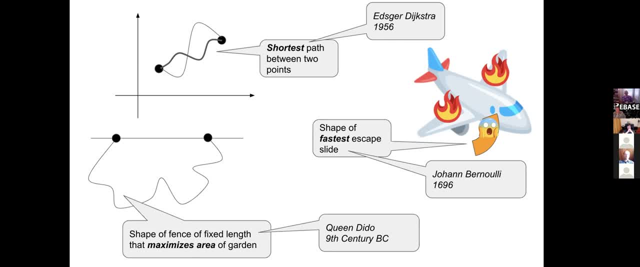 that when you slide down photographed, that understood what came from yourvens檸. that shape and the time it takes to go from the start to the end is minimized. so, again, like you're looking for a function- the shape- that function describes the shape of your slide and this was. 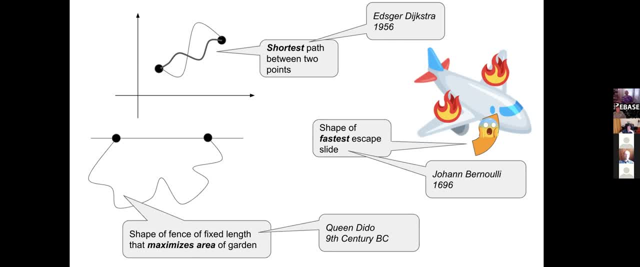 like posed in in 1696 by johan bernoulli, of course not in the context of slides to escape airplanes, burning airplanes, but it's. it's there as well. and then there's even like a much older thing where you're trying to and not minimize something, but maximize is say that you kind of like get a fixed. 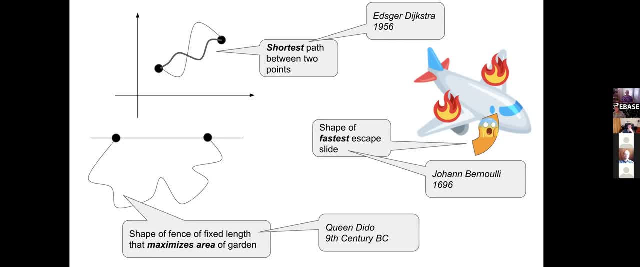 length fence, and now you want to find the, the area, the shape of that fence, to maximize the area of a garden. and again, like what you're doing here is, you're trying to find a function that maximizes the area. and here you're finding a function that maximizes the length, and here you're trying to. 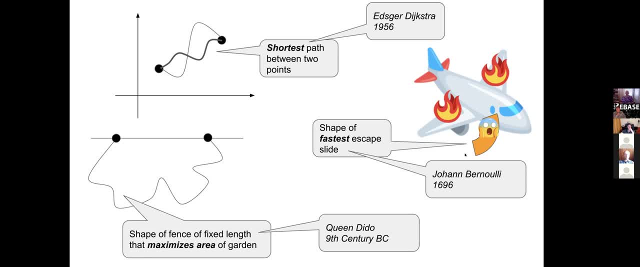 find a function that minimizes the the time to travel across that. so these are all kind of like you know, like interesting optimization problems that don't require you to search for a vector of parameters, but to find a function, all right. so, in order to get like you, 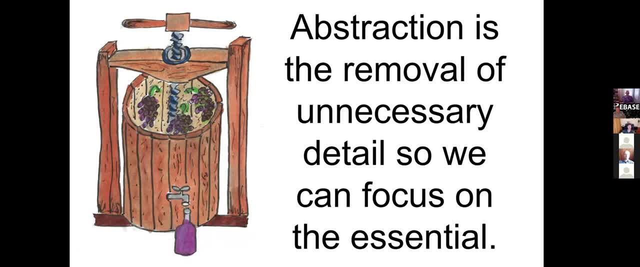 know, make progress. what we need to do is we need to do to find the underlying abstractions. what is, like, you know, the, the correspondence between all this- that we can describe this in an abstract way actually, but then I don't have a physical ways to provide that in my students- is anни, if you have, 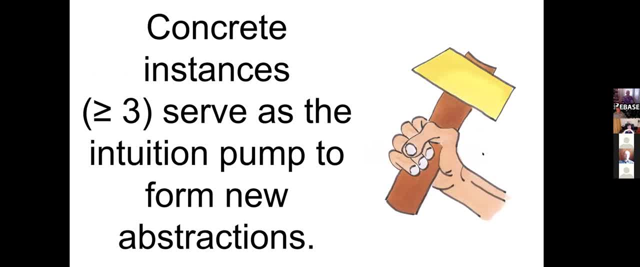 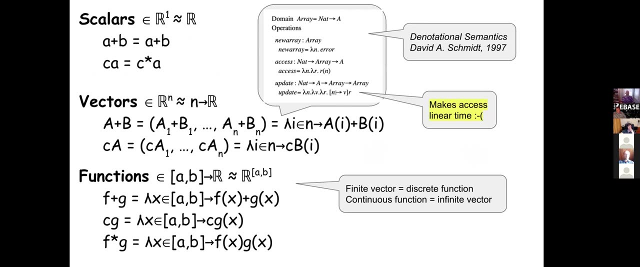 any time. uh to you can uh any time. so I'm going to take a few minutes in from the difficulty mode, as I mentioned. actually, I could maybe try to, if I have the time service, use it earlier. arm a- haven't had time for slides- option could help a little bit there. meaning that sometimes let's say, for instance, like: I guess like. 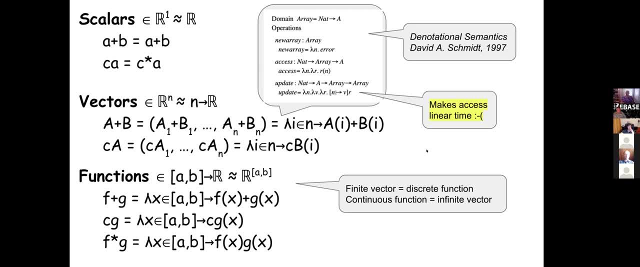 in Esper. here we might just maybe point out something like that, which is a fixing plan of length, one right, And in Haskell there's not even a one tuple, because they are the same as just scalar values And addition is just addition, Multiplication is just multiplication. 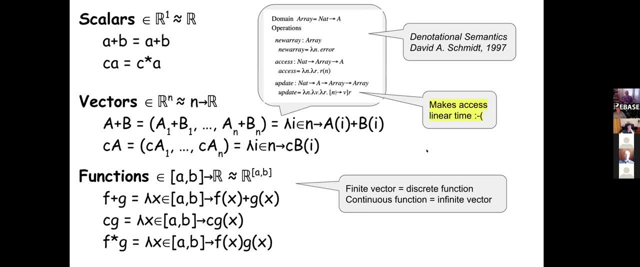 If I look at n tuples of real numbers, if I add them up, I add them up pairwise. But if you again, like you know, I am a big fan of denotational semantics. I don't know other people. 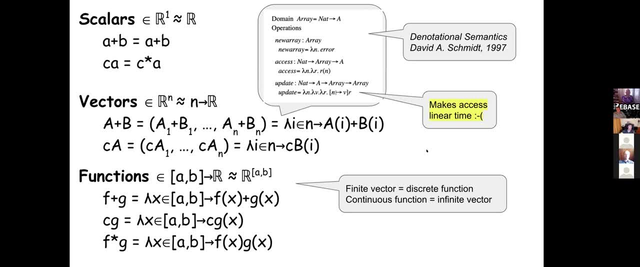 but in denotational semantics the way people model arrays is by functions, from integer indexes to values, And well, and then you can define the addition of two arrays as the addition of two functions. right, So here you see, I get a new function. 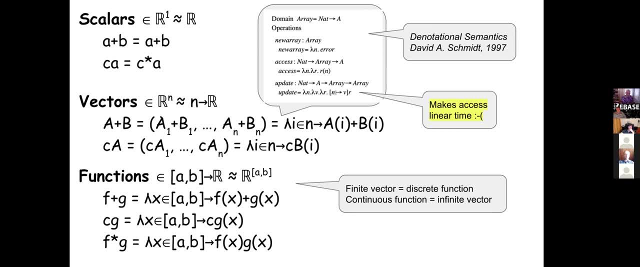 Instead of saying: this is an array where each the element is the sum of the corresponding elements from the previous array, Here you get the function same with multiplication. And then here you see if I generalized from functions that take real numbers and the interval between A and B. 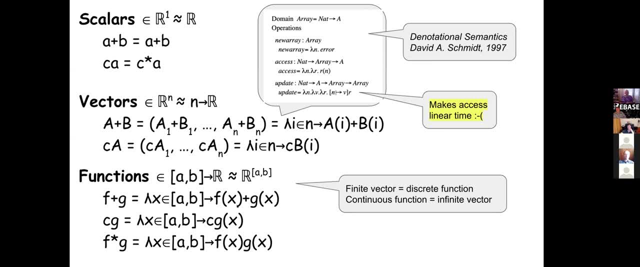 and the definition of addition of two functions becomes exactly the same as the definition of the addition of two arrays. So suddenly there's no difference. Yeah, One second. There's a question, maybe in previous slide Vinod was asking, so it sounds like you need argmax. 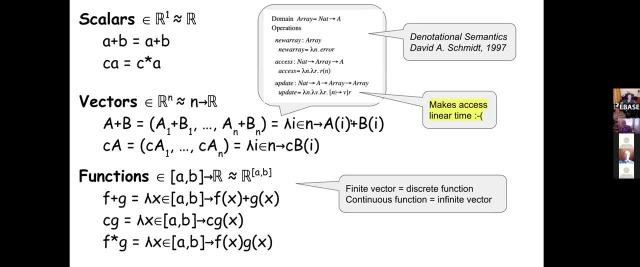 on general arguments types. Yes, that is, you can look at it that way. Yeah, because that is what gradient descent is doing. Is the solution to the last problem. a circle arc asks Alex. Yes, And that's also another interesting problem. 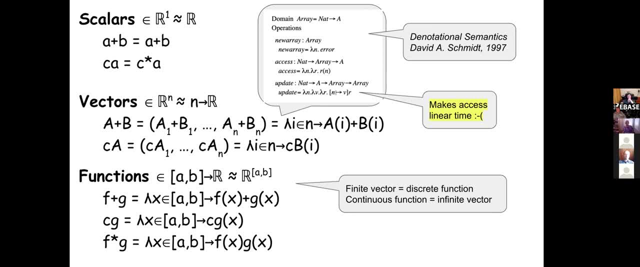 namely that a circle is not. you cannot describe a circle by a function, So we have to also generalize from functions to something else. Yeah, Yeah, Yeah, Which is also something we'll talk about in the end. So that's a good question. 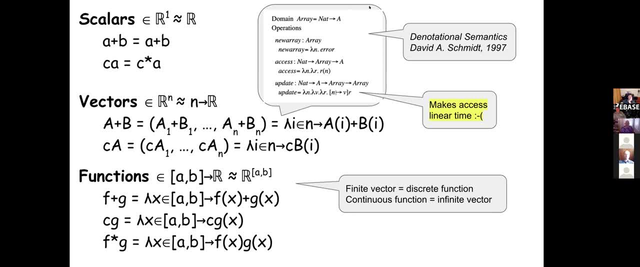 Let me see if I can show the chat here. Don't worry, I will read them to you, because it's very disturbing to have to monitor it. OK, if you read them to me, then it's fine All right. So here's another. 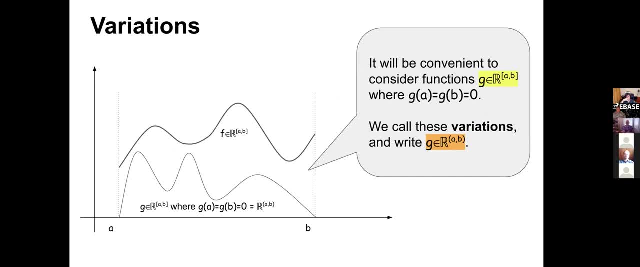 Just a quick matter of notation, and we'll also be looking at functions- partial functions, in the interval between a and b, where they are 0 at the start and the end of the interval. So here you see a picture. Here's a partial function defined in the interval. 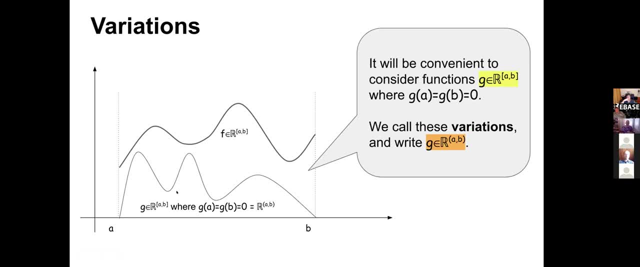 between a and b, that's f. And then we are looking also at functions, partial functions, that are like 0 at the endpoints. that will really be abusing notation here. But we call these variations and we'll write them with round brackets here. 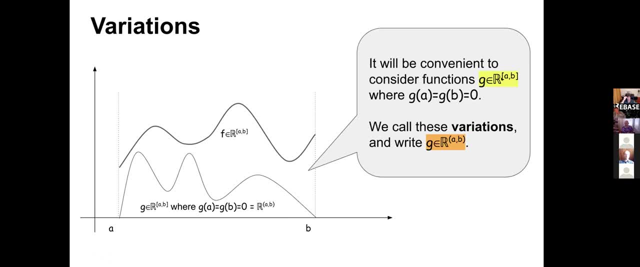 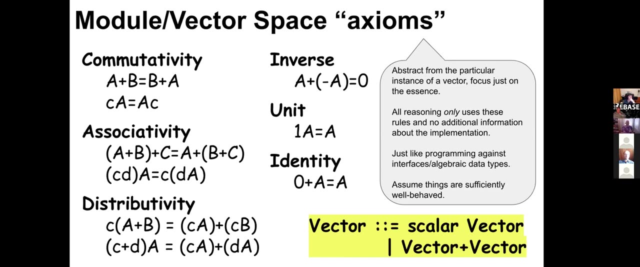 So partial functions will be written with square brackets, And then these variations. we'll write them with round brackets, round parentheses, And I'll call that out later. All right, so now that we've seen scalars, vectors and functions, let's now abstract. 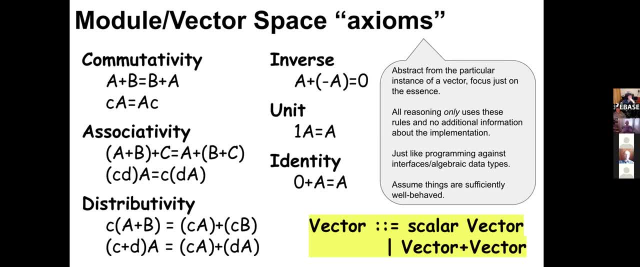 from these particulars and just define the operations that we want to have on that. So we're going to define. we've seen several implementations. That's great. Now let's assume what are the operations that we want on them, And those are the only thing that we'll use in reasoning. 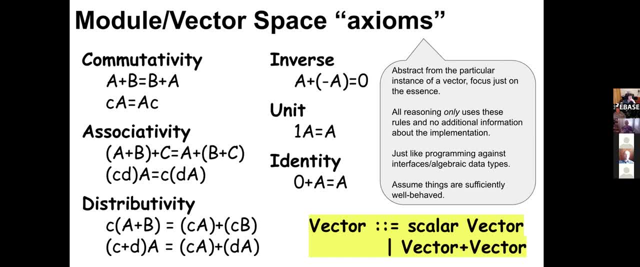 And we'll not try to use anything about the implementation. It's just like programming against an interface or an algebraic data types And then, as I said, we'll be sloppy, but we'll assume that these are sufficiently well-behaved. 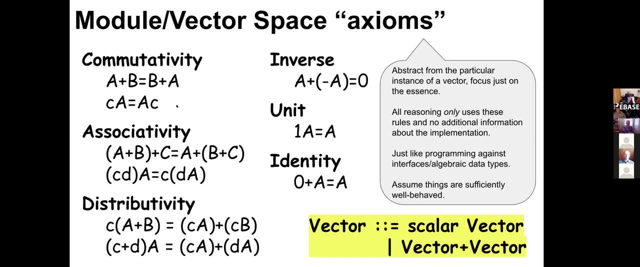 So what we assume is that addition is commutative, that multiplication is commutative, that it's associative Distributive, that there's a negation, There's a unit element- 1 times a equals a- And there's an identity for addition: 0 plus a equals a. 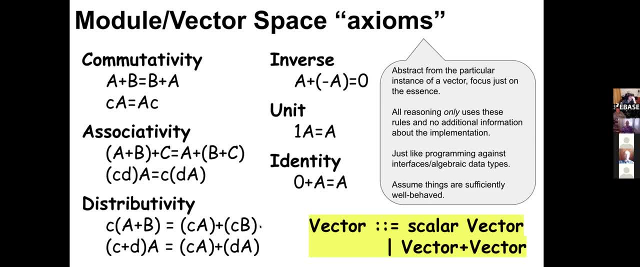 Good, Now, if you look at all these expressions here, we can write a little grammar for vectors, And you see it here Like: a vector is either the sum of two vectors or the addition of two vectors, And all the expressions here follow this grammar, right? 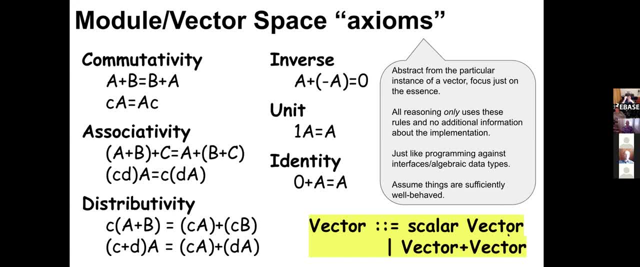 So that's kind of like you know. so this is again like if we look at how expressions that construct vectors look like they're either scalar times vector or vector plus vector, And then of course there should be some vector literals. 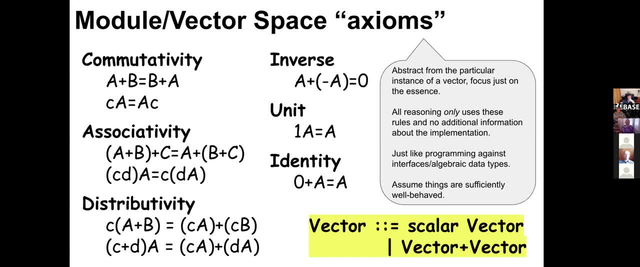 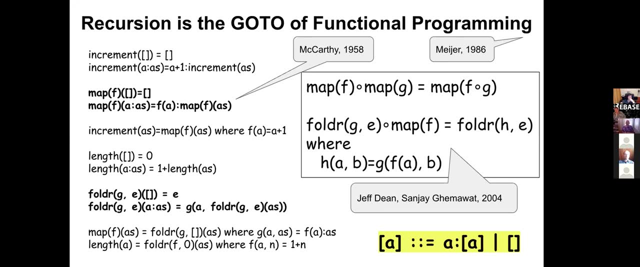 But for now we'll just assume that there's some kind of variable that contains a vector, So there should be maybe here an extra field here, But we'll just ignore that for now. All right, And now let's look At a similar thing here, where we have lists. 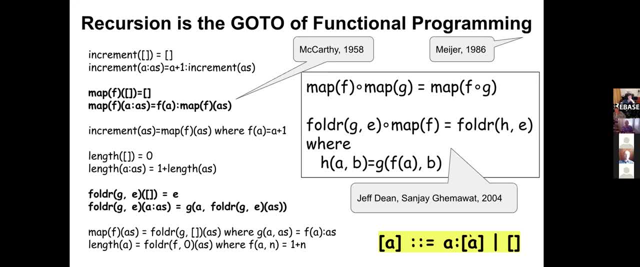 So if you look at lists- and here I'll use Haskell notation- So a list is either an element concatenated onto a list or the empty list, And now we can define all kind of functions over lists, And so we can define a function that increments every element. 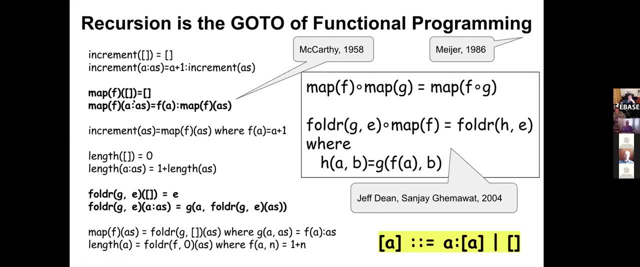 But that function can be defined as a map, And so any function that applies a value to every element of the list can be defined as a map. But there's an even more general function: to work on lists, And that's fault or fault write. 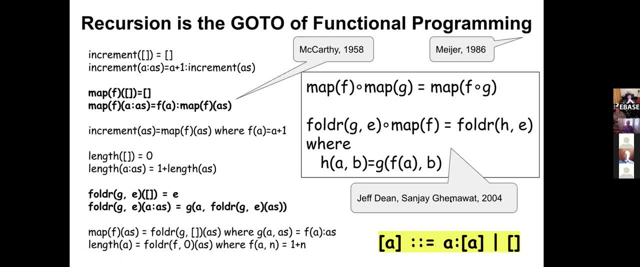 And again this tongue-in-cheek- this is kind of like MapReduce, But of course the functional programming community has known this forever- that you can write functions over lists using faults. Now, what is so special about faults? Well, faults are home and work. 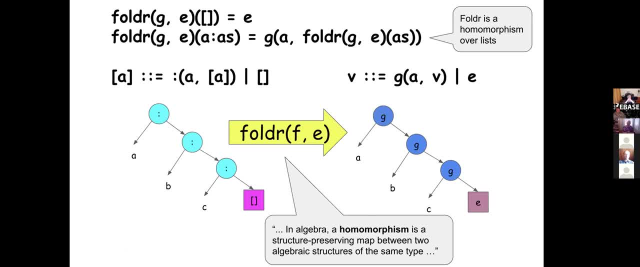 Yeah, Yeah, Yeah. So you have to have a structure like a path, that is like a very, very simple structure, And you have to have a structure that has very simple map, And so the structure is like a map, just like any other structure. 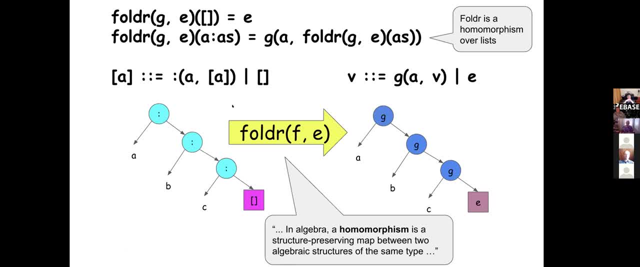 So if you look at記-bira, the oldest homeomorphism is the structure preserving map between two algebraic structures of the same type, And that's all sounds very impressive And it's easiest to just look at the picture here. And what does a fault do? 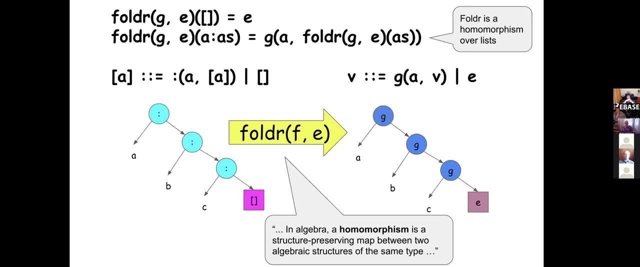 So here's the list. So it's like A comes B come C comes empty list. the value e and really the, the structure that you get here is exactly the same as this structure, right, and so a value here looks as like you know, e, or the function g applied to a and v. 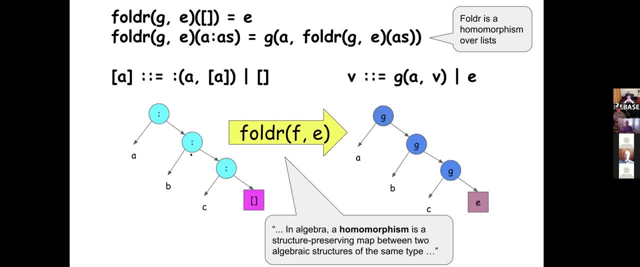 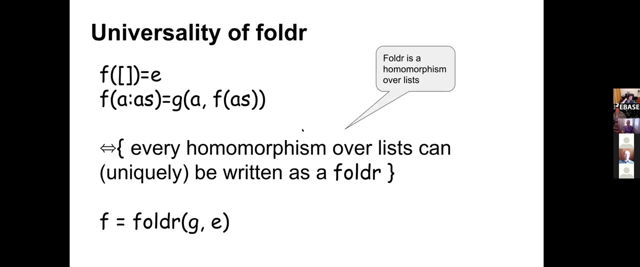 and so, literally, like you know, a fault just replaces, like in this kind of linearly nested structure, by another linear and nested structure, and, and these faults or these homomorphisms, have all kind of nice properties, um, and one in particular is that any homomorphism over lists 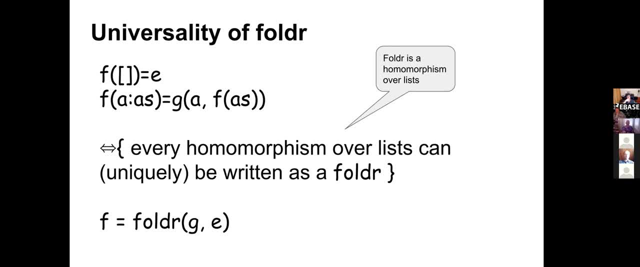 can be written as a fault? um and uniquely be written as a fault. the graham hutton has a nice paper about it. it's called the universe on the universe: universality of fault r? um. but it's kind of kind of beautiful right. it's like you know, you, it doesn't matter what function you write over. 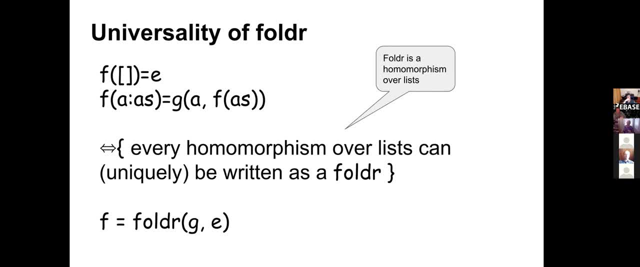 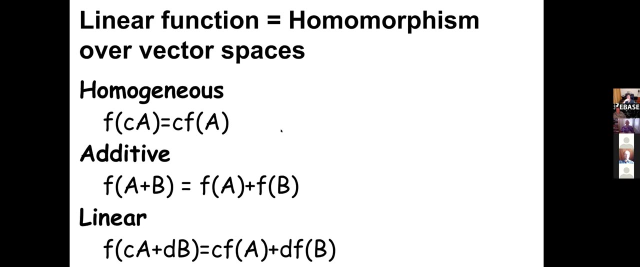 list. if that function happens to be a homomorphism, you can uniquely write it as a fault r, um, and this is, i think it's truly beautiful. um and now um. let's look at here: um. we've seen that these um vector spaces also had a similar structure, so 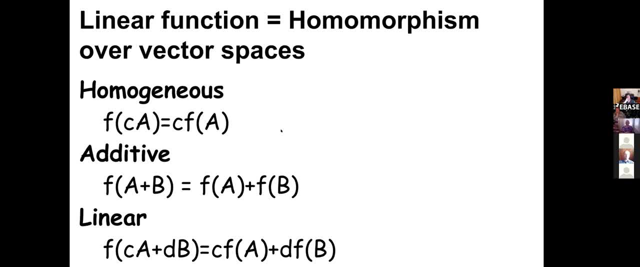 let's look at homomorphisms over vector spaces. mathematicians happen to call those linear functions, but what are they? well, they have to, um, um, preserve the structure. so if i apply a homomorphism over vector space on a scalar multiplied by a vector, that should be a scalar multiplied by a function applied to. 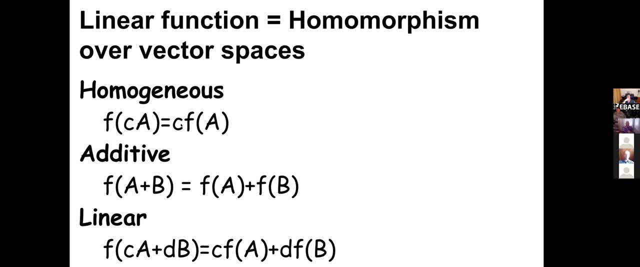 the function applied to the vector and notice that here there's implicit multiplication that's overloaded and here's multiplication that's overloaded, and these multiplications can be of different types, right, because f maps like one vector space to another vector space, so there's a lot of implicit overloading going on here, and then it has to distribute over addition. 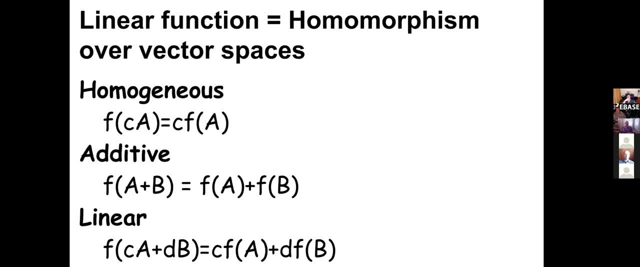 and again, this addition here is of a completely different type than this, because this one is over the source vector space and this is over the target vector space. um, but i'm going to get, like you know, not be a like typoholic today, so i'm just pointing it out here. you can take these two. 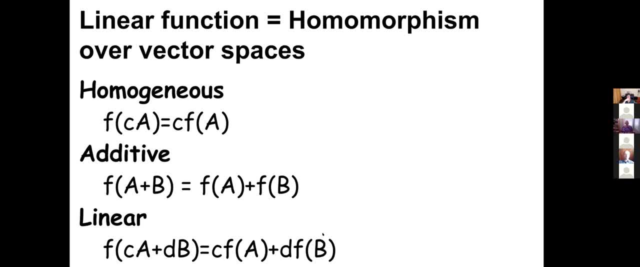 rules together and then you can write it, like you know, in one go like this: so a linear function is actually just a homomorphism over vector spaces. now what we saw for lists- that every homomorphism over lists could be uniquely defined using a fault r. so now the question is: is there something like 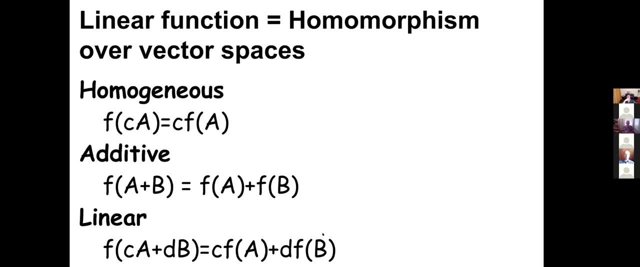 that a universality property also for linear functions or for homomorphisms over vector spaces, and that would be great, right, like you know, because then something that we know for lists and we know for um vector spaces as well and in some sense um the vectors look very much like lists, right like this is like list concatenation and this is like 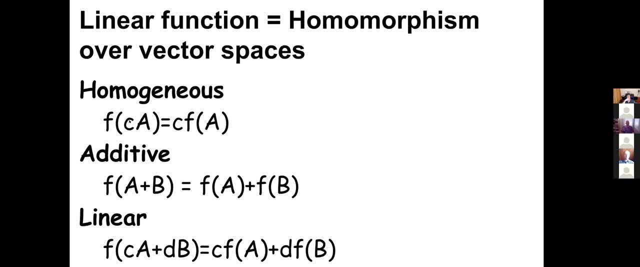 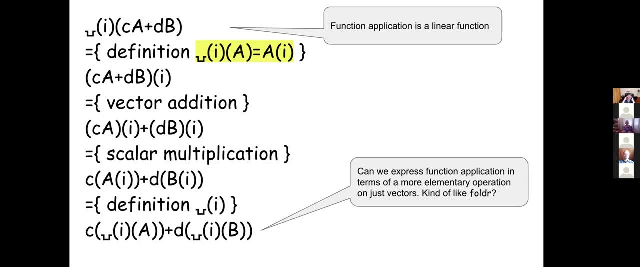 you know something like a map over list, so it's kind of like you know you would expect something like that to happen, um, but let's look at like an example of a: um, a linear function first, and this one is kind of like- maybe a little bit surprising- function application is actually a linear function. 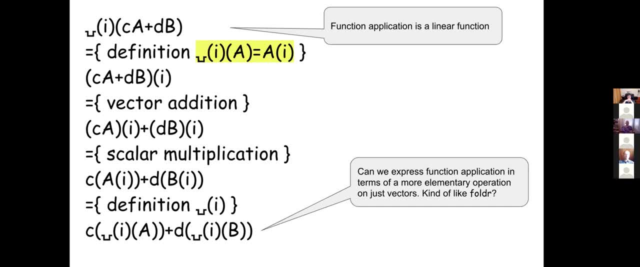 um, and so here we define function application and there's a hole here. so the hole applied to i applies to an array is the array applied to i. so this is really function application. um, it's a, it's a higher order function, right, because it takes a function. this is an array. 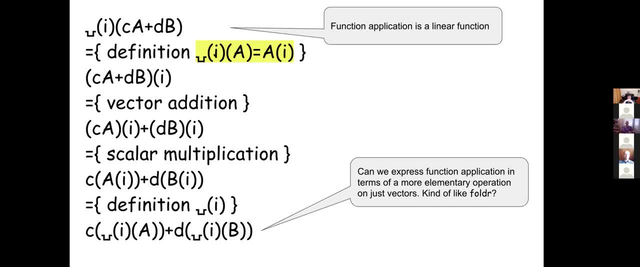 an array is a function from integers to values and it applies that function to a parameter. so so this is really a higher order function, um. and if you look at this um derivation here, you see that that application distributes over addition and multiplication. so function application as a higher order function is a linear function. um, and now the question is: 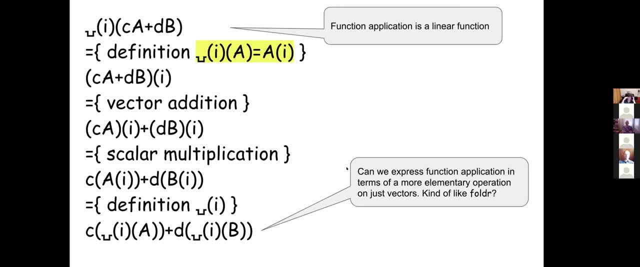 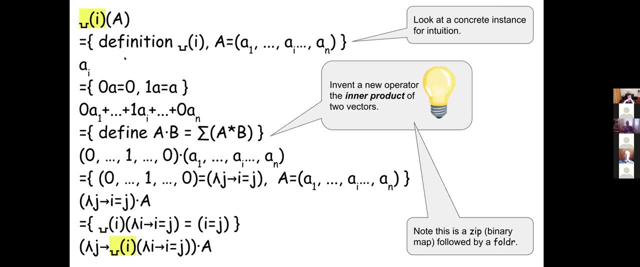 can we express this thing um in terms of more elementary operations, just like we did with fold, R, um, and in order to do that um, we're we're going to go and kind of like you know, use our intuition pump. so we're looking at a concrete um array here just for fun. and so if we select the id element of 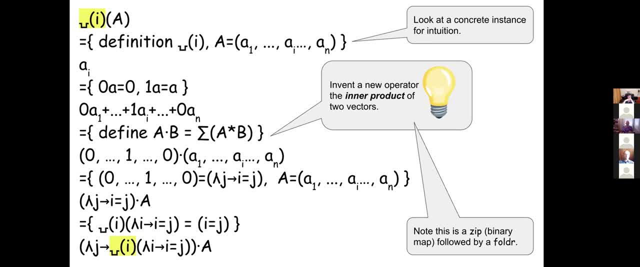 the array, we get a i. now we know that zero times a is zero and one times a equals a. so a i is just the same as zero times a one, but every zero except for a i, um, and what we see here is really: it's a zip, right, a zip. 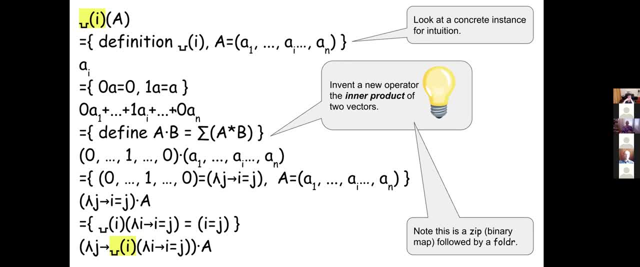 a zip width of multiplication followed by a summation, um. so we know how to do that. so let's just define this new operator which multiplies two arrays and zumps them up. so this is zip width, and then we do a sum and now this becomes- like you know this expression here. 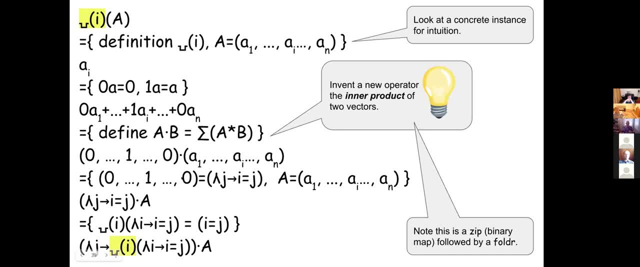 this array that has like a one at position i, we can represent it by this function here, so we can write um function application like this. and now we see that here- really here- there's function application hidden in here, so we can just do that here, and now we see that we can write function. 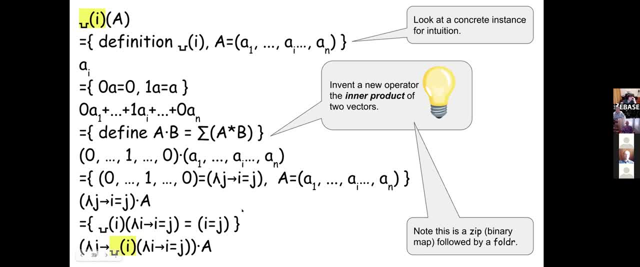 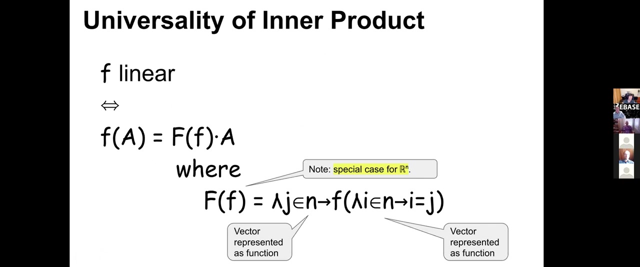 application as a um dot product of the argument and some expression that involves the original function, um, and again this is, like you know, very similar to um defining a function, the homomorphism over lists using full bar um, and this is the universal universality of inner product, if f is a linear function over any vector space. 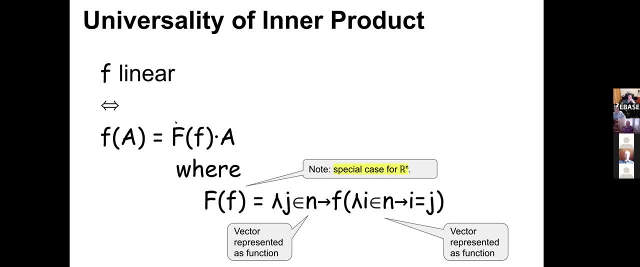 we can uniquely write it as the inner product of of two vectors, which is two functions. and so think of this really, as, like you know, the same thing as any homomorphism over list can be defined as a full bar, any homomorphism over vector spaces can be written uniquely, will be written as an inner product. and eric yep um alex. 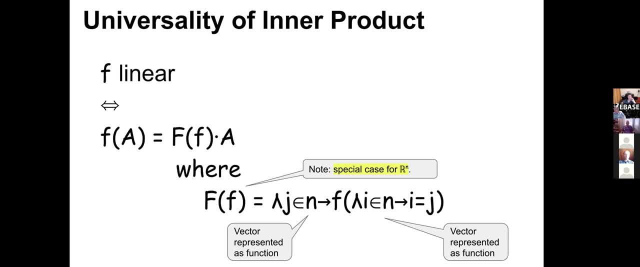 is asking: i equals, j is one. is i equal j and zero? otherwise, uh oh, it's equal and equal, equal. yeah, so i'm actually asking, like in this list, like a shorthand function that you had in the previous slide: so i equals, j is sort of an. 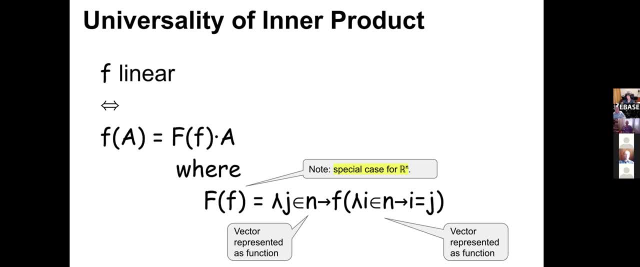 expression here that values to one when left and the right side are equal and to zero otherwise. so, yeah, so i'm also kind of, like you know, like, um, uh, yeah, i'm. i'm implicitly converting from, like you know, zero and one to the booleans: um, okay, well, or javascript style, or php style, whatever. 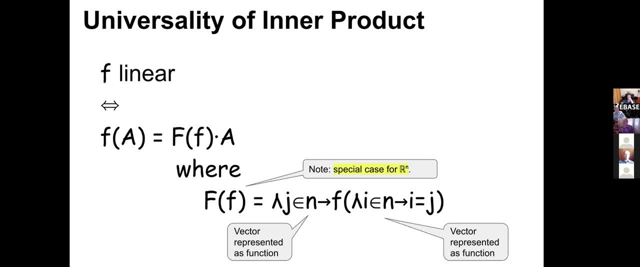 today to honor young. i'm not going to be like a type of hollywood, i'm going to be like a type of: I'm going to embrace dynamic typing. Okay, Also, I'll be switching implicitly from arrays to functions, right? So I'm not going to write a cast that, if there's an array, 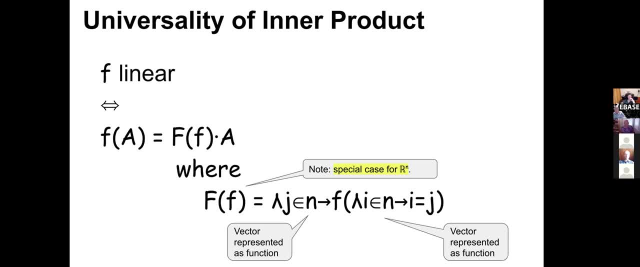 I'm going to just kind of jumble them up. So here this really is a vector represented as a function, And then this is equality, where this is like either zero or one. So this is an array of zero and ones that has a one on the i-th position. 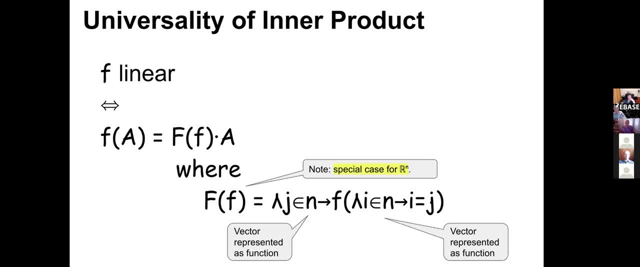 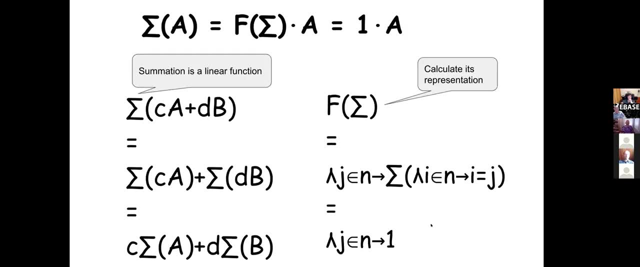 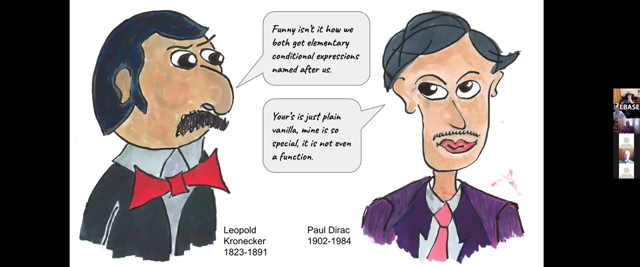 or on the j-th position, And Matt says: so it's just the Kronecker delta. Ah good, That's two slides here. It's exactly the Kronecker delta, Yep, And which is kind of interesting, right. 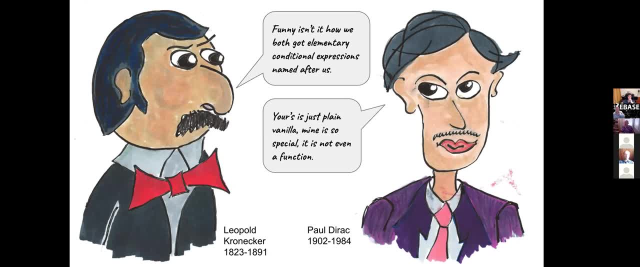 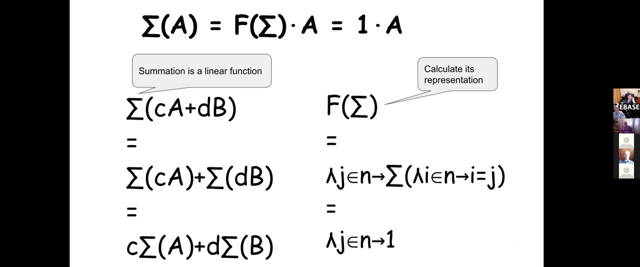 That just a simple conditional expression is named after someone. All right, So let's look at here now And we Okay, So let's look at another kind of example here. So, summation of a vector. if I sum up all the elements, 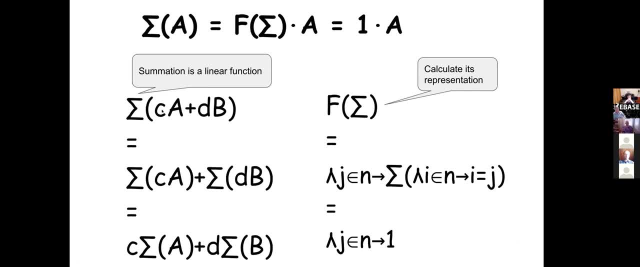 is a linear function. That's kind of not surprising, right? If I sum the sum of two vectors, then this sum distributes over sum And then I can pull out the multiplication. So this is the Like. sum is linear. So that means that sum can be written as a composition of the argument of A. 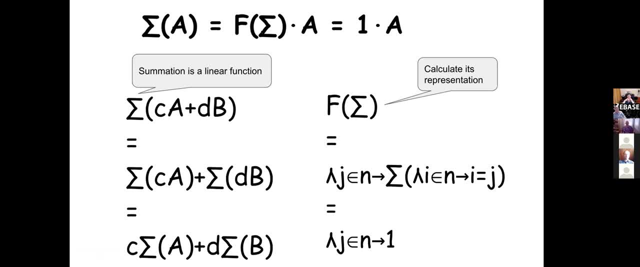 and the inner product of sum. And then I can pull out the expression of summation. In this case I can calculate the representation just plugging it in the previous formula. That turns out to be the function. that's always one. So to sum the elements of an array: 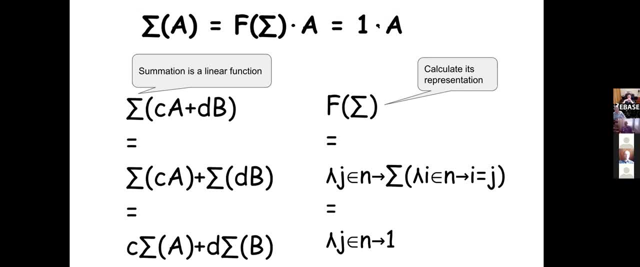 I just take the inner product with the constant function one, And then later we'll see that if I want to take the integral of a function, I just take the inner product with one. So there you see what's first required: intuition suddenly becomes just. 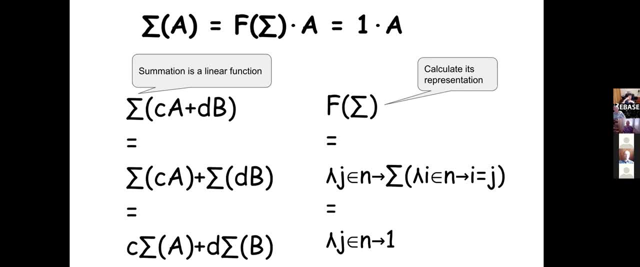 equational function. So that's the idea of equational reasoning, right, Because integration is also a linear function And it's just like the inner product with one. So that's kind of like you know, suddenly unifies these concepts. 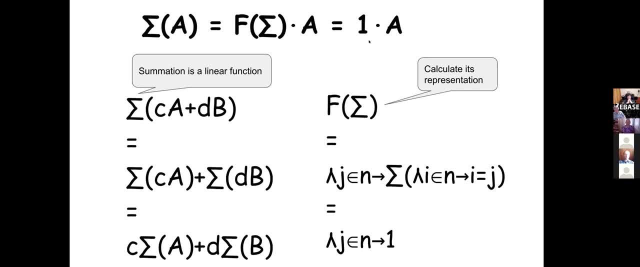 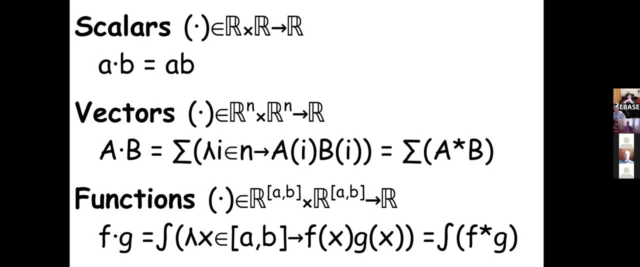 And because you focused on what is similar instead of what's different. So let's look at the various implementations of inner products before we abstract from them again. So for scalars, it's just multiplication. For vectors, we've seen that already. 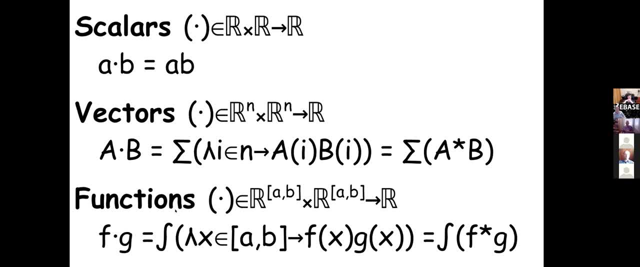 We just zip the two vectors and then sum them And then for functions it turns to be you multiply the functions and then you take the integral And the way I do integrals here. often you see integral from A to B And I use the same convention here that if this is a function, 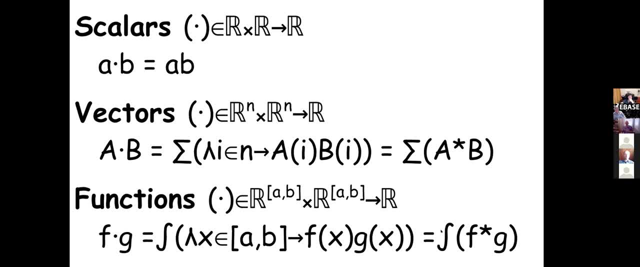 that is a partial function from A to B. the integral kind of, like you know, integrates over the range and the domain of the function, Sorry, And so I won't write the A and B here. I can see that from the type. 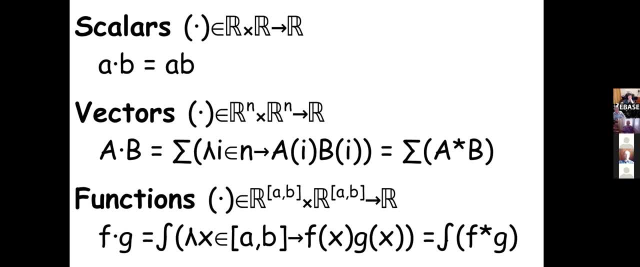 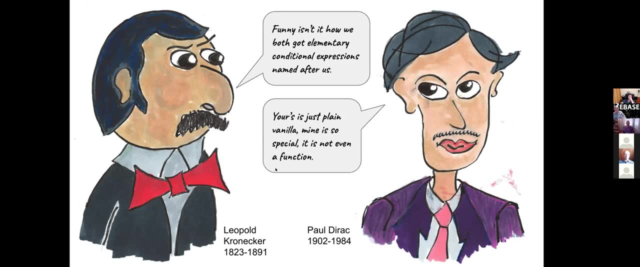 And this is a partial function from A to B, So the integral goes from A to B And that makes the notation like much shorter. I don't have to get like carry around the bounds, But as to who was it that asked, Yes, this is definitely like just Kronecker delta. 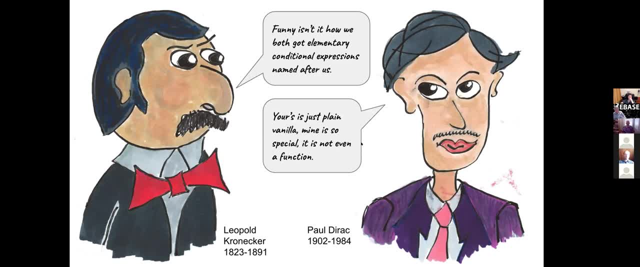 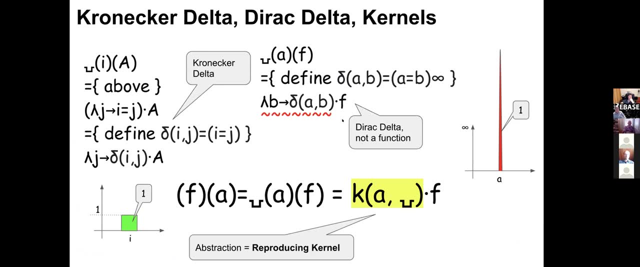 And then for integrals we need something similar, which is the Dirac delta, And the Dirac delta is a little bit of a difference here. It's the only time I will do some type checking And if you look at, like Kronecker delta. 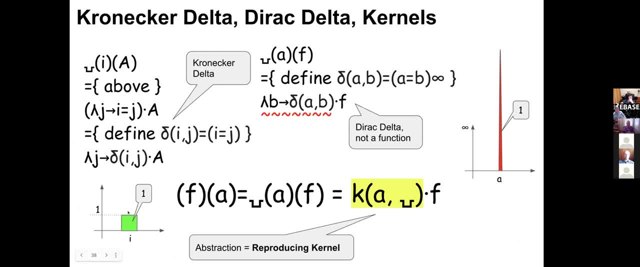 that's something that's got like zero everywhere, except at position I it's one, And here we see that the area, the surface here is one. So for the continuous case we need something similar that is got like, you know, zero everywhere. 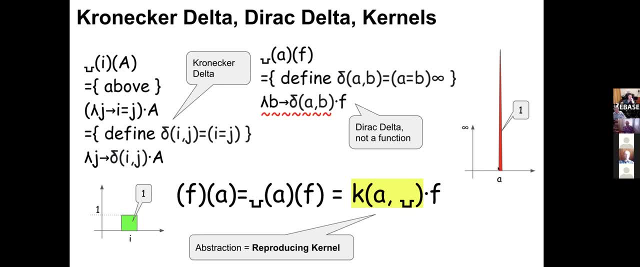 except at here I use A and B instead of I and J, And it should be something that's got like you know has a surface area of one Where it's got like you know, only got like you know at A. 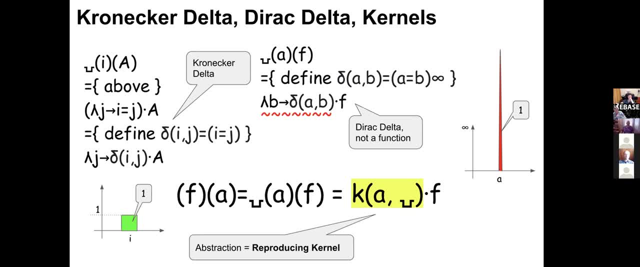 And that's not a function And that's people call it the distribution. So it's not a function And I defined in our product to be to work on two functions. So this doesn't type check because the Dirac delta is not a function. 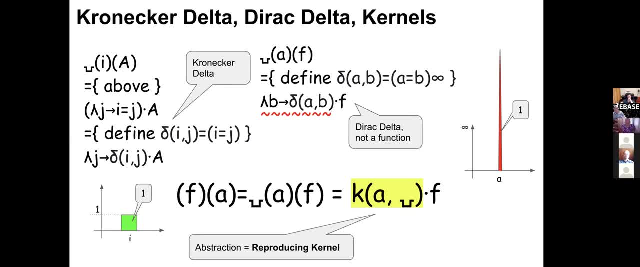 A lot of. I think physicists don't care and computer scientists do care. So what we'll do is we'll, kind of like, acknowledge our sloppiness And we'll just say like, look, we have a special function here, which is- let's read this one: 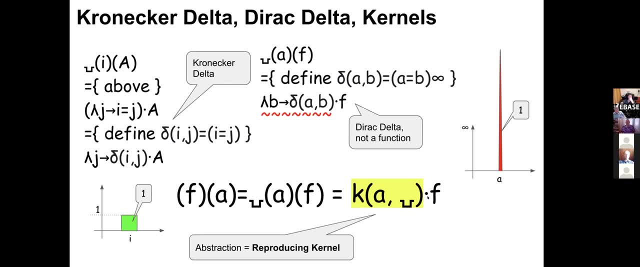 But that's the representation of application. that is a function And we won't go into this here. And was there a question A few seconds ago? David asked: why is it not a function? And I'm not sure which part he was referring to. 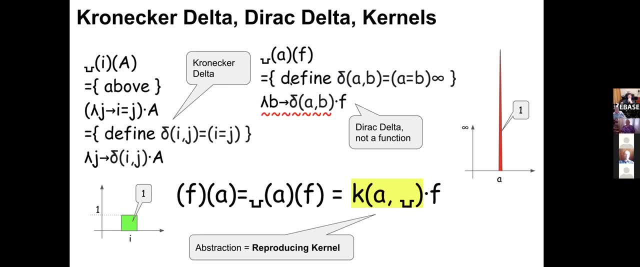 OK, the Dirac delta is not a function, And the reason is that this thing is kind of like it is something here that has a value of whatever infinity at A, But the integral is kind of like 1. So that's kind of like. that's a weird thing. 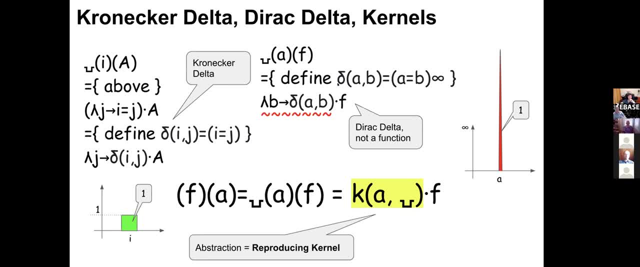 That's kind of like it's not a function And you define it kind of like by saying that it satisfies this property. So basically, what we're doing is we're saying like we assume that there's a function that satisfies this thing. 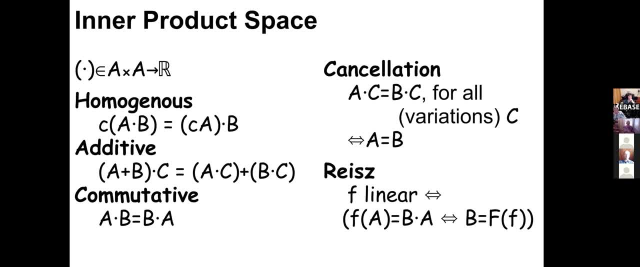 All right. so now that we've seen several implementations, let's abstract again, just like we did with vector. So now we have an inner product space, And here are the properties. We want scalars to distribute over inner products. We want inner products to distribute over addition. 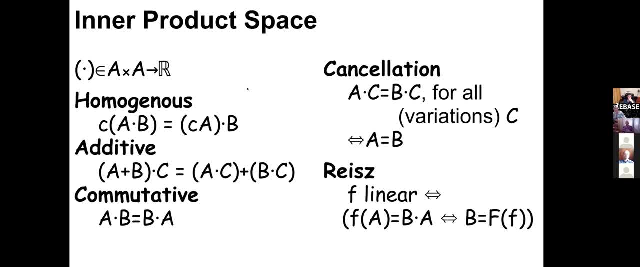 And we want them to be commutative. And then here, so this has got, like you know, in some sense also some linearity property here. And then there's two other rules that we're going to use, And one is the cancellation rule, because often we 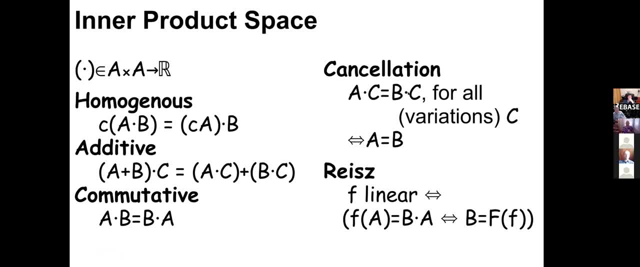 have expressions A- inner product C equals B inner product C, And then we want to: well, if A equals B, then of course A times A inner product C is B inner product C. But we also want to use it in the other direction. 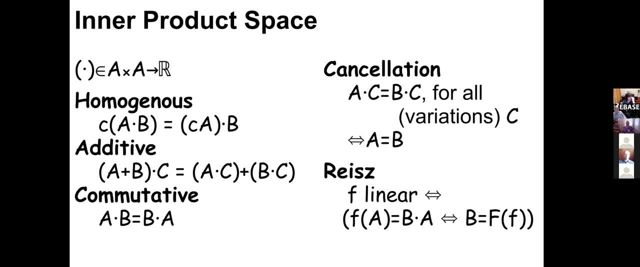 OK, OK, OK. And we've seen this rule like in one of the first slides for multiplications, So we'll assume that this holds, for if A inner product C equals B inner product C for all possible C's- And these C's can be also variations- then A equals B. 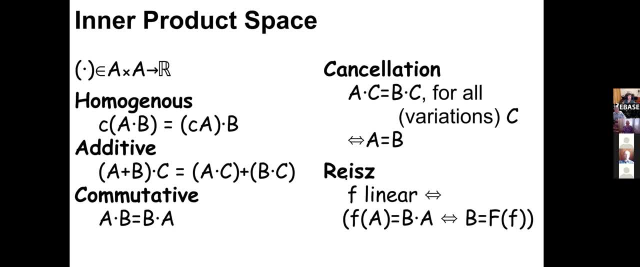 And then the other one, and this is the folder rule. So this is called the Riesz representation theorem. It says that if F is a linear function, we can write it as an inner product. all right, So if F is linear, it can be uniquely written. 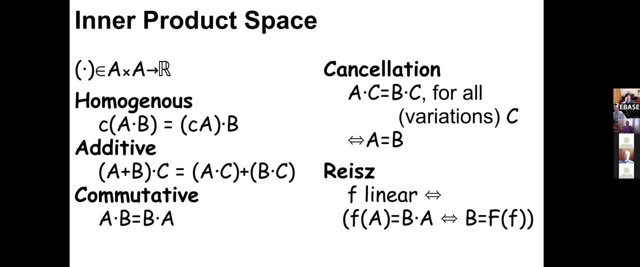 as B inner product A, where B is, like you know, there's some function F that takes the linear function and turns that into a vector, And you can look at your favorite linear algebra book and find, like you know, a proof for this. 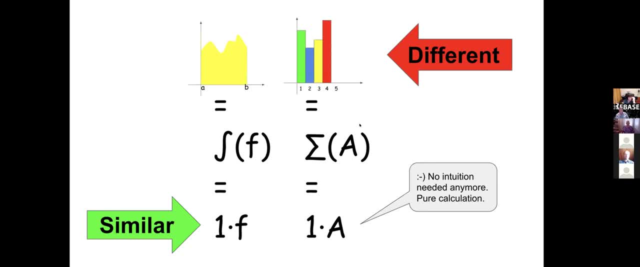 All right. so now we like the thing that we needed. intuition for becomes, like you know, just the same thing. right, Like the integral here is just 1 inner product F and the summation here is 1 inner product F. 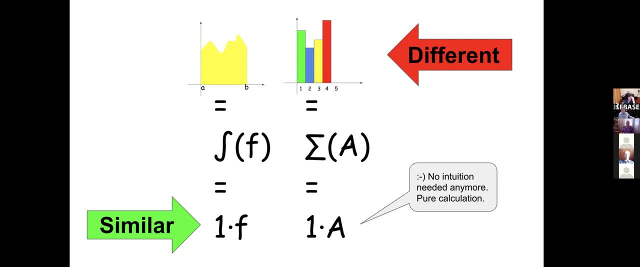 And I think this is really beautiful because suddenly, something where I need to draw pictures and, like, have some intuition about areas, surface areas. I don't want to do that. I don't want to look at pictures, I just want to look at expressions. 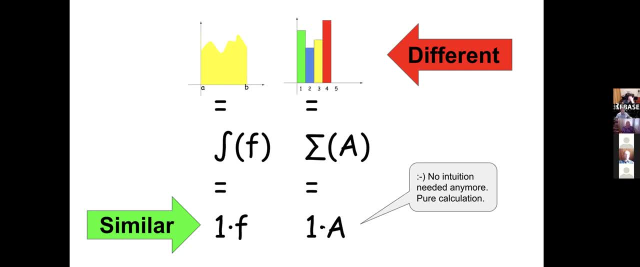 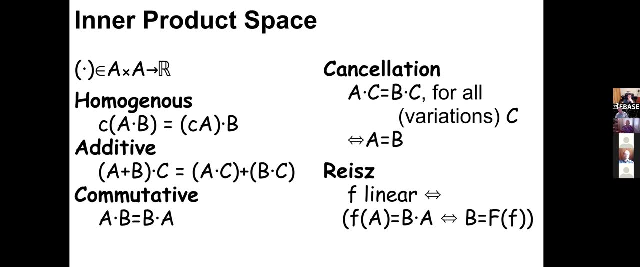 that I can manipulate, And here I have expressions in terms of inner products, and I know the laws that hold for them, for inner products, so I can manipulate them without any intuition. That's exactly what I want, All right. so here is the rule. 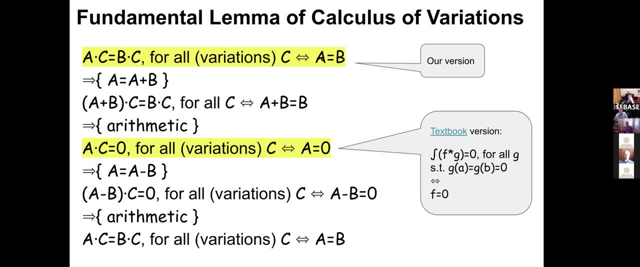 That we use the cancellation rule. If you look at this calculus of variations, they have something they call the fundamental lemma of the calculus of variations, which is slightly different, which says that if the inner product of A and C is 0 for all C, that's if, and only if, A equals 0.. 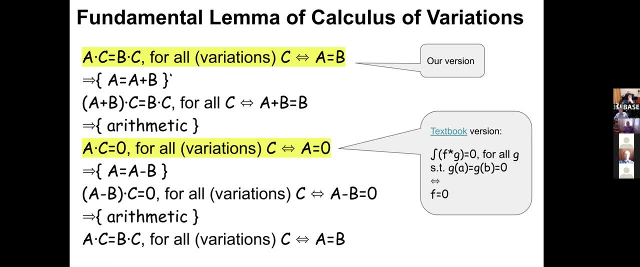 And this proof here shows that this is the same thing. It's just. here is the circular implementation. I like this version much better because I think it looks much nicer. This is the same thing And this even though they're equivalent. 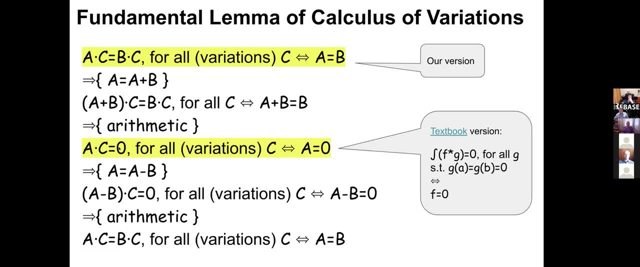 this one feels way more special because it only looks at when the inner product is 0, where here this feels more general? But again, it's not more general because they are equivalent. All right, good, Now the next thing we have to do. 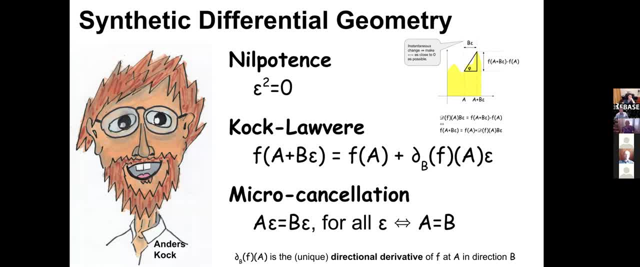 and now we know all about inner products. and this was your linear algebra course from university in 10 slides, And now we have to get your calculus up to speed, And one of the things that I said is we want to make the change here as small as possible. 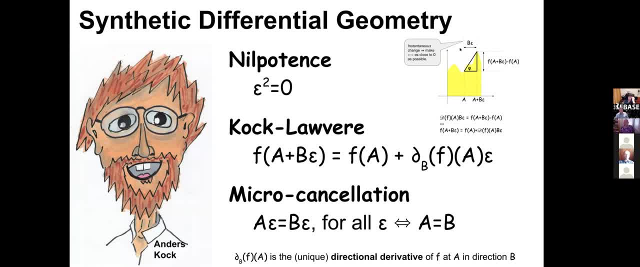 And Mr Gauchy wants us to do that by limits and epsilon, delta and whatever. But there's a much better way, I think, and also that appeals much more to my computer science heart. here is what does mean something. 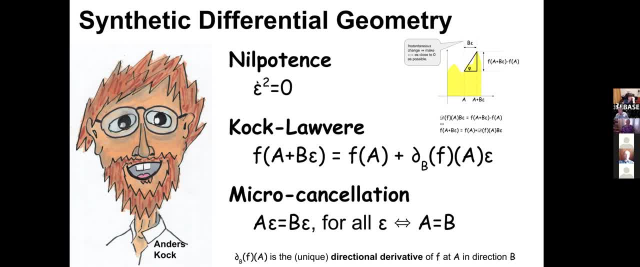 as close as possible to 0? Well, if we square this value, it becomes 0.. Well, if epsilon is so small that when you square it becomes 0, that makes me think that's not good. It's something that's as close to 0 as possible. 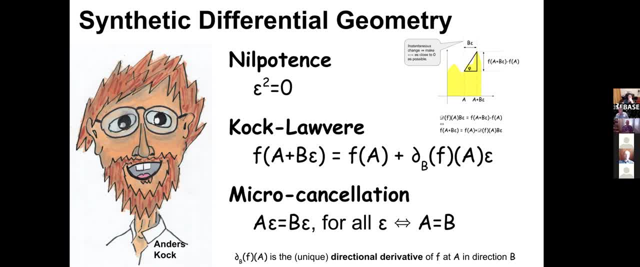 And so we're introducing this nilpotence and nilpotent values. epsilon squared equals 0.. And then remember that we defined derivatives here, like via the tangent, We're going to just take that as our definition of derivatives. But we're generalizing a little bit. 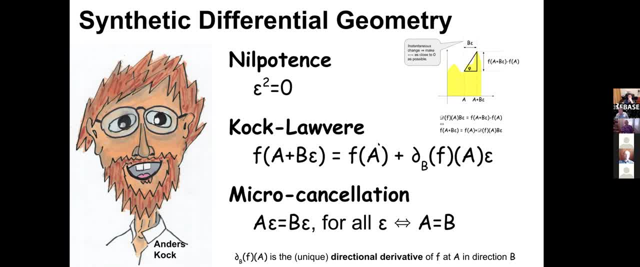 because here we only had scalars And now we need to generalize the derivatives over vectors, And this is called. It's called the directional derivative, And this value is also unique. So uniqueness is important here as well. So we just define like we look at this picture. 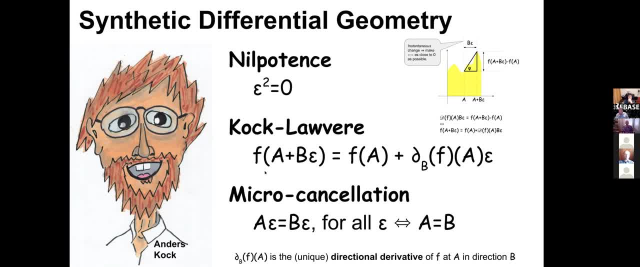 and we say, OK, let's abstract from that to any vector, And we define derivatives like that And we looked at this thing. What does it mean to be as close as possible to 0?? Well, we'll say that means that epsilon squared equals 0.. 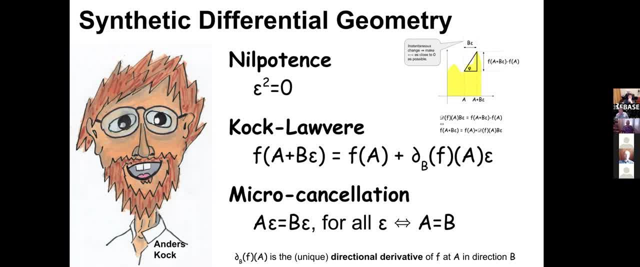 And from this it follows another cancellation rule that if A epsilon equals B- epsilon for all epsilon- then A equals B. So that's it. So that's another cancellation rule which kind of follows from the uniqueness here, But we'll mention it here. 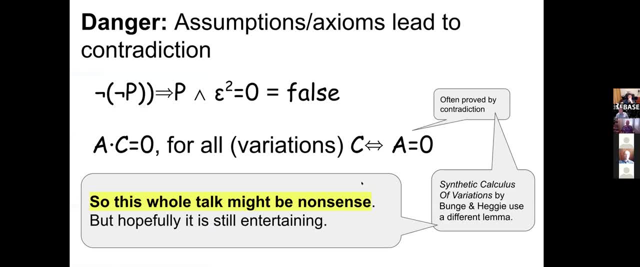 So this is all the calculus that we need. Now, there's a little bit of danger here- is that if we're taking epsilon, squared equals 0, then in conjunction with- oh, there's a missing parent here- in conjunction with the law of excluded middle, 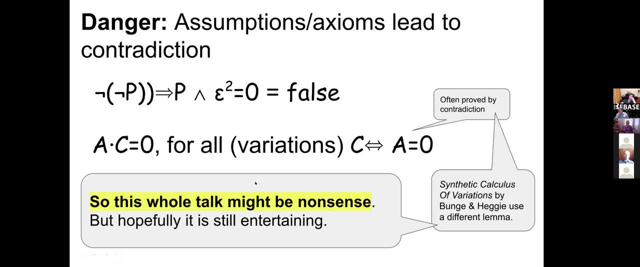 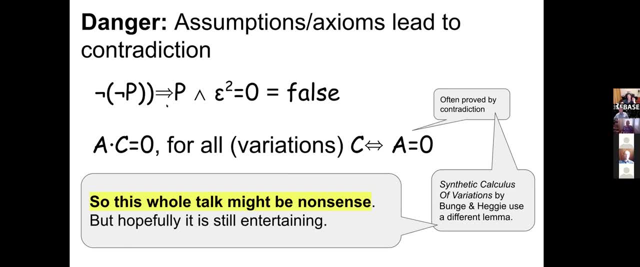 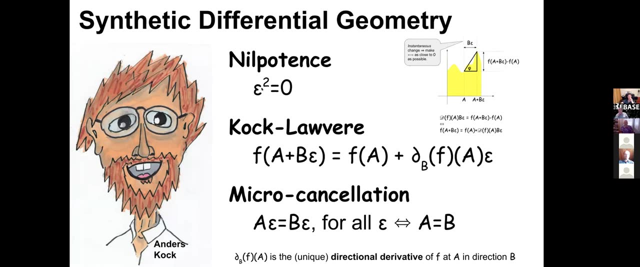 that like an excluded middle. Eric. what is the domain of epsilon? Sorry, What is the domain of epsilon? Ah, So what we do is we, we extend the real numbers with, with this, these nil potent values, and because, like 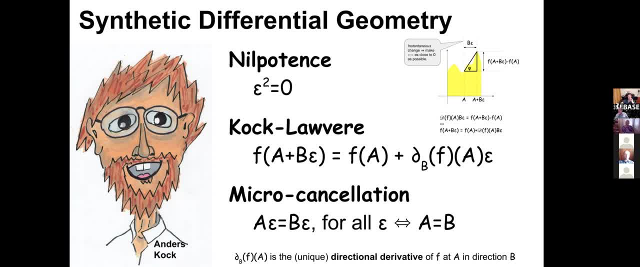 you know, real numbers are also just some some abstract data type that have certain properties. So we're we're free to, like you know, own cap, like. so this is like our real numbers have these epsilon and are no potent infinite decimals. 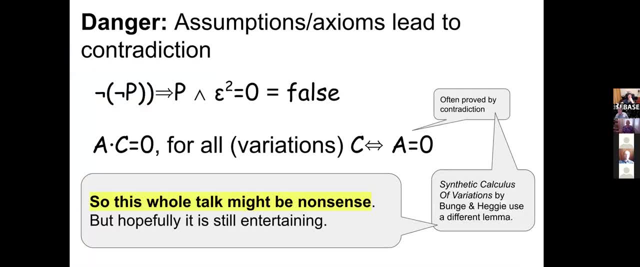 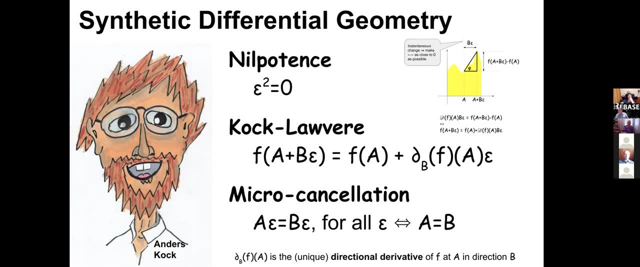 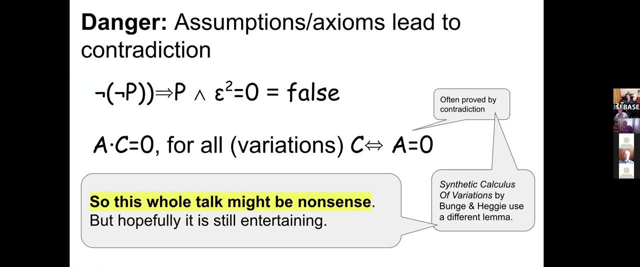 and we will just write them as real numbers, but they're just slightly different. so instead of, like you know, and the real numbers you know from your calculus class, these are the real numbers from um the cock lover, the real numbers, and it's a number smaller than any real number, but greater. 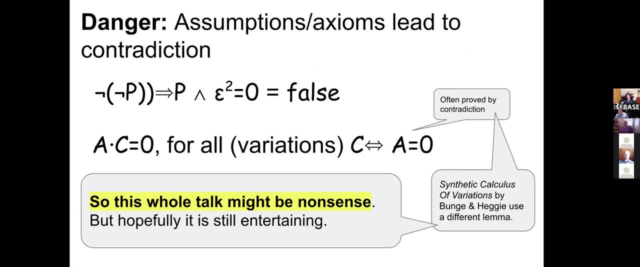 than zero. yes, that is the intuition, but because the the, because of, like you know, this, um uh, you can get contradictions. so you cannot prove that they are kept, like you know that they're not the same as zero, you cannot prove that they are, like you know, like not zero. so this is like you know. 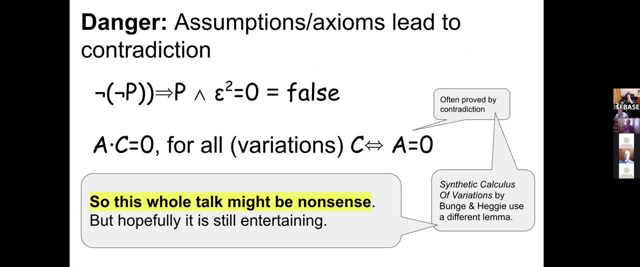 where we are here, kind of like in this, in this cat, like strange world, um, but intuitively, yes, you can see them like. there's also something called non-standard calculus, and there they define it in a slightly different way, and these are kind of numbers that are smaller than any real number but greater than zero. so think of that as your intuition. 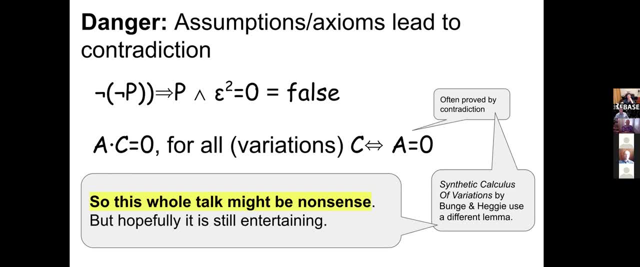 but depending on the account, like way you formulate it, and in this case you cannot use classical reasoning, as you have to be a little bit careful. and so, if this, if some other axiom, you can use classical reasoning, and so you have to be a little bit careful. um, so, if this, if some other axiom, 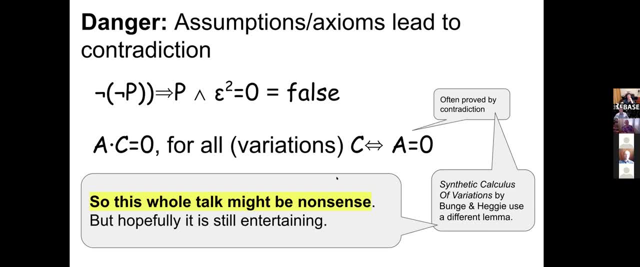 that i can't like. propose actually implies excluded middle. then everything collapses, um, which is is a possibility. i haven't proven this, um, and you, you know the story right where the phd student is doing their thesis defense and then some professor asks a question and then they go. oh, 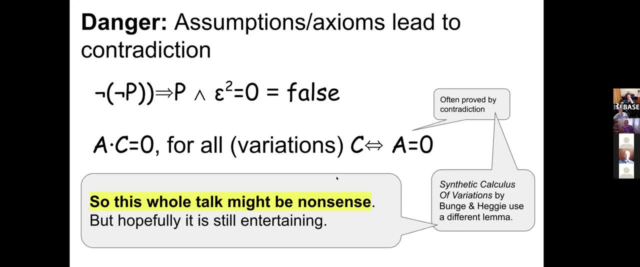 that's like: no, the only model is the empty model, and that could well be the case here, but i don't assume that is the case. but you have to be a little bit careful that once you bring in um nilportant infinitesimals like this, you cannot use classical reasoning. um, all right, so um. here's another, um. 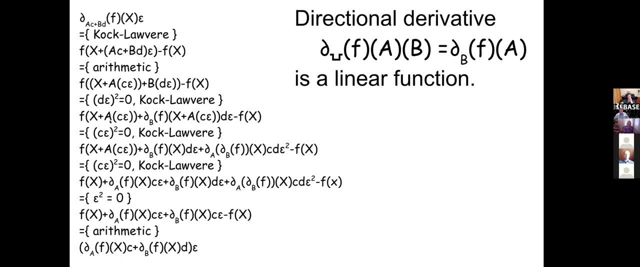 calculation. and again, just look at it, marvel at its beauty. don't try to understand it. just look at there's equals, equals, equals, equals, equals, with some simple rule here and that shows that directional derivatives are linear right. and again, like you know, i love this because i don't understand this. 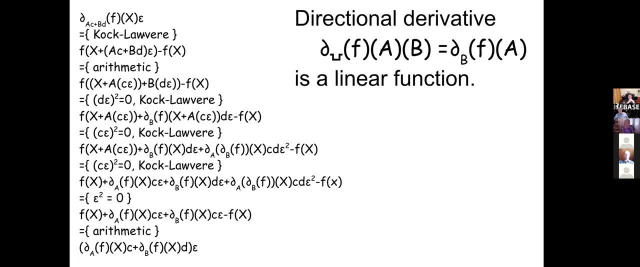 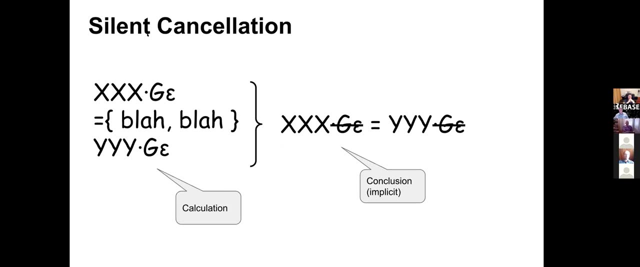 at all. i don't want to understand it. i just see that. it's simple equational reasoning. i just calculate. i love that. all intuition is gone. i don't need to think about graphs and pictures, whatever. it's now just equational reasoning, um, and this is where we use um, um cancellation, because i've used this silently. 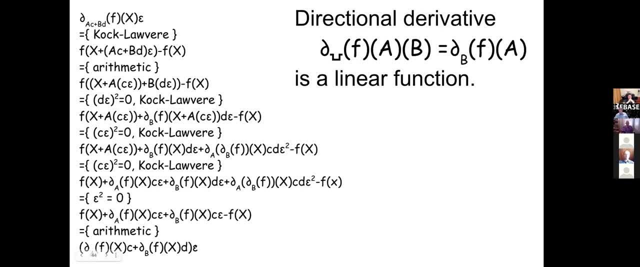 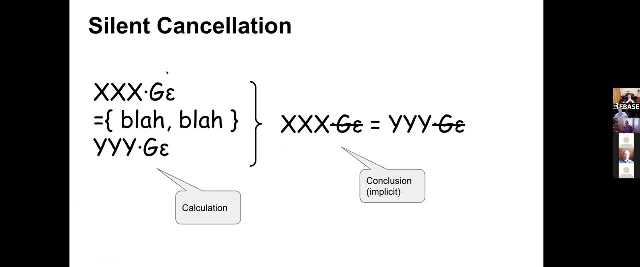 right, there's an epsilon here and epsilon here, but in order to prove that it's linear, i need to. i need to prove this without the epsilon. so that's where this cancellation rule comes in. so often i have a, an, um, a calculation that looks like this, and then i just can silently, just use my cancellation rules. 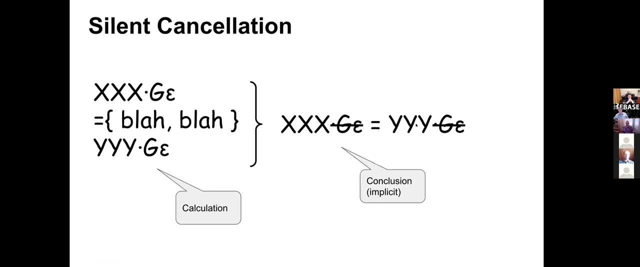 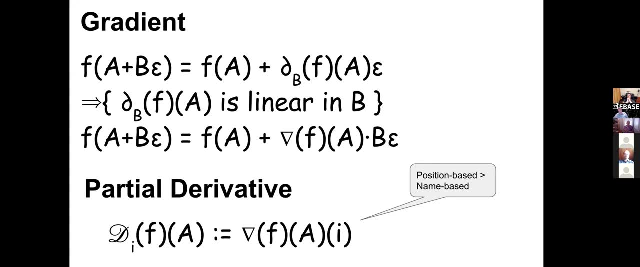 to just prove that x equals y. all right, um. now, since um, um, this directional derivative is linear, i can use the previous theorem to say like: oh, i can write this function here, which is linear in b, i I can write that as an inner product. So, because that function is linear, 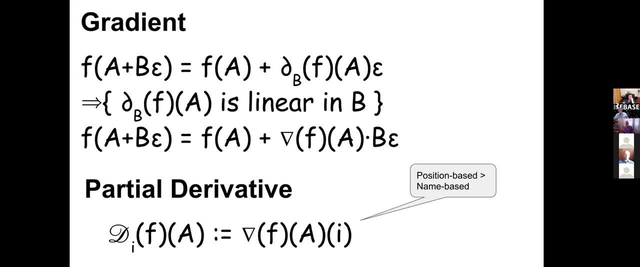 now, similarly, I can write the directional derivative in terms of this: whatever delta or nabla, whatever inner product would be, And this is called the gradient, And then I can define the partial derivative, because this is a vector. So I can define the partial derivative. 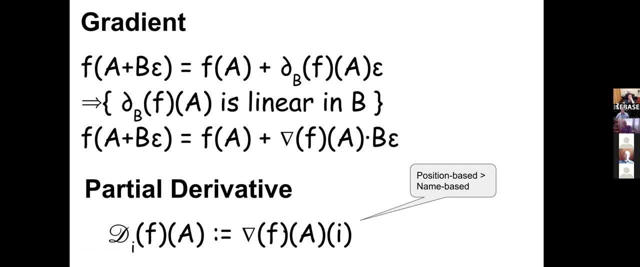 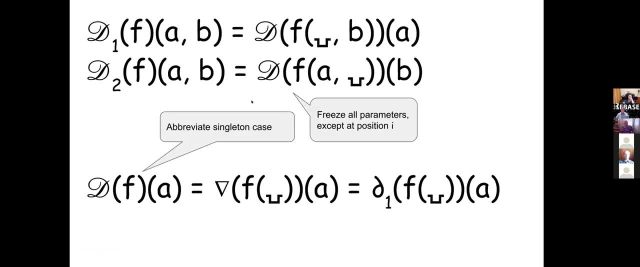 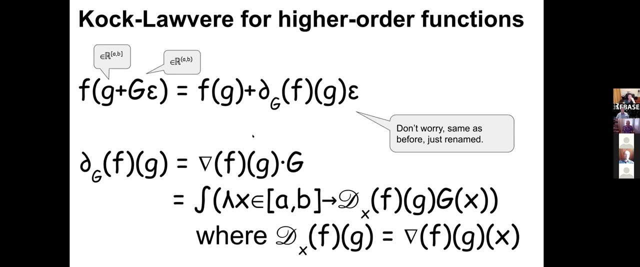 as the ith element of the gradient And notice that there's like. this is a super simple proof again. it just uses what we have seen before, Based on time. I'm going to skip this because I do want to have like a few minutes. 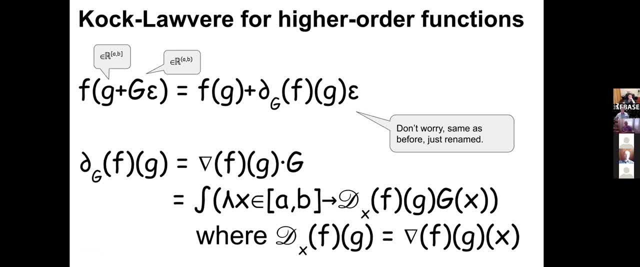 to talk about like what we are set out to do is to look at like doing this for higher order functions, So for not for NRE functions, but higher order functions. So this is the same rule here. I just renamed A and B to G and capital G. 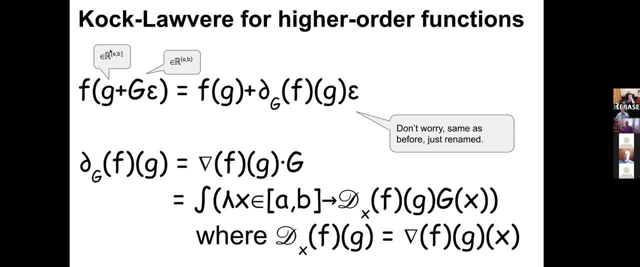 And these are now functions right, Because this rule holds for any vector space and functions were also a vector space. So I can define the directional derivative of something that takes a function as an argument. So this is a F is a higher order function. 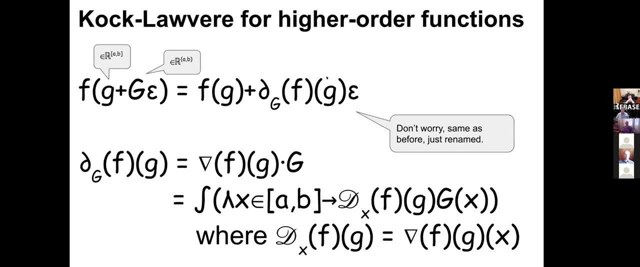 that takes a function G as a parameter, And I can define the notion of a directional derivative by the same. And again, since this thing is linear, I can define this thing here, like that. And now, if I look at the definition of inner product for functions, we'll see that. you see that this is an integral. 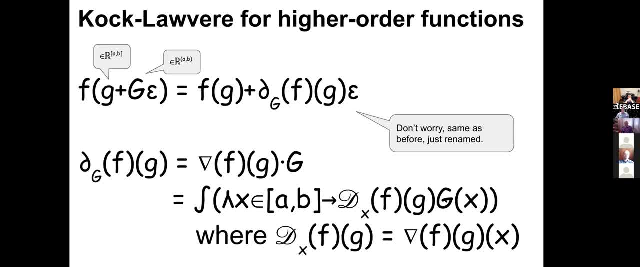 And the integral is over a product of this G with the partial derivative. So this is a partial derivative. but this is not a partial derivative on an integer parameter but on a real number. So the partial derivative just selects a value out of the gradient. but the gradient is a function. 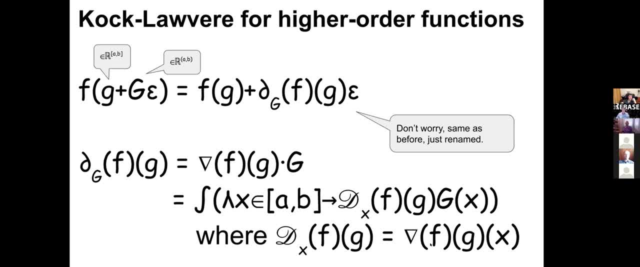 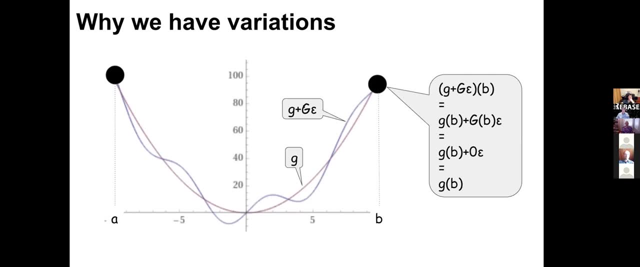 And again it just all follows just by using these axioms. Now the question is: why do we have these variations? So if you look at this thing here, I assume G was a variation and G was a function. And if you draw the picture here, you see that if I take G plus capital, G, epsilon at the endpoints of the interval, these things collide. 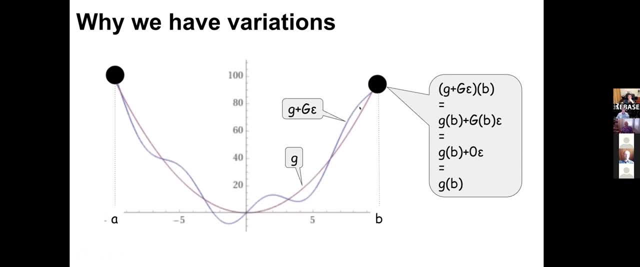 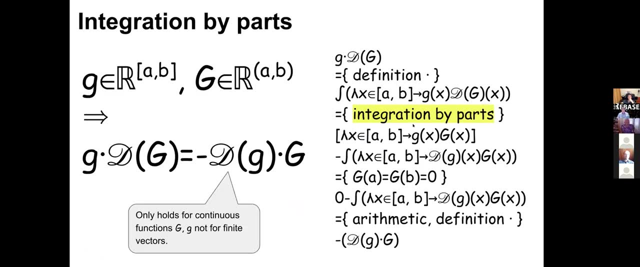 So that really makes this thing G plus G, epsilon like a variation. It varies that function a little bit. All right, Now here are a couple of other rules that I need, And this one looks really beautiful. I think it says that, Like you know, if I take the inner product of a function and the derivative of another function, I can kind of swap them and it becomes the inner product of the derivative of the previous function times the other function. 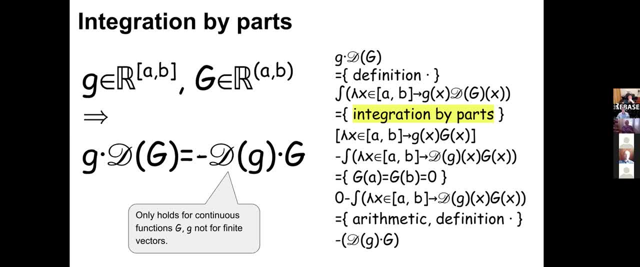 And then there's a negation here And I don't know about you guys, but this looks so beautiful to me, right, Like a rule like this. It's just like you know. I can look at that all day and just go like, wow, this is just like blows my mind. 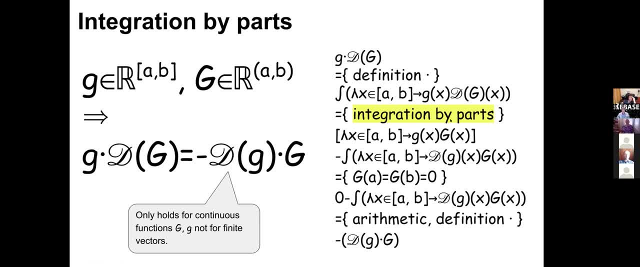 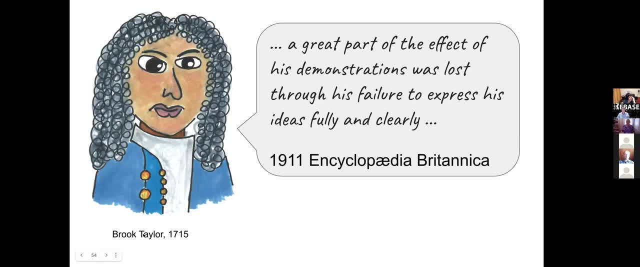 And here's the The proof. And it depends on something called integration by parts, And integration by parts was invented by Taylor, a person also kind of responsible for Taylor expansion, And I don't know People are not so kind to him. 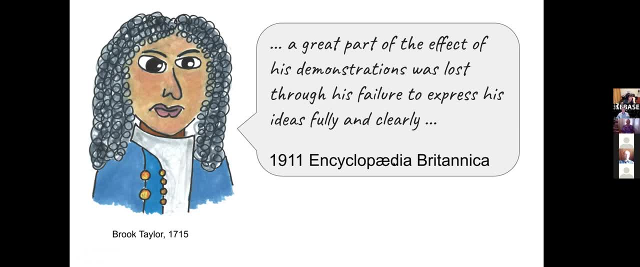 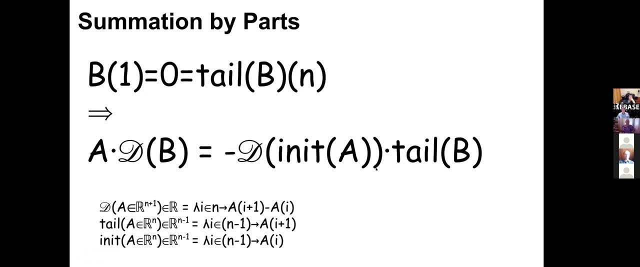 Maybe look at the quote in the Encyclopedia Britannica. It said that this. apparently he couldn't explain his work very well, But I do think that it's pretty beautiful And you can also show this thing And for In the discrete case, if you define in its entails, it becomes a little bit of layer. 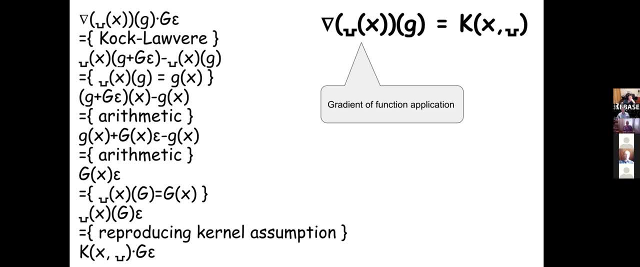 So now that we can do this, we can compute the gradients of function application, which is interesting, right? Function application is a higher order function, right, It takes a function and applies it to an argument. Well, I can compute the gradient of that. 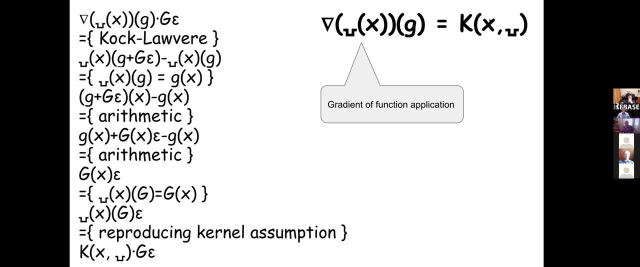 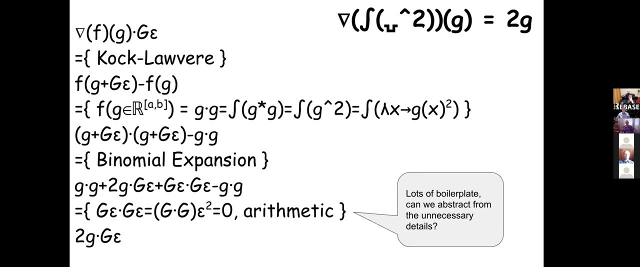 And that becomes this chronic or delta thing. That is, the chronic or delta is the derivative of function application. That's pretty deep, I think. Then here's another function here where, like you know, it takes the integral of the square of a function. 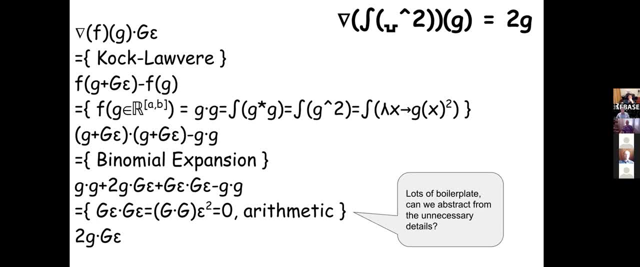 And then it becomes two times that function. Now, if you look at these two Thanks- here There's a lot of boilerplate- You see there's a lot of calculations here. That's our kind of boring. So just like we defined on lists, we defined map and folder. 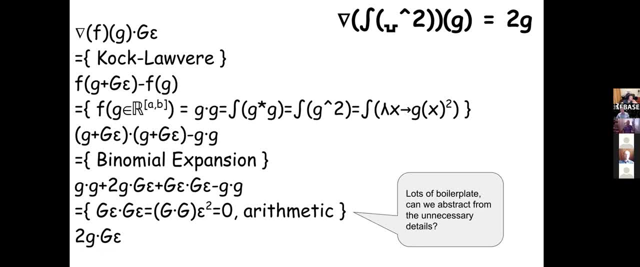 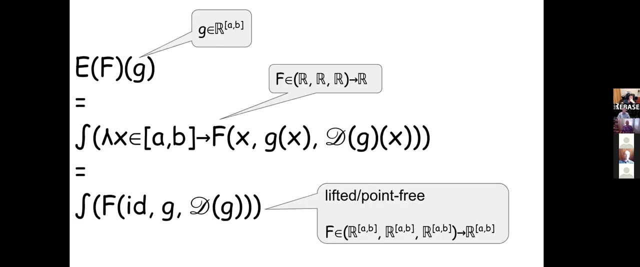 So we can define the. So let's look at it here. So let's define this function here. E, Which takes two functions, F and G, And it's defined as follows: It's defined as this giant integral. So what it does, it applies F to. 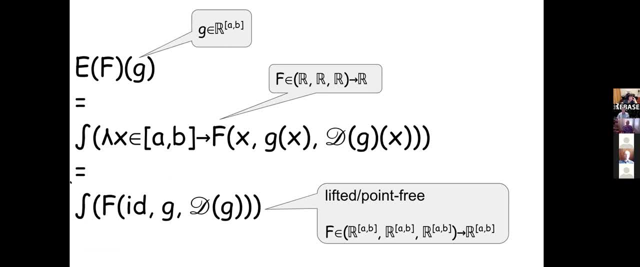 X, G of X and the derivative of G of X, And then this is the points freestyle. So so this is a super cap, like you know, crazy higher order function that encapsulates this, This big integral, And now what we're going to do is we're going to compute the functional derivative of this function. 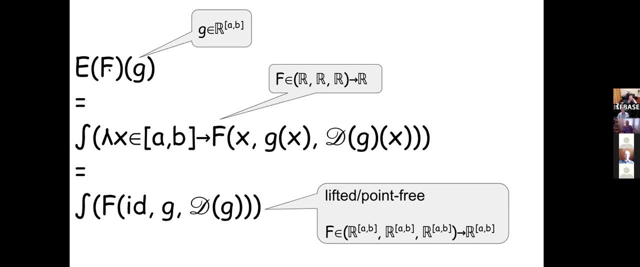 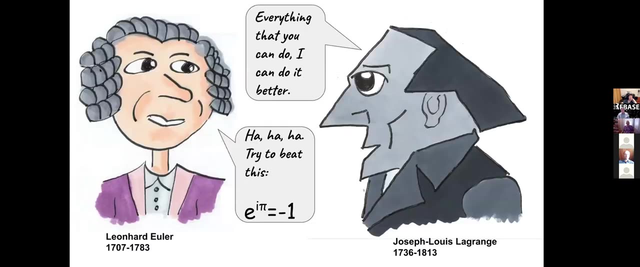 And And then, whenever we can find, like you know, a, an F, For which this we can express our function in terms of this F, we can find it's derivative, really easy, because we use the results from this And and this is really what Euler and Lagrange got, like, you know, invented, or like really Lagrange invented somewhere in 1750 or something, or like I don't know when this guy was 23 or whatever. 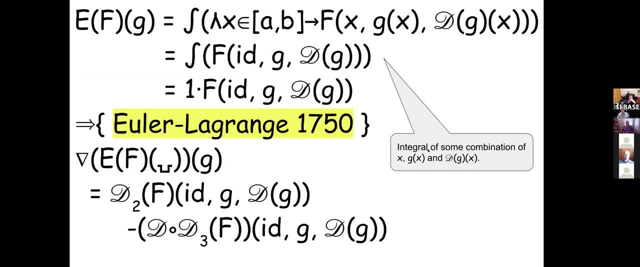 And, And, And, And. So this is where you can find the problems, And this is where you can find something that's not that easy, And this is where you can find a function that's more complex Or more complex than this one. 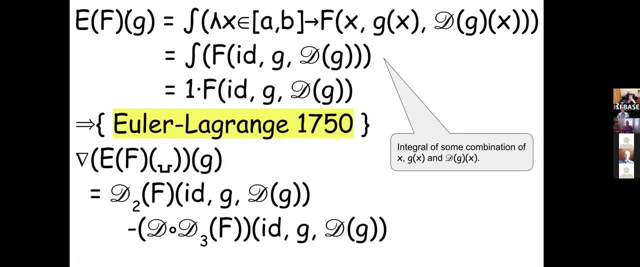 Or one that's not that easy. It's called the. So here's the, the proof, And if I define this thing here, then the, the, the gradient of that function is this scary looking expression, All right. And now you think about like: wow, that looks scary. 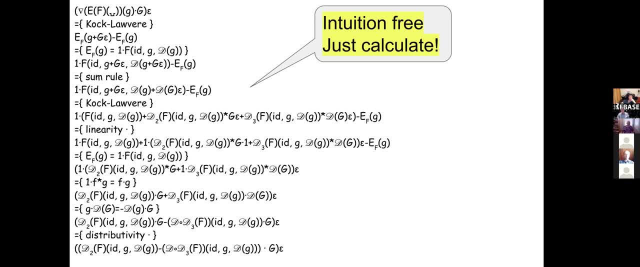 Well, Here's the proof. And again: Equal, equal, equal, equational reasoning. This is like what Leibniz wanted us to do, right, Just calculate, And all the rules are simple. These are all like use, linearity of inner product. 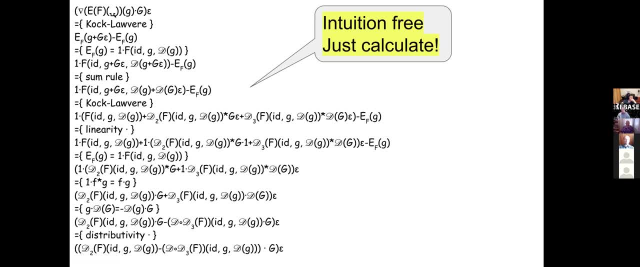 use, like you know, these simple facts. So while it looks intimidating and long, it's really trivial. It's just kept like simple equational reasoning And again, like. I think that's beautiful. And the strange thing is that in a lot of books 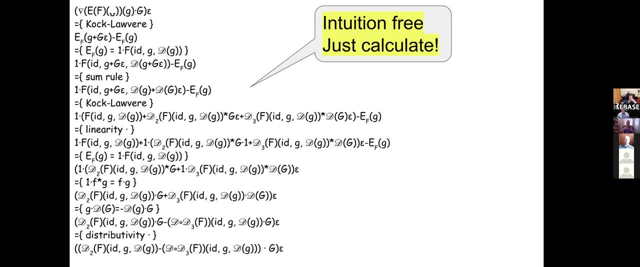 on variational calculus. people express this all using integrals and whatever. where? here we're really kind of like doing this just in terms of inner product spaces, which I think is the right thing to do. right? You see, there's no integral here inside. 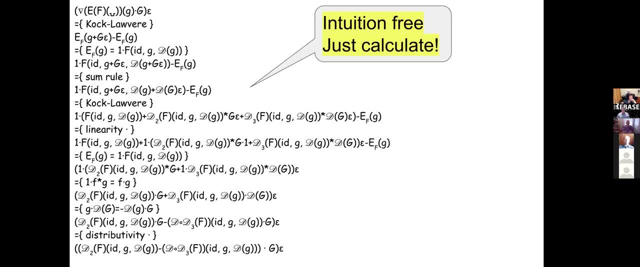 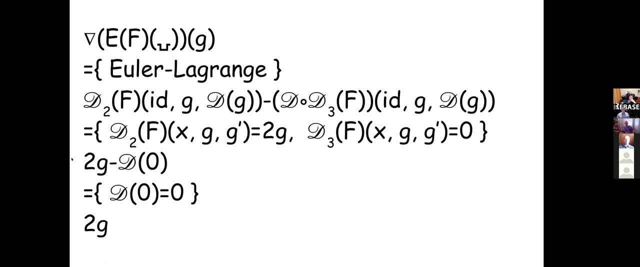 This is just purely equational reasoning, without showing the implementation details of the structure that we're working on And where I think a lot of math books, they break the abstraction and they kind of like go down in the implementation details. So for our previous example, 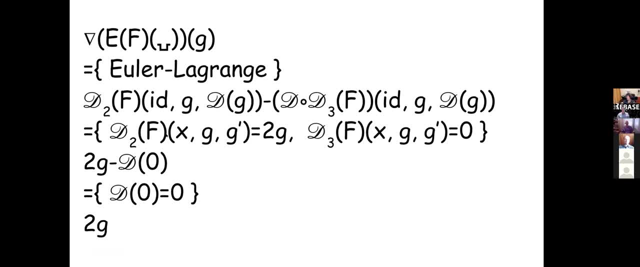 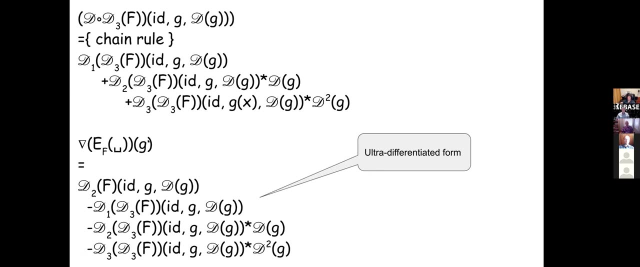 we can now show, like in like three steps, that, like you know, the derivative of that square is 2G, So it really becomes simpler and it's less work. And now, if we can, kind of like you know, write this thing here slightly simpler, 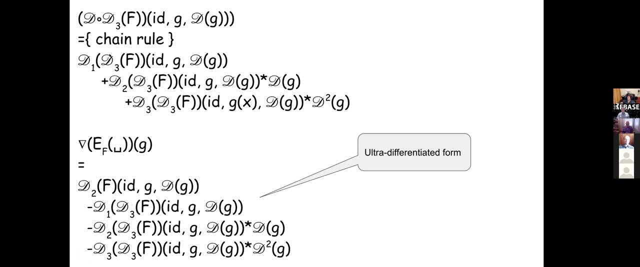 it's called the ultra differentiated form And it looks kind of like you know, maybe a little bit more intimidating, but it's again like you know, we don't care because we just calculate. So now let's look at our last example here. 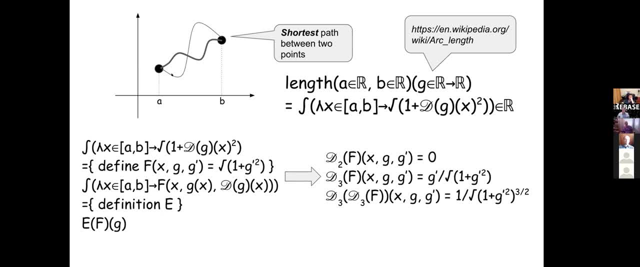 And this is we are trying to find the function that is the shortest path between two points. And of course you will say that's a straight line, right, Like the shortest path in Euclidean space between two points is the shortest line. But how do you prove that? 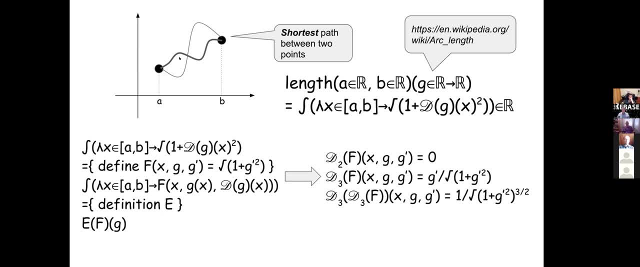 Well, let's try to prove it. The length of a of a function between two points is given by this integral. You can look at that in Wikipedia. If you look for arc length, you will find that This is: maybe you've seen this in your calculus class. 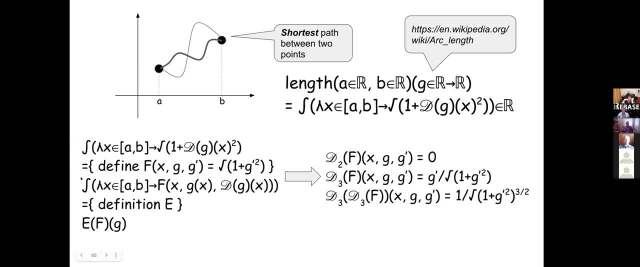 And so what we're looking for here is we're trying to find a function G that minimizes this expression here. All right, because this function G, this expression here, is the length of the path, And so we're trying to find a function G. 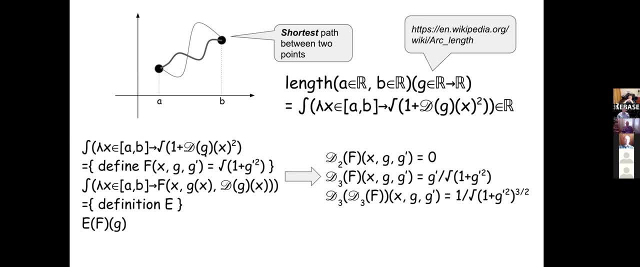 to find the function g, for which this integral is minimal. and now, in order to use this um, the, the, the higher order function, f, we need to define it. well, let's define f of x, g, like as this, and then, like you know, it's, it follows that it's e of g. with this definition of f, these things hold. 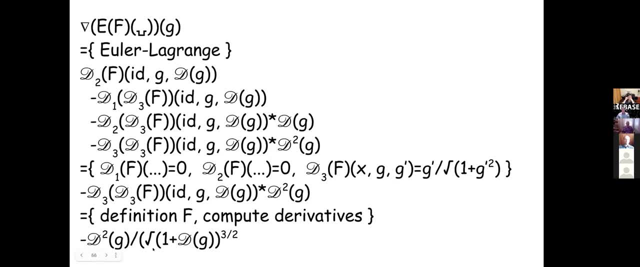 and now we can compute here and it's just equational reasoning. so now we can find that the function that kept, like you know, um or the, the gradient of that, that expression here to g and satisfies this equation here. so the gradient of this higher order function. 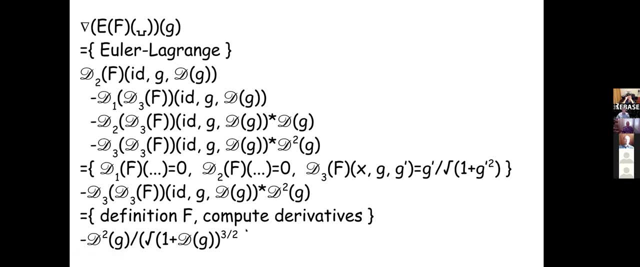 in terms of g is this complicated expression. and now what we need to do is this: this: we need to find the function g that minimizes. that's the minimum, which means that we need to look at the function g that makes this gradient zero. so we need to look for the function g that 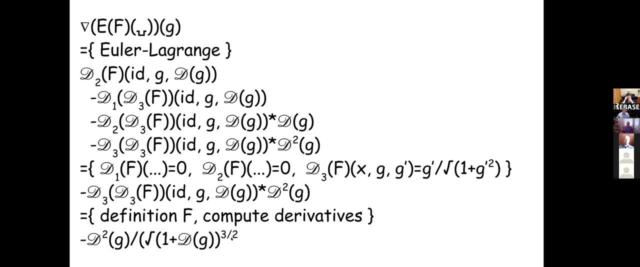 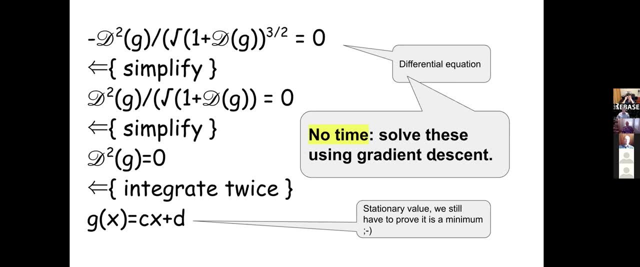 makes this expression zero, and that is um. like you know, a differential equation. we'll do it here analytically, and we don't have time to do this by gradient descent, um, and then we find that g is of this form- and now, of course, we're going to do this by gradient descent- and then we find that: 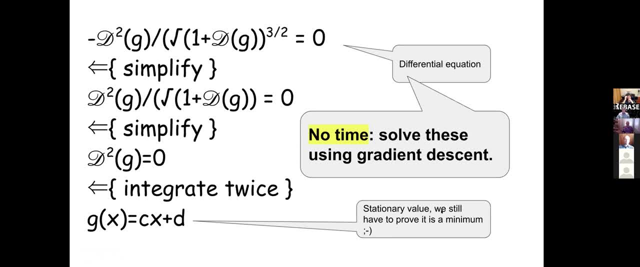 course we still. we have only proven that it's the like. you know, that it makes the gradient zero. we haven't proven that it can still be a maximum. so our proof is not yet completely done, but i think it's. this is probably good enough here. now let's see why. like you know, solving this by gradient. 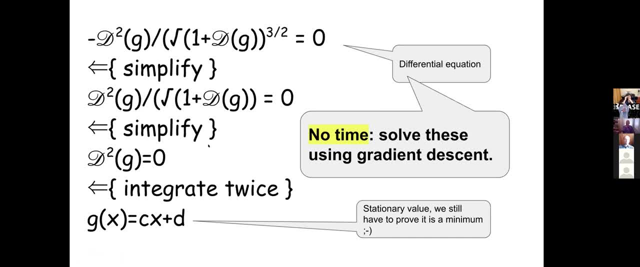 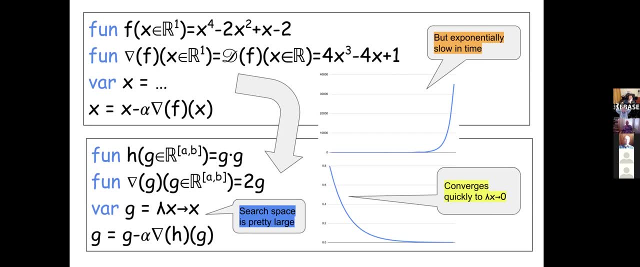 descent is pretty hard. so let's look at it like: let's end with some code- and i'm over time, but let's end with some code like in a good note. and so we saw that we do. we could do gradient descent here by taking a function, take its its gradient and then do this um loop here where we just update. 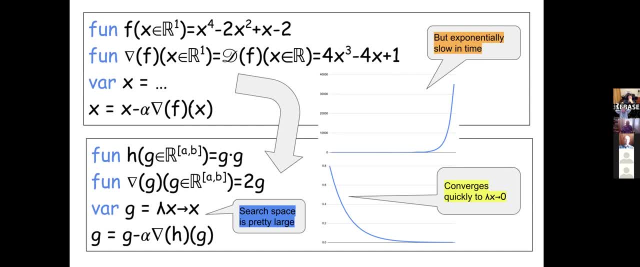 the value um using the grade, compute the gradient, update it. in this case, instead of like a single um scalar, we have a function and this let's look. look at it for our function here. the gradient was 2g. now let's start with. g equals the identity function, and now let's have like just go through. 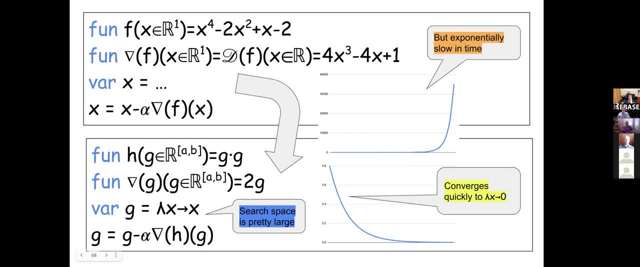 this loop, and we can't like compute, like you know, you g minus alpha times this. what you will see is that this converges quickly to lambda. x equals zero, which is exactly the the function, right. like you know, this is the one that minimizes it, so this is the right value, but it takes exponential time to get there. so even 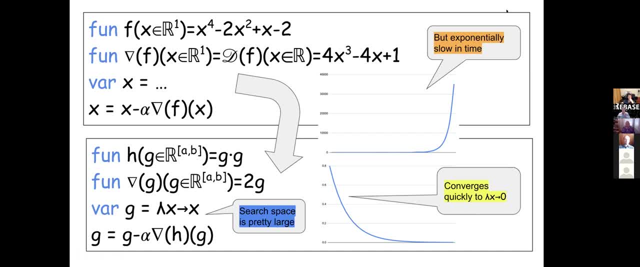 though it's, it converges in a few steps. these steps take exponential time, and why is that? it is because here i'm i'm updating an array and that's a mutable cap, like i'm really mutating the array, where here i'm updating a function and 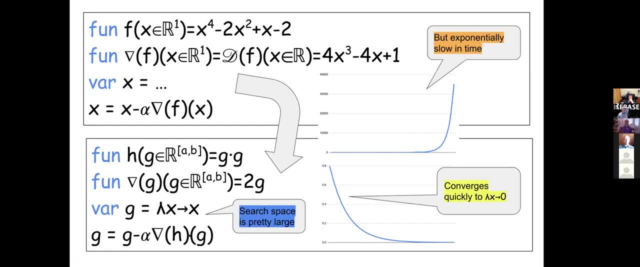 which means that every time i evaluate the function, i cannot get like update that function in place. um, so this: while it works theoretically, in practice you cannot get like efficiently update a function like this. so what we need to do is we need to like- and this is why i don't have to do this. 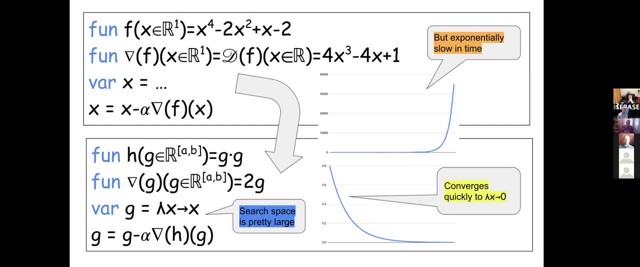 have time, we need to find a representation of this function that we can efficiently update, and that's a whole new um, a whole talk. that takes a much more time, but what you see here, that's like theoretically it just works. the only thing is that it's just got like crazy inefficient and 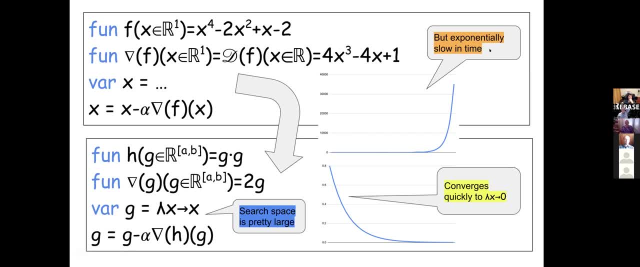 that this search space is really large, so you probably it won't even converge for anything that's less, even less trivial than this um, but you can do um gradient descent in function space. you have to just be a little bit smarter and you have to find a good representation of your 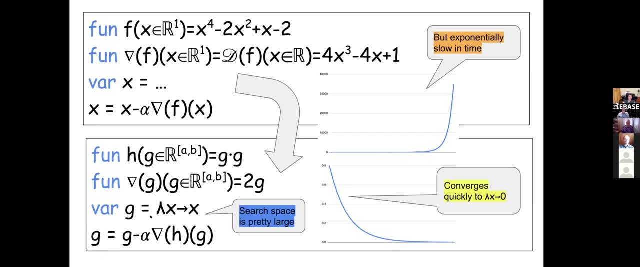 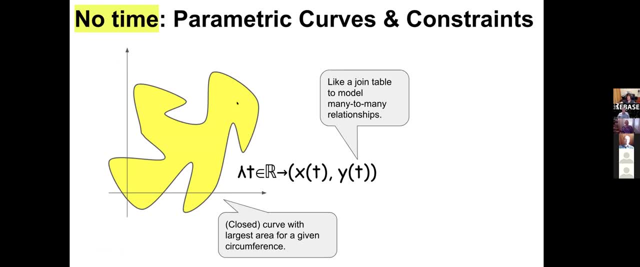 functions that you can um update in place, and the other thing that that um i don't have time for is to look at these kind of- like you know, and other curves, like you know, the area, the maximum area. in that case we cannot um deal with um functions anymore, because the shape of this curve is not a function. 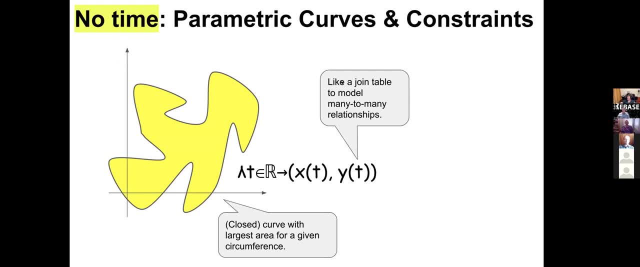 so we have to look at relations which we can model with a joint table, so like as functions from a intermediate value to a pair of values, and which i think is also interesting, um that there's, like you know, there we get another connection with um, with relational 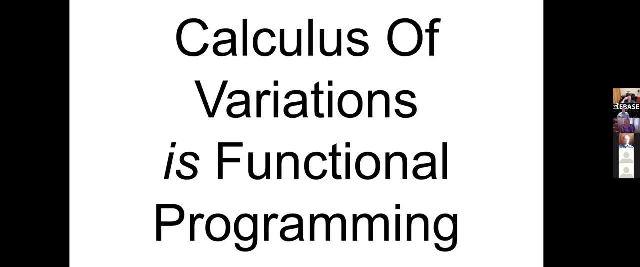 algebra, um. anyway, that was it. so i hope that you all saw that calculus of variation is really functional programming, um, and that's um. the, that inner product is kind of like the fold r for vector spaces, um, and if you focus on what is similar, then suddenly there's nothing weird here. 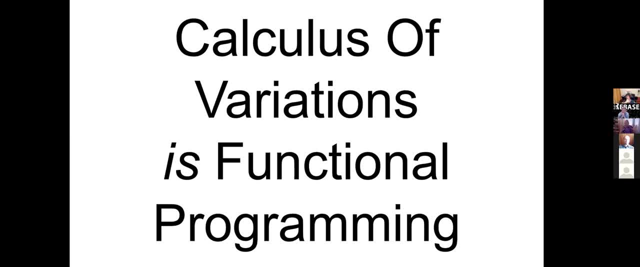 like everything that worked on on finite vectors also works for in the infinite space, um. so that that's it, um, and i, i, yeah, i, i think this was. it's pretty good. i think it's pretty good. i think it's pretty beautiful to see that like some of this got like very old math from, like you know this. 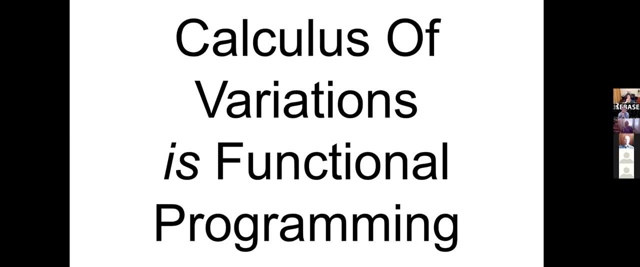 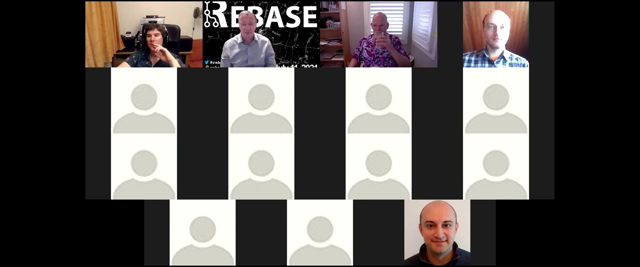 17th century really has got like strong ties to, to functional programming, um and and all the things that we, that we do um as computer scientists. but somehow the this relation is not really like shown um enough. i think. all right, thank you, eric, as, as was said, nothing we are not. 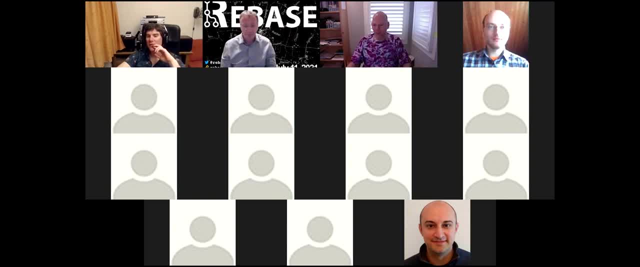 here. um, so, before we take the question and discussion, i would like alex to uh to speak. uh for a bit. share either his position about what eric said or you know what he's. he's interested in, whichever you feel like going. yeah, so i had actually a few questions about the presentation. 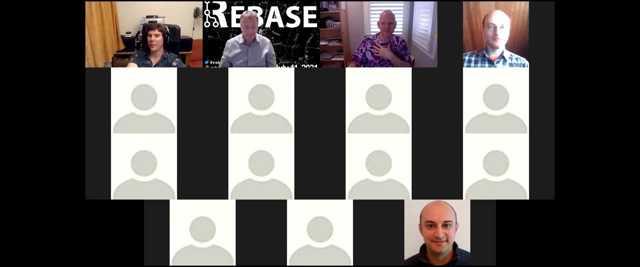 and i also wanted to say a little bit more about what i work on. so maybe that raises some ideas of what the connections here are. um, but if it's not a question, i think it's a good idea to ask. talking about what i work on, then maybe, uh, a little divert from questions about eric stocks. 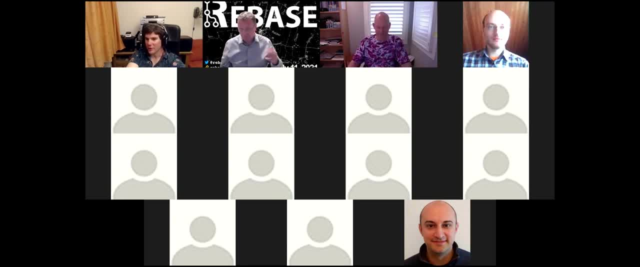 and which is fresh at the moment. so i would maybe start with asking a few questions about the talk itself. so, uh, actually i wanted to ask you about some things in the slides. so one of the things is like in the one of the latest slides. you said it was exponential, the running time of the 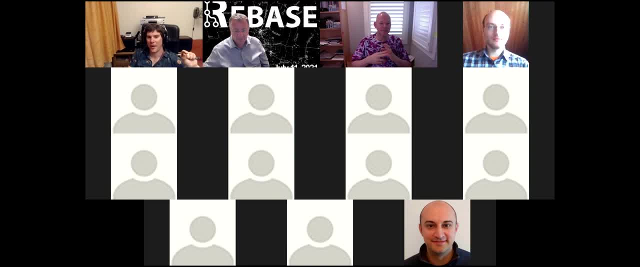 simplex when you do it on the function space, right? yep, but this is exponential. i mean, like the function is a vector with infinitely many components and not even infinitely many, but like i'll have one number of components, like on a real, on the domain of real numbers, right? 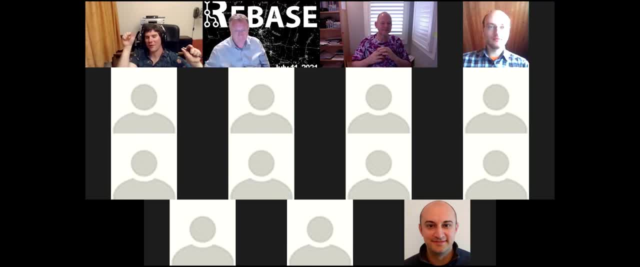 so why this? why did you say exponential space? i mean, how do you even execute one step of updating the expression with the g equals g minus gradient of g? you remember, in front of the other members, i i can explain it so too, and remember that when i defined an addition of 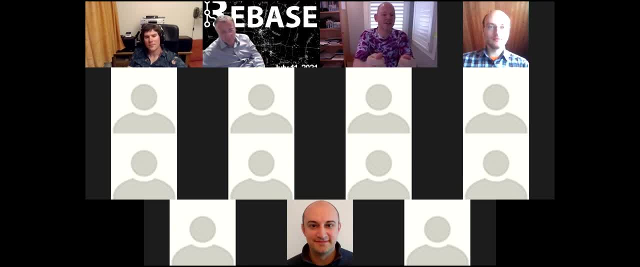 two functions. right, if i add two functions, i create a new function that takes a parameter and then passes it to these two functions. so in this case i- i have the, the expression of g equals g minus the kind of, like you know, gradient. so now these are two functions, and so what you get? 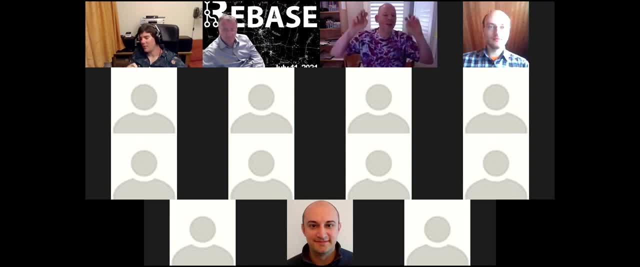 is that, like you know, if you look at the tree that you built, every time you update the function, you're not updating the function, you're just creating a new function and that grows exponentially. okay, look at the value. or when you want to take the derivative of that function, it gets bigger. 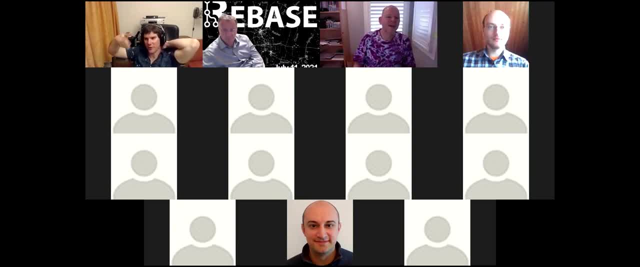 and bigger. so you build a representation for the relation for the expression and the expression- it grows exponentially. okay, yes, the trick that you need to do is to to find another representation of the function that you can efficiently update, and so the way to do that is to kind of like use. 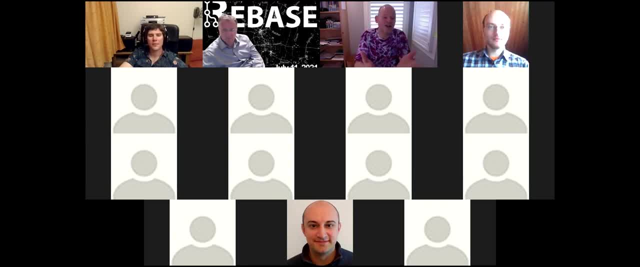 a like. there's universal function approximators. for example, a neural net can approximate any function and it's or like a um, um like a um, but they um expansion or something, and those are functions that are parameterized by weights and now you can update the weights. so the kind of 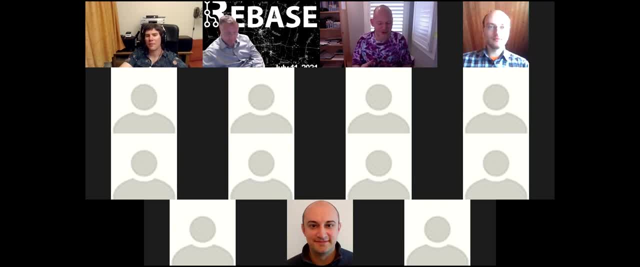 trick is like, in some sense it can, like you know, completes the circle. so you represent your function by something that's parameterized by weights, and then you can update these weights destructively, and then you can do it efficiently. but it's kind of funny here that, like, all of this really relies. 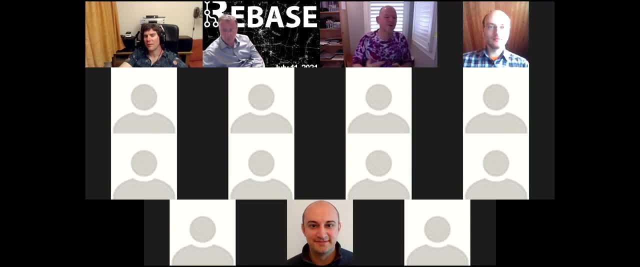 on the fact that you have to do a destructive update. if you, if you, if you're going to do gradient descent in this loop, you, you, you cannot do functional updates right, because then it becomes, it becomes linear, quadratic, whatever, because you're building this structure where you have 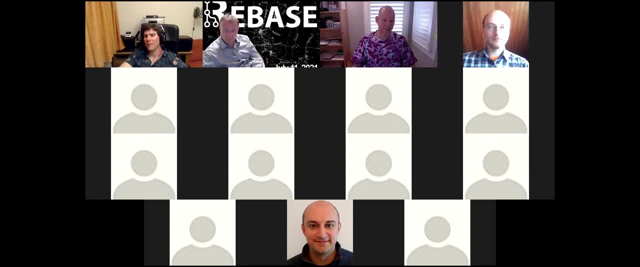 to get, like, really updated in place to to remain efficient. i see, let's just say okay, also, very um, it's very nice, right, because we're we're we're finding a function, but we're doing that by destructive updates, which i i think that's just so cynical, right? i mean, in the end, you're executing. 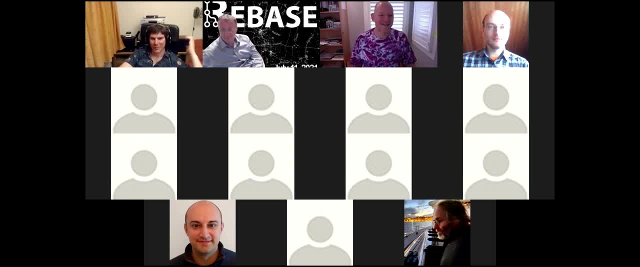 that on a, on an actual machine. so you have to do it's destructive updates at some point and so so. but, um, but then, like related to that, one of my questions is like: is the idea sort of to use this in a programming language, or to have a programming language where you sort of express this, this sort 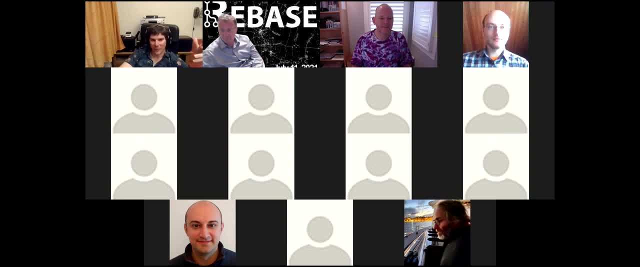 of relations, and then you implement algorithms in the programming language in which in which you can express, which you can basically implement this sort of relational reasoning, right, so like? can you actually like? what you're shown here is it was some sort of a kotlin like syntax, but can you? 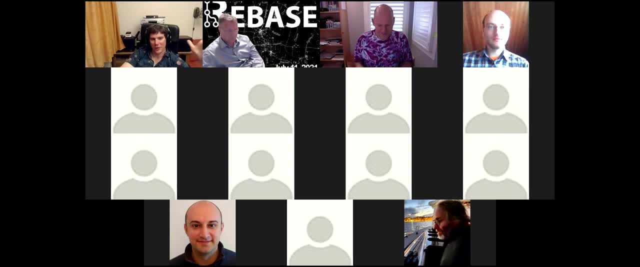 actually do that in a language and then like: how would you do that in a language? like: would you, would you like leave this approximators or something? that's an implementation detail which you decide at the end, and you just express your program in terms of these high level concepts and then you decide on the representation of your functions. 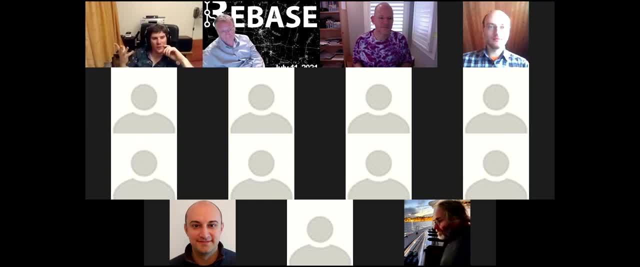 at the end and you see what kind of result you get. or like, how do you imagine like implementing that, or like having that as a programming language tool? very good question. so, um, yes, so what you want to do is, in principle, you want this to be in the programming language, right? so? and this is what we 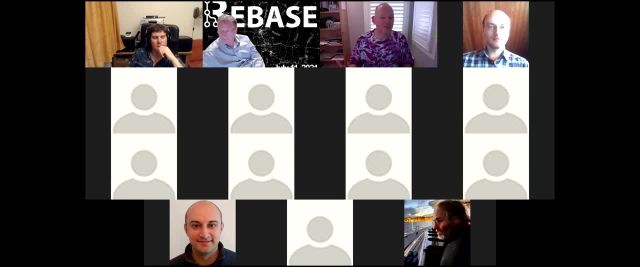 like you know, if you think about this, when people talk about differentiable programming, that's what you're, what you're doing here. so you want to make sure that we're making sure that we're every program is differentiable. um, because, like, we're taking derivatives here, um, then the other. 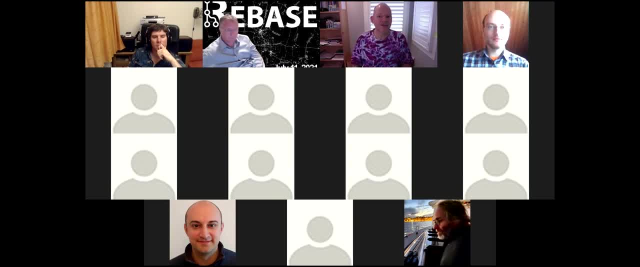 thing that you also need is integrals, like the example that i showed. like you know, they're the, the derivative of this thing with integrals didn't have integrals in them, but sometimes they still have integrals in them. then the other thing: what you saw with the um, the straight line is that the 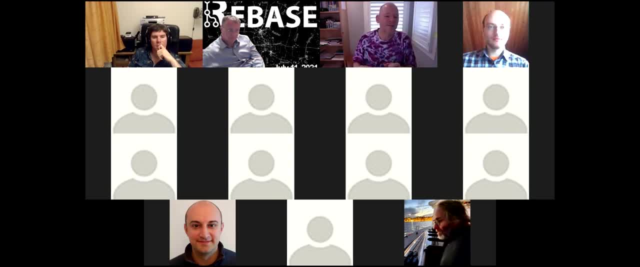 derivative still had derivatives in there, um, and so if you're, if you're kind of like executing the update, then there's still derivatives in there. and then the other thing is like i, as a programmer, don't want to think about how to represent that function, right, i want to just say 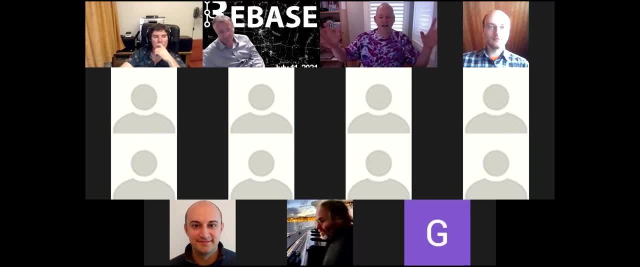 like: find a function that minimizes this um, this expression, and so the compiler should kind of come up with the, with the representation of the function that it can get, like update, um, and in some cases it's not going to be the same thing, but it's going to be the same thing: um, and so 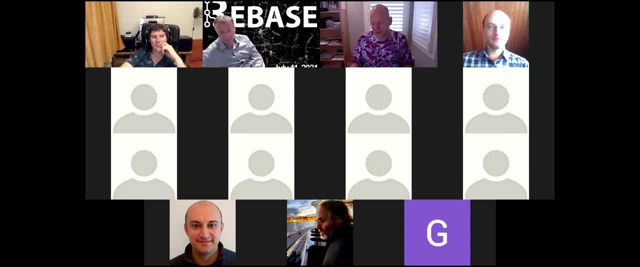 um, and so in some cases it's going to be the same thing. but it's going to be the same thing um sense. if you think about like, if you look at standard deep learning frameworks, there everything is is represented by like tensors, right like there. that's like you know your weights, but here we want. 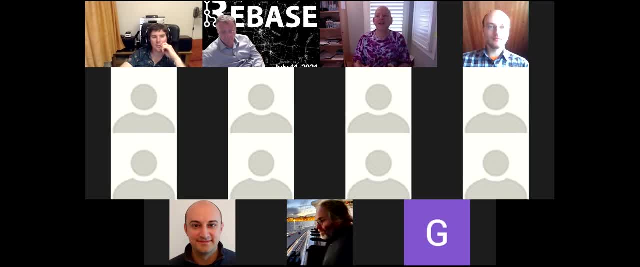 to get like: take one step further. it's like you know, we want the compiler to say like what? and there's many choices of these function representations, um, and, and. now you get into kind of things like gaussian processes and whatever. but there's, there's many ways that you can construct. 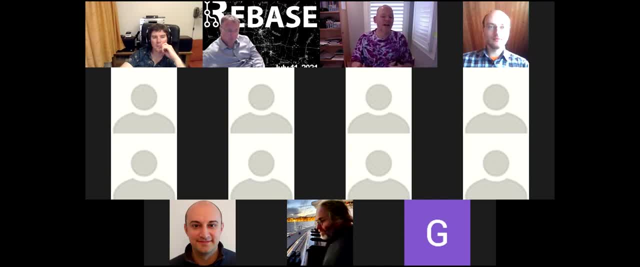 a basis in which you can represent a function, um, and the compiler should do that, um. so i do think that there's like yes, and i i've shown this here now, um, in this pseudo syntax, but yeah, what you want is like all this stuff, but now, suddenly, like the compiler is coming up with a function. 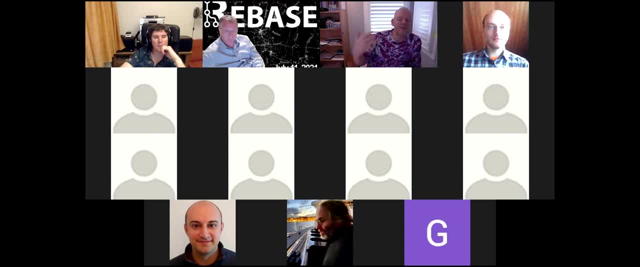 representation during this in order to efficiently do a gradient descent over function space? okay, pretty cool. um, i have some questions about the earlier slides, but i see there's some interesting question from david, so maybe you wanna uh, but, uh, let's, let's pause this. uh, finish. uh, let's finish with your. 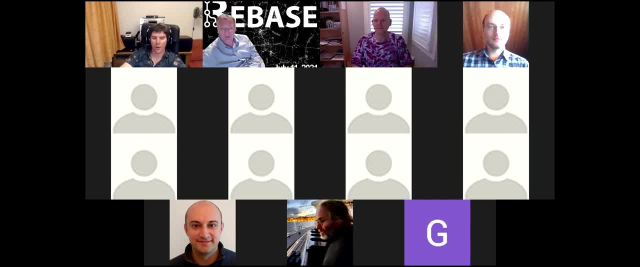 what you're doing, because otherwise we'll never get to it. um, okay, okay, okay. so i mean, i had a comment, which maybe ties in more in what i'm doing, about what you said earlier, uh, during the talk, which is that people are imprecise about semantics and 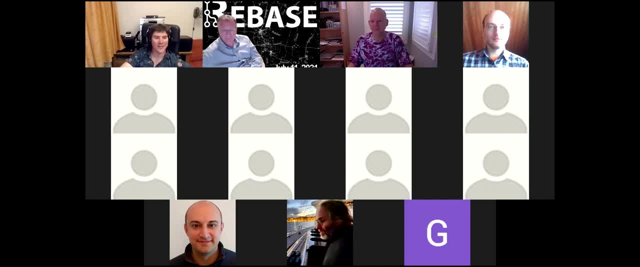 in particular, the f sharp and the c sharp ends up being the same thing, because, if i got you right, because they are not the same vm right, but which i mean as a side note is something that you could say about n into programming languages, because in the end they run on some sort of a process, cpu. 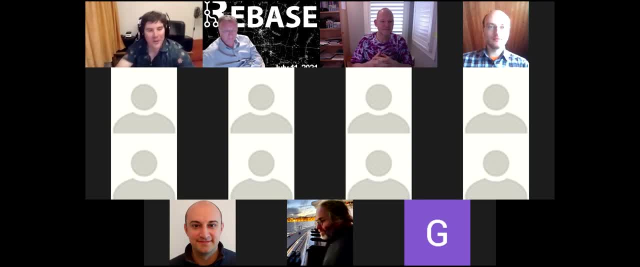 right and uh, uh, so i didn't quite like get you completely there, but it maybe ties in, uh in in a bit of what i'm doing is i'm like doing some work in in the area, uh, of virtual machines and i a few slides that i wanted to maybe show quickly to people, if that's okay, and i think that's um. 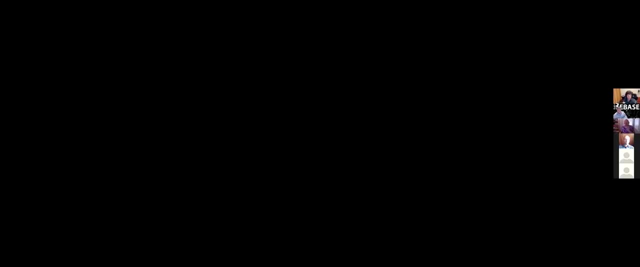 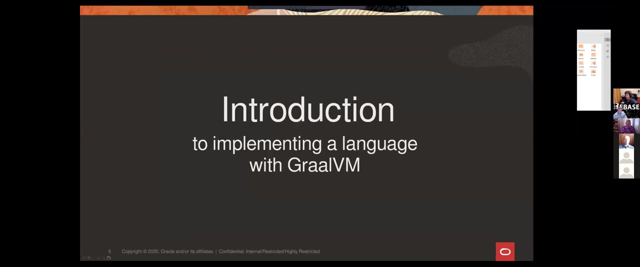 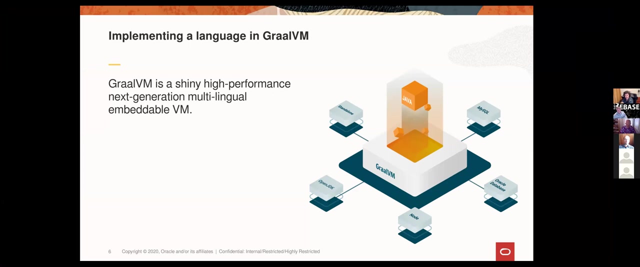 yeah, so i'll share my screen and it's uh, maybe, uh, the fastest way to to kind of showcase. so can you see the slides? yep, and now when i said full screen, you'll see them, okay, so so basically, i'm working on on grow vm right, and one of the recent projects that i had is the implementing one new language. 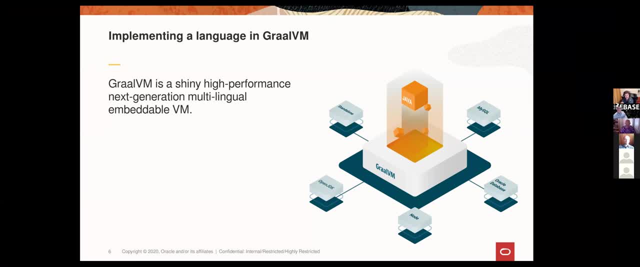 on top of this, grow vm, and grow vm is a virtual machine that's meant to be extendable, uh, with new programming, languages and, and the question is, how do you then implement a new language? and it's it's kind of interesting, because you don't need to implement the low level part of the language. 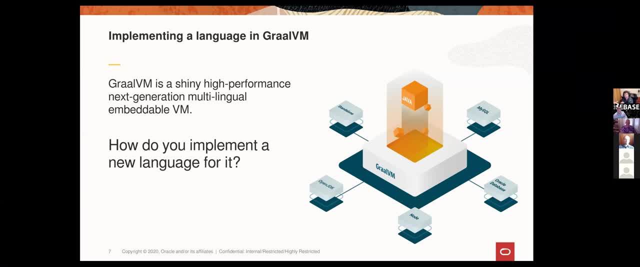 it's kind of automatically derived for you from the semantics of the language that you define. and you define the language semantics by essentially defining an interpreter, and the steps are basically in this, in the, in the framework that the vm gives you as a language implementer, is to: 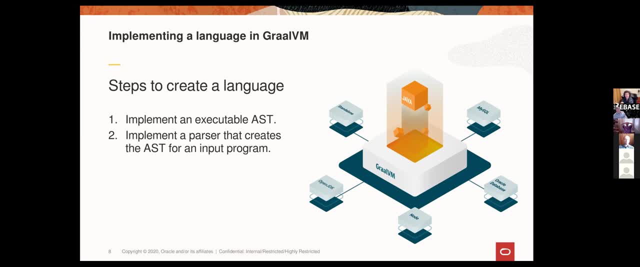 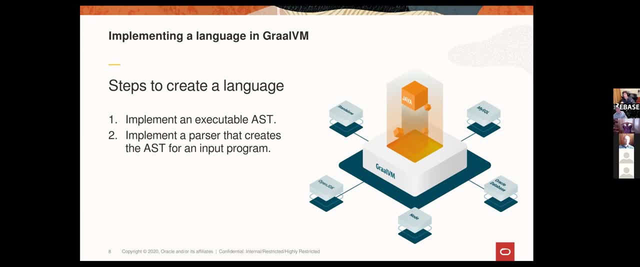 executable ast. it means you have a set of rules which say how, uh, basically the ast, the, the program, evolves, your, the state, the state of the machines. it's a little bit different than, in that sense, from functional programming where you would have, basically, your state would be the expression. 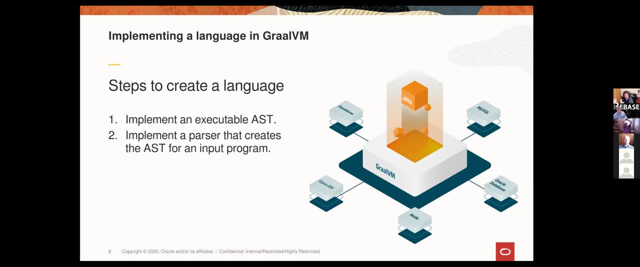 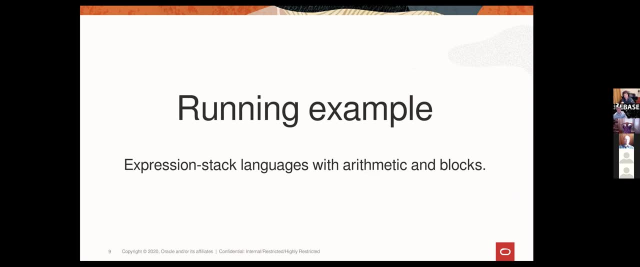 and you have a set of rules with which you're evolving the expression. here you have an ast with which you're evolving the state of the program, right, and here i want to give you a simple example of a simple language which has an expression stack as its state and then it has some restricting blocks. 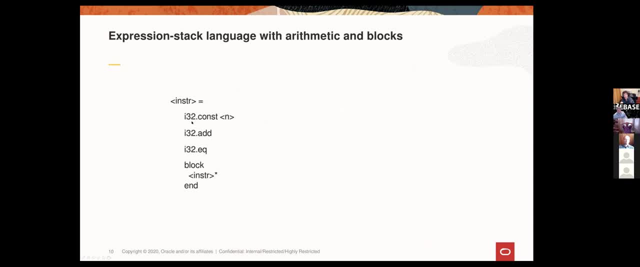 And here's the syntax for that is: you sort of have certain commands and one of them is like: push a constant to the stack, add two things from the stack together and push the results there. check if two things on top of the stacks are equal. 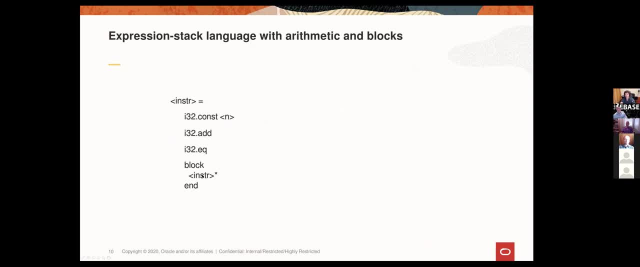 and push zero or one and then you can have a block which is a nested list of instructions. And if you have an example program, essentially the semantics works like this, So you have some program state right And if you push, you can push seven and nine to the stack. 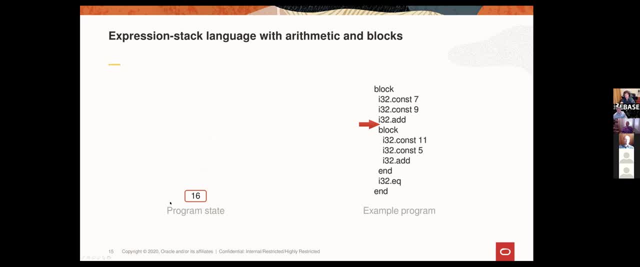 and you add these things together and you have a new value as a program state, you can enter a nested block. then you push 11 and five, you add them. now you have 16 and 16, and if you see, if these two things are equal. 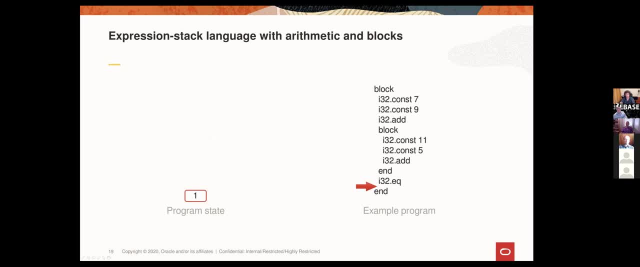 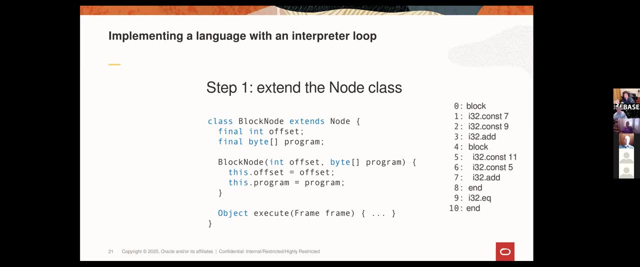 then you get one as a result. So that's an illustration of how this works, And now, in this sort of framework that we have in GraalVM, the way to express these semantics like this is to write an executable AST. An executable AST is just something. 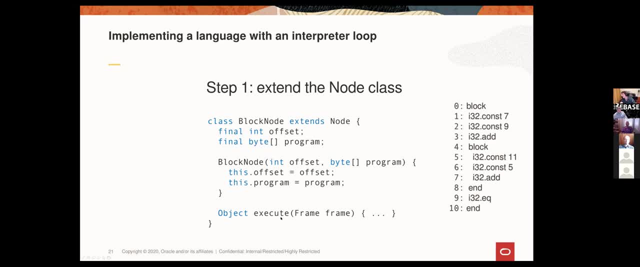 that extends a norm, it extends a node and then it has- Is there a question? No, Okay, so essentially this is So: the executable AST is essentially a class which extends a node class, and then you have to have a method called execute on it. 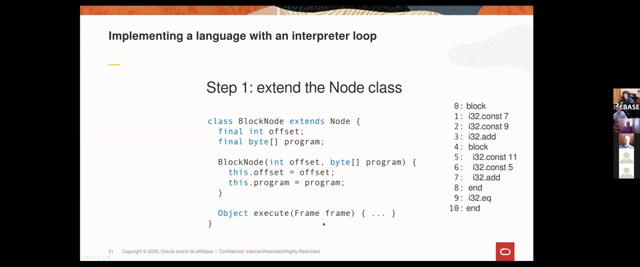 And this method called execute basically says what happens when you execute this particular fragment of the language And you can think of these frames that you give to frame as an argument, as an array of local variables, and you can use it as an expression type, for example. 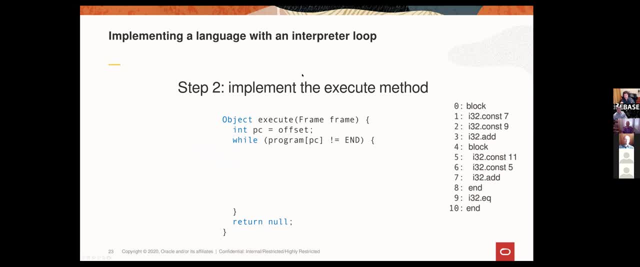 And typically how you would do this is that you would you would write some sort of an interpreter log So you would say, initially, my offset is zero and then, while I didn't reach the end instruction of my program, I'm just doing a switch. 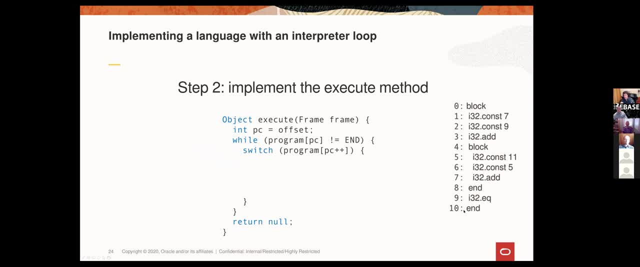 on the current offset in the instruction, in some set of instructions, and then I have different cases to implement them. So if I wanna add two things, I pop two things from the frame and then I push a result, And so you just implement this thing. 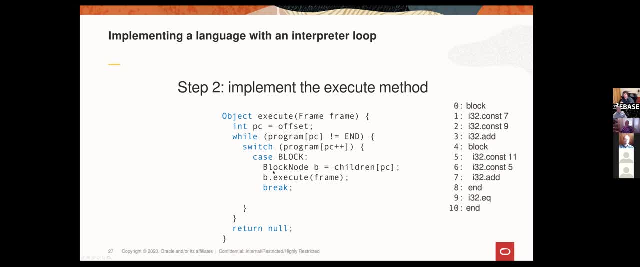 And so if I have a block then I can recursively have like another block mode for the child which will correspond to this section from four to eight, then call, execute on that And essentially I end up with having an AST which has offsets into the instruction array. 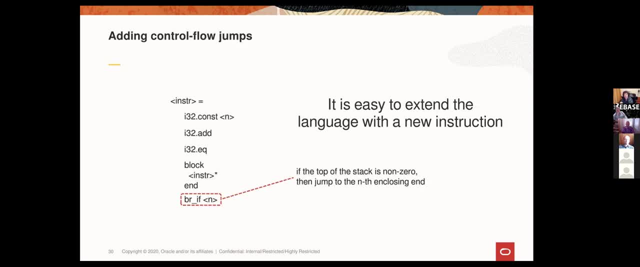 And of course, you can extend this language with new instructions like jumps, So you can like change the current program counter depending on the value on the top of the stack and you can decide how much do you jump on. And okay, so then I can show you. 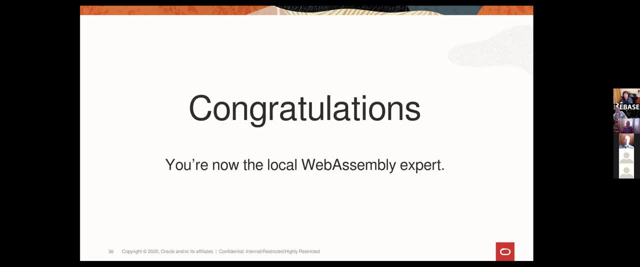 let me just skip over that. And the point is like this is basically the core of WebAssembly as it turns out, which is like this language for the web And you kind of when you see like these three instructions, you know like what WebAssembly is. 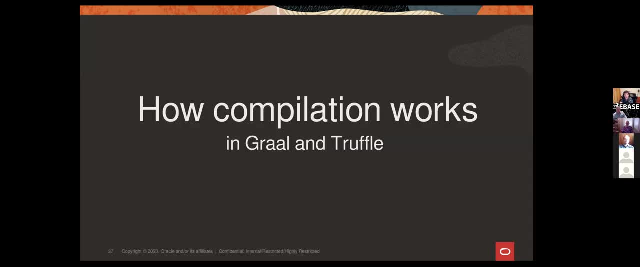 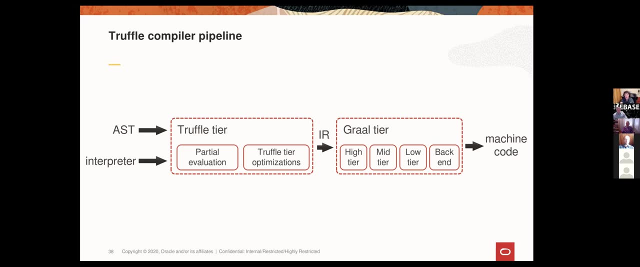 And this is basically the language that we're implementing in this project. And what's specific about GraalVM and Truffle is that after you define an interpreter, it essentially uses partial evaluation tool for any AST. where an AST is one call target or like one little function. 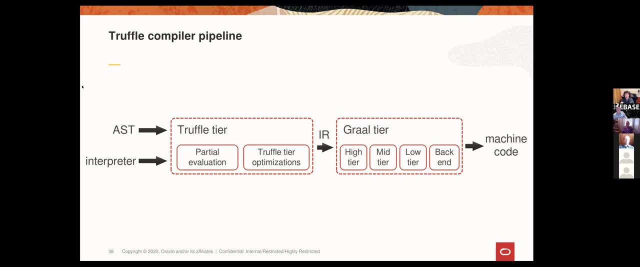 In your program it can specialize that particular function for the interpreter of that function. So basically you give it an interpreter and an AST and then basically does this partial evaluation process where it tries to simplify the interpreter, assuming that the program that it's interpreting is constant. 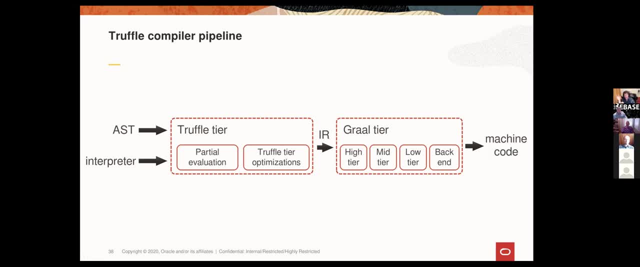 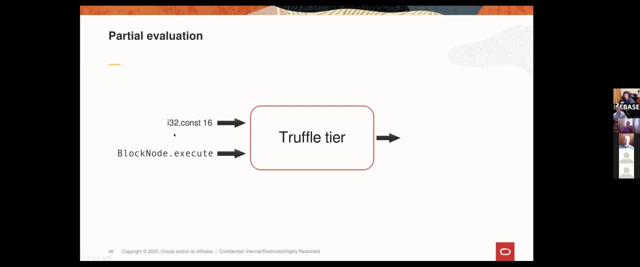 And that way it can specialize the interpreter for that particular program and then you get like very efficient machine code in the end. And to illustrate how that works, let's say that the program is i42.const16.. It's a very simple program that just. 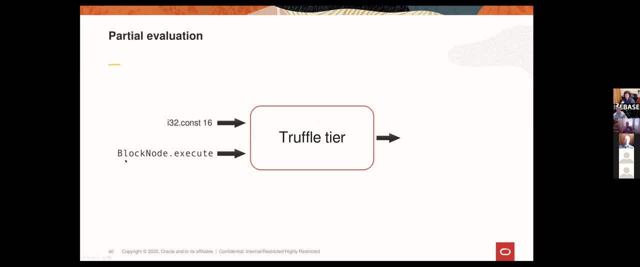 pushes a constant in the stack. And what's the interpreter? The interpreter is this function called execute. right, And the way it works is. you now look at the body of execute, you look at this AST and now you try to think what is constant in these variables? 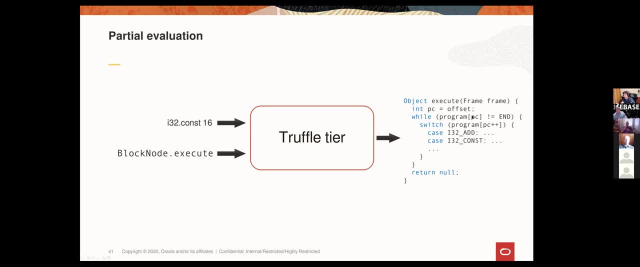 and fields that I'm like referencing here in this program and start replacing this in constants and then folding constants essentially. So this is the partial evaluation step. So the first thing is you know the offset is not whatever. the offset when you start the program is zero. 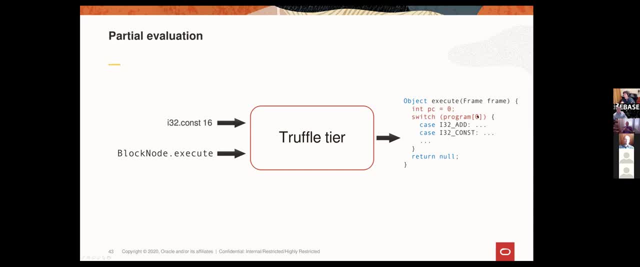 Okay, So if I put zero in the PC, then if you put this zero in this program, read of the program array. and the program array is just the array of instructions. then I can read what's at the program array at index zero. 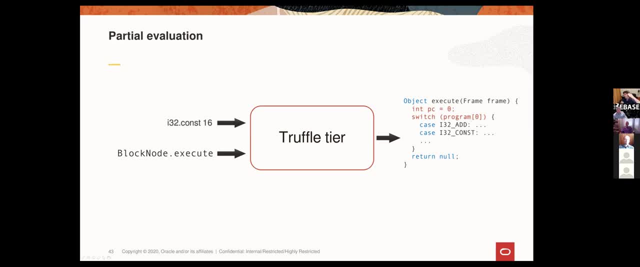 because the program itself, the AST is. it itself is constant, right, So I can replace that with a constant, and the constant at location zero for this particular program is i42.const. That's the opcode of this instruction. Okay, And that means that I have to switch. 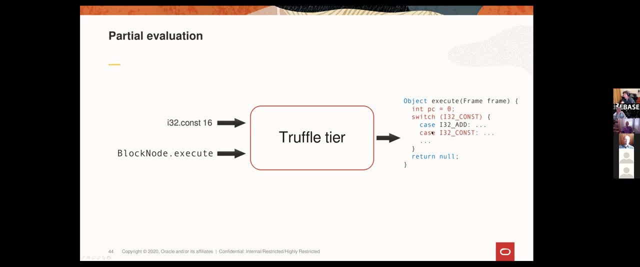 to this case. Okay, So I can eliminate the switch and I can eliminate the other cases and just leave the body of the particular case that I would jump to. Okay, And now we have to see what's on the next position: PC plus one. 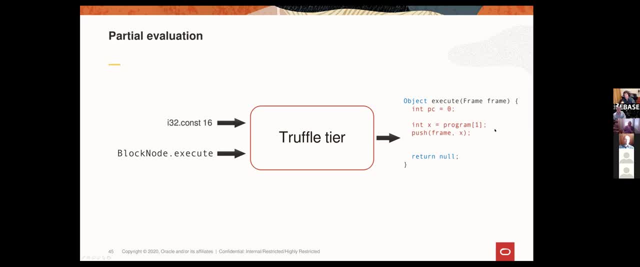 Okay, That's one. So program one is this: constant 16.. Okay, So we can read that and we can put that to the frame And in the end you know if you simplify this push, and then the fact that we always return. 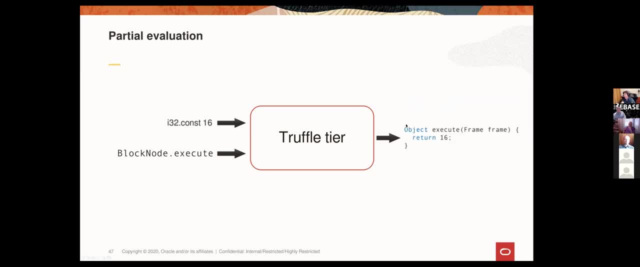 the zero location of the stack. that ends up being just returning 16.. Okay, So that's now the intermediate representation of the partially evaluated program, which is this program for this interpreter. Okay, Now that you have something that just returns 16,. 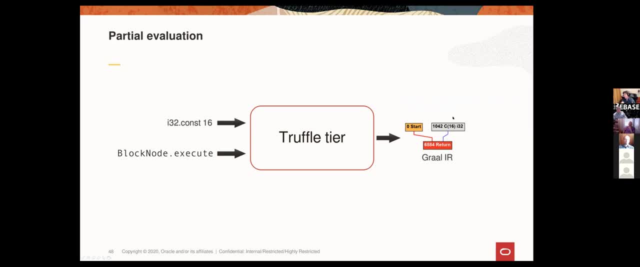 you can emit very efficient code for that And this is an internal representation used in your LVM And, of course, from this it emits assembly in the same way that it would emit assembly for, you know, compiling some Java method, And essentially this is what's interesting. 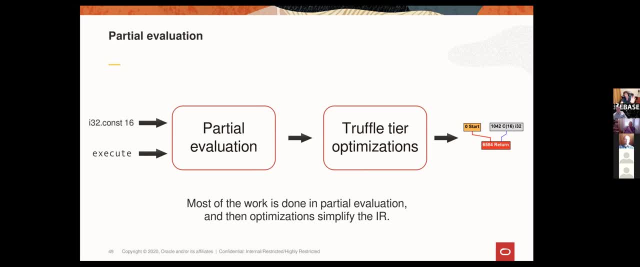 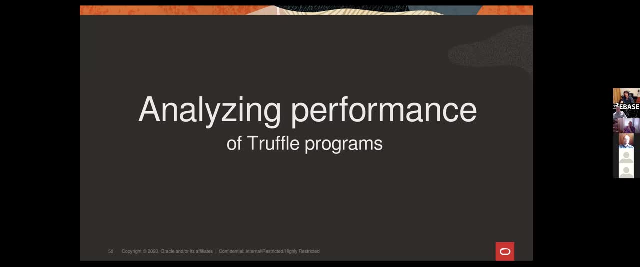 about this partial evaluation is that you, you know, define the semantics on a very high level And then you get this partial evaluation process for your interpreter for free and you get very, very fast code And that's a little sort of segment and a little bit. 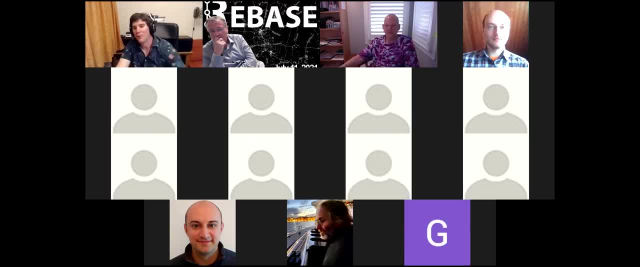 about what I do and work on. that maybe ties in what you were talking about, because what occurred to me during your talk is that somebody could actually implement an interpreter for the language that you described, And so that could be an interesting project, because then you would get like all this low level. 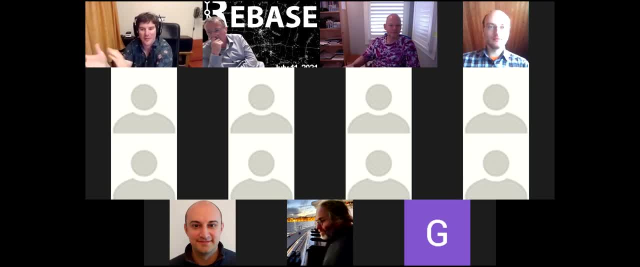 optimizations for free, because you would just define the semantics of the language that you were describing, which does basically calculus and functions as an interpreter. So do you think that that will be possible? Is that something that's feasible? Yeah, so let me kind of like you know. 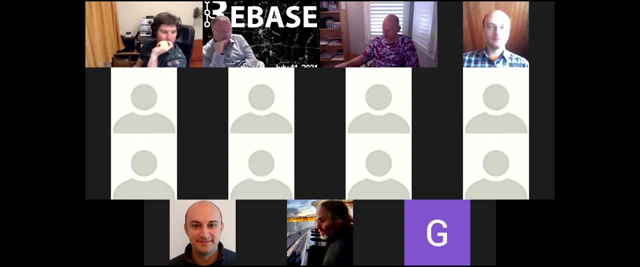 answer that in two phases. So the first one that, like the first question you had, is like when I said, like you know, like you have to, that people kind of like confuse languages say that they're different when their semantic domains are the same. 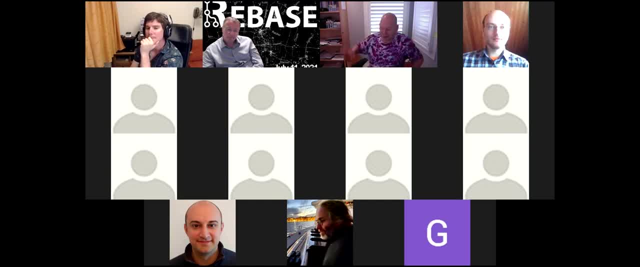 And so for me, if you look at the notational semantics- and probably I'll step on a lot of toes here, but the notational semantics is also nothing but writing an interpreter in a certain meta language, right, And what you saw, these semantic domains. 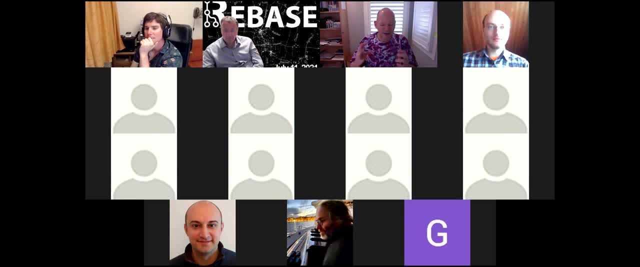 that were in my slides they kept, like you know, are the data structures that you can use in your interpreter And you have to be kind of careful that, like when you write your interpreter, that it really kind of like actually represents, you know. 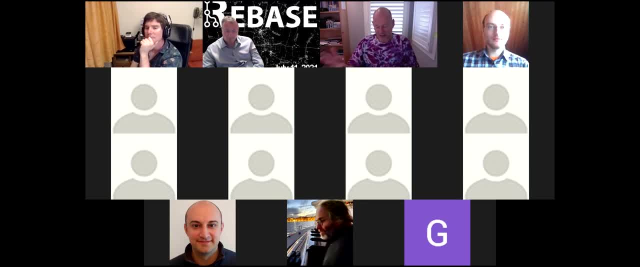 the language that you, that you compute right, Like, for example, if your language has slightly different semantics for exceptions and like C sharp has different semantics for exceptions than Java, if you look at kind of like try, finally blocks. And now if your interpreter is kept, like you know. 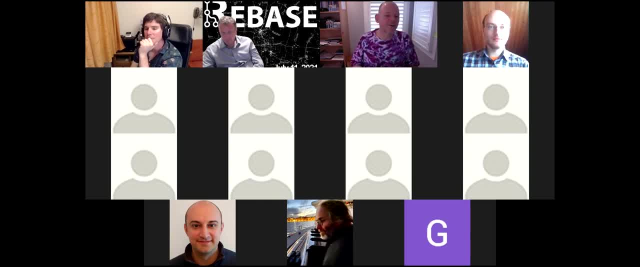 using the underlying implementation of exceptions of the meta language, then you might have the wrong semantics, right. right, and that's kind of what i mean it's like. so in some sense, like you have to make sure that your interpreter describes exactly the right language, um, and sometimes it means that you 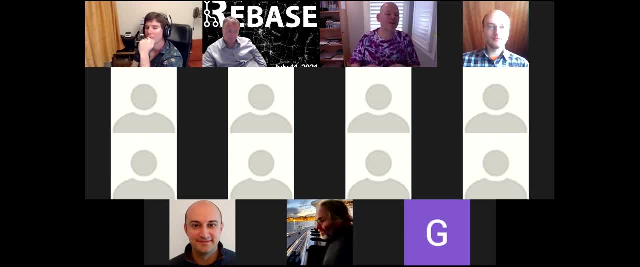 cannot borrow the like. you know the function space of the meta language, because the function space of the language that you're trying to define is different um. so in that sense, i think there's um. i like it that you define an interpreter, because when you define the interpreter, you 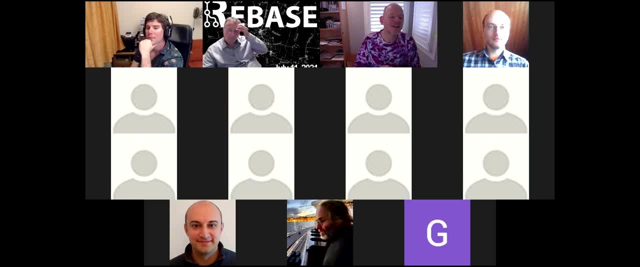 you have to be mindful about. like you know what your program means, um, and, and, and. often when you compile into like an intermediate representation, people don't really think too much about. like you know what your program means, um, in that sense, because it's easier to borrow the underlying 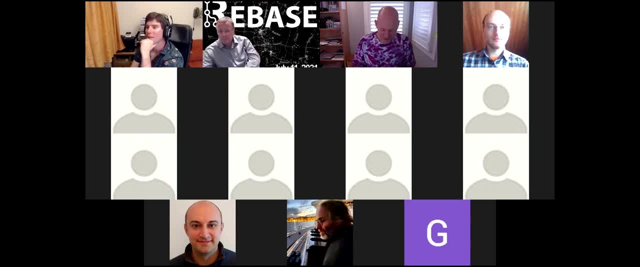 control structures, um, or lack of control structures. and now, in terms of, of using it like this: yes, because if you look at the gap, like, i think this is very interesting, because if you look at the, the, the, the function representation, if you use polynomials or something else, in some sense that's a very 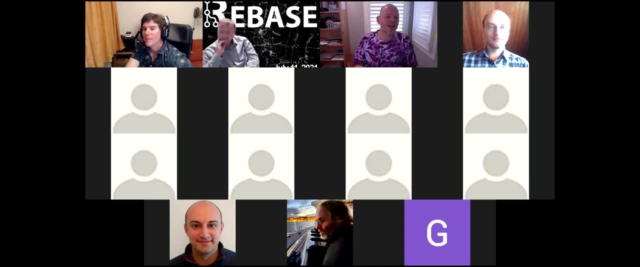 primitive way to define a language, right, because you say, oh, my structure looks like this, um, it's a polynomial. and then you know, like the interpreter is, when i evaluate this, at a certain argument i compute this thing um. and partial evaluation is also interesting there, because a lot of these 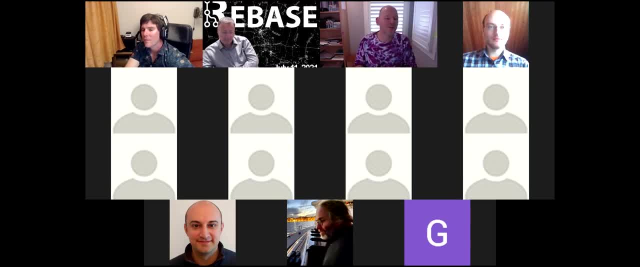 values are known. so you, you, you can remove the interpretive overhead. so instead of having like a general thing that just because a neural net is kind of like an interpreter- right, it is an interpreter that takes the weights and they got like all these other functions and then computes it, but if you could partially, 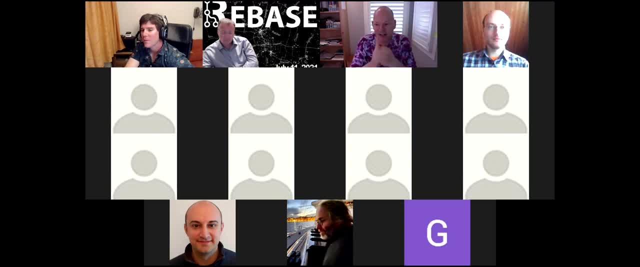 evaluate that. i think you that that is super useful, so i think that's a very interesting um question is: can you have a function representation that you can update um and then still efficiently execute it? yeah, so, um, can i add one question from the uh the chat? now David is asking: 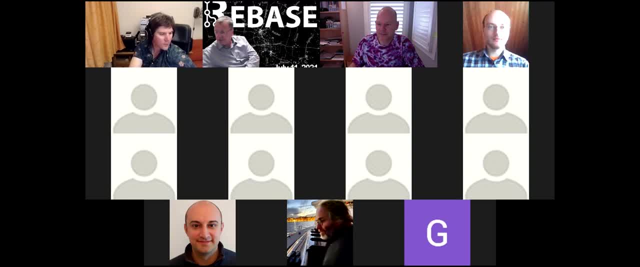 when learning function, does it also make a difference to represent them as a list of instructions or, more functionally, as in a, a pointless encoding eg, as the composition of some more primitive functions, versus as ast3, to be able to not care about structure. so let me try to answer this. so if this is, like you know, related to my um, 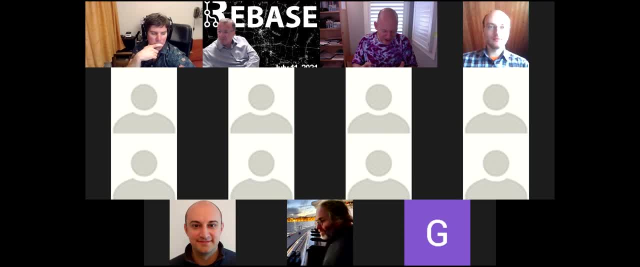 my, my talk, where we need to have some representation of a function, as we're doing gradient descent. um, i think there the the representation of the function. there's two things that you need to do. one is you- you are kind of, like you know, learning this function by. 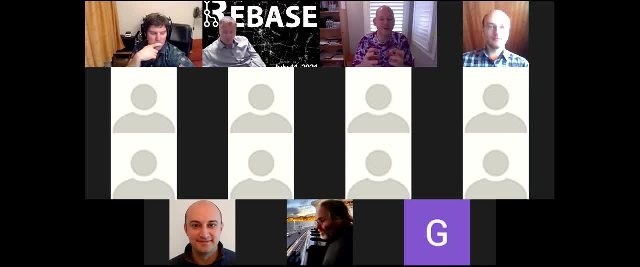 successive updates. right, so you're. you're starting with some function and then you're mutating its representation based on every iteration of that loop. so that is something you have to do to be able to do efficiently. so you have to create a new function based on a previous function where 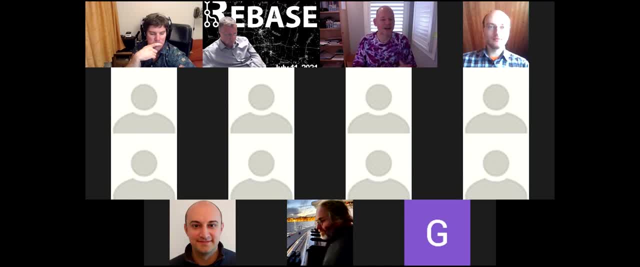 that's when you execute, that it shouldn't get, like you know, like turn into something of the size of the number of steps you've taken, right, so you should kind of get a kind of like is the smallest possible function at every step. the other thing is that that function itself often contains um. 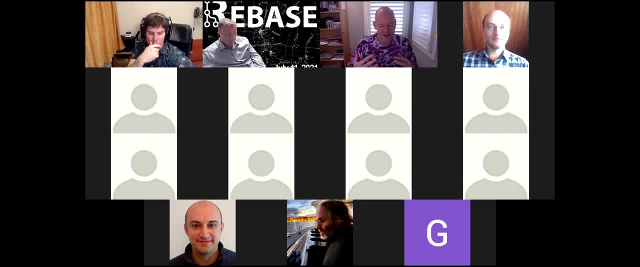 differentiation um as well. um, so it should also have itself be kind of like differentiable um, and i'm not sure that they get like whether you represent them as a list of instructions or an ast um makes such a difference. um, i think what people typically do is they use some kind of like of these universal representation. 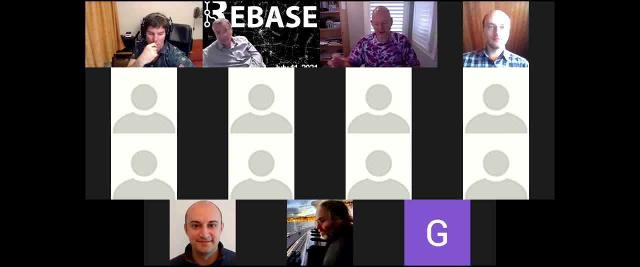 there's always some separation of the state, which is the thing that you update, and then a fixed set, which is the, the gap, like the structure of your model, and that's the way you make it kind of like um updatable, because the only thing you need to update is the weights and not the the structure. 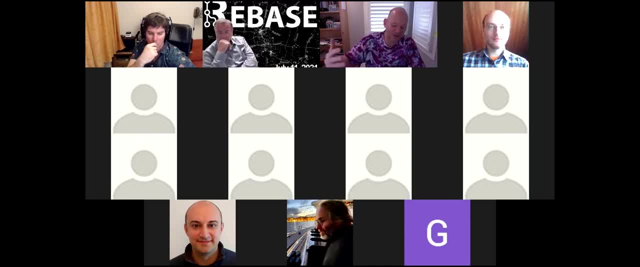 of the function remains static in some sense, or you can add to it um in in in some sense, uh, um, but yeah, but typically the the thing that's mutable is is the states think of like an object where, like you know, the methods are fixed but you get like are changing. 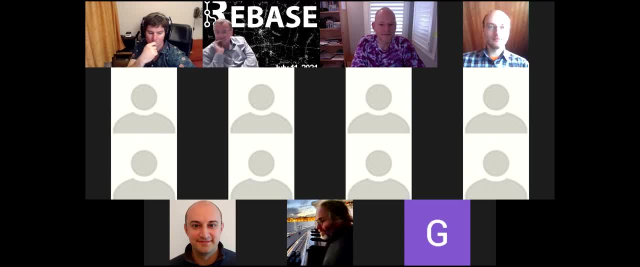 the, the, the instance states, um, but i do think that it's interesting to to think of, like you know where, also the, the actual like you want to have self-modifying code in some sense, where we're not just the state is mutable but you can like literally get like updates, the, the code of. 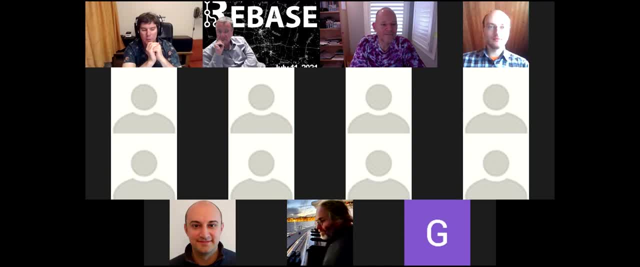 the function. yeah, i mean like the crucial bit there is to get this differentiability right, because that's what you need if you're learning it and, like you're going, probably at the same, yes, yeah, you keep taking the gradient of that thing right. so, yes, it has to be differentiable as well. 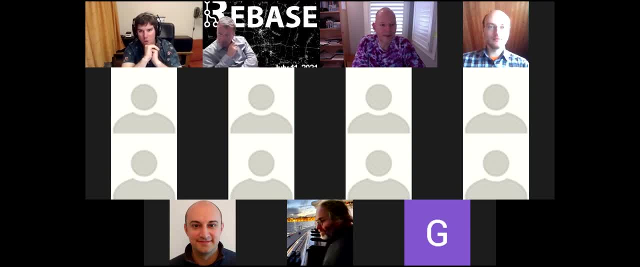 So I actually have a question like regarding to that, because you're, like, in your talk you were talking um, so you started, like you mentioned like, uh, like linear regression and CNNs, and then uh, and at the end you said like you, you, you can, you know, represent the functions with the 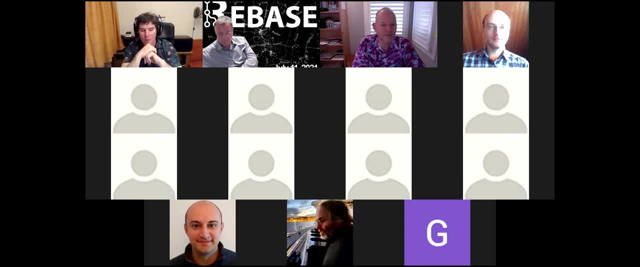 sum of approximators being the neural networks. uh, but like what kind of neural networks does it cover? does it cover, like only functional neural networks, which you get like inputs and outputs, or do you get, like this, neural networks which have, like previous state and like they compute, basically, you know, output based on the previous? so they're like these recurrent neural. 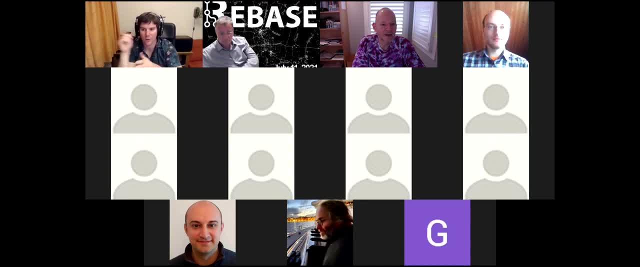 networks which, like, have some day some memory essentially, can you that into that, into your framework? yeah, so? so here's the thing that the um like, if you look at the neural network, what they're doing is they're doing what if you look at the kind of like linear regression example? 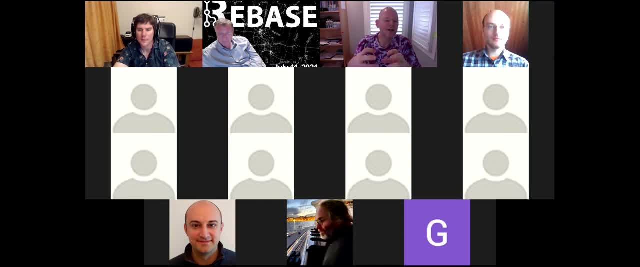 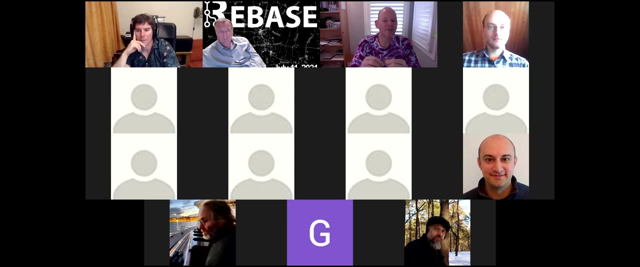 there you're trying to learn a function given training data, um and where. here, if you look at all my examples, they're kind of different. right, I'm not learning based on training data. I'm learning a function that kind of like minimizes the distance between two points. so that is kind of like something that typical neural nets don't do right like neural 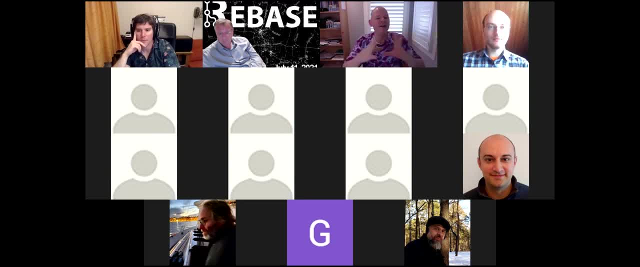 nets are always data driven, so here's some type like training data and then you can still look at them as like finding a function. right, because you're trying to find a function. that kind of like minimizes, um, the error between the function and the training data, um, but I think the objective 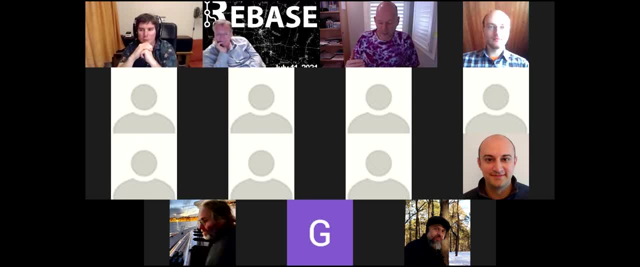 right, yes, yes, um, but but what people don't do there, I think, is they don't really look at it as learning a function. they learn, they look at it as learning parameters, right, but really what you're doing is you're learning a function, but that function is kind of 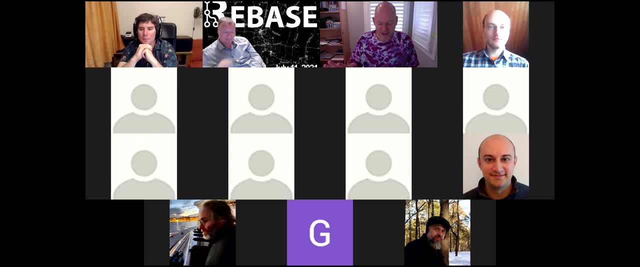 represented by parameters and maybe that's not such a big distinction, but I think the biggest distinction is that you're limited to learning things based on training data, where I think there's many other things where you want to learn a function, where you describe the constraints on 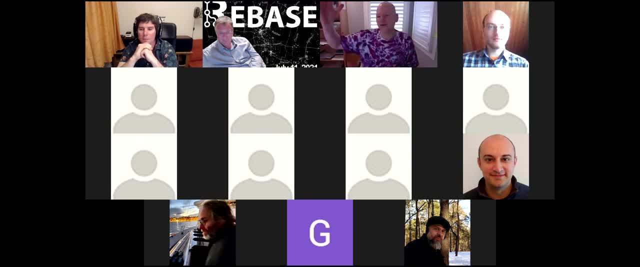 your function, not by training data but by other things, right, like, as I said, like you know what is the function that has the kind of like shortest traversal time and that has nothing to do. that is very different than here's some training data, but still you're you're trying to find a function still, and so in that sense it's it's a really nice. 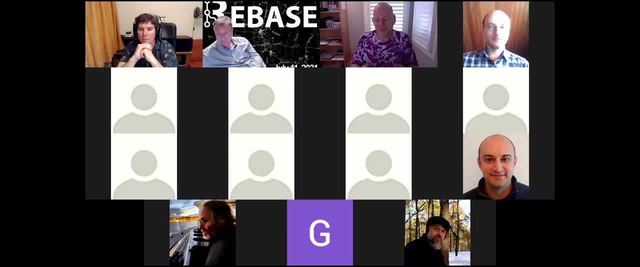 generalization of deep learning. deep learning is, or like machine learning, it's, too too much focused on. here's training data, find a function. what I want is give me some constraints, not just, like you know, some minimize the error between the function and the training date, but other. 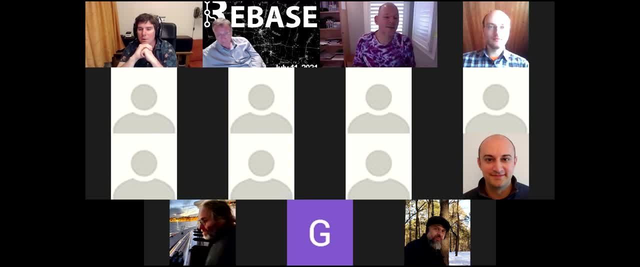 constraints and find a function based on that. and yeah, because training data just a special case of function, of defining a function exactly like machine learning, traditional machine becomes just a special case of this, and so that's why I I like this it's, it's a very nice. 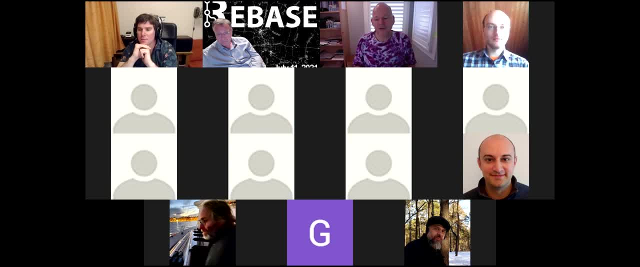 generalization, because another thing is like- and I didn't have time to talk about this, but this is the one with the kind of like the area with where you have a given length of fence, like, maximize the area. now you get a minimization with constraints right, and maybe you remember like you use Lagrange. 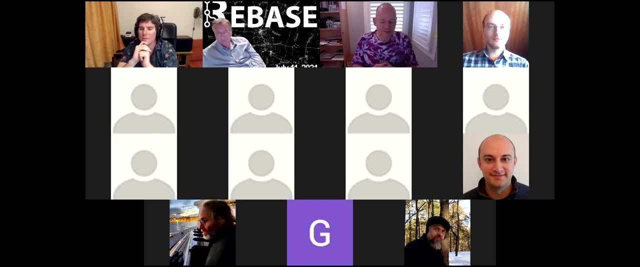 multi-tool suppliers for that. typically people when they do machine learning, they don't talk about constraints, right, but you, you want to do also constraint optimization. so I think this this generalizes it a lot. and ultimately, what is programming? it's like finding functions given some constraints. 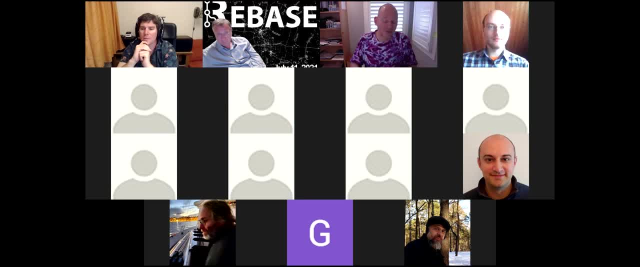 um, and so this, this gives you, gives us a way to to find, like a much more general um, like, sort of functions, or like it. it increases the express power to describe the kind of functions that we want to search for and like, like in terms of, like, specifying these objectives, like, like for the trading data. it's. 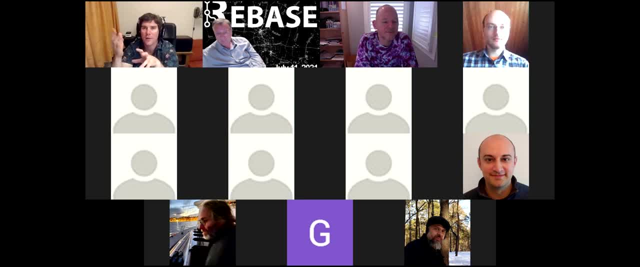 kind of it's straightforward, I guess, in the way, in the sense that you know you can have an automated system that, uh, you know like captures some sort of training data from from the real world and just like feeds it into into into learning system. but like here, do you see, like a programmer? 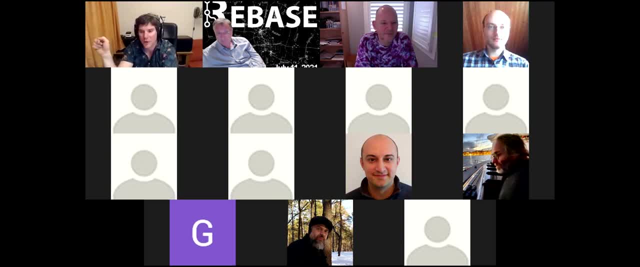 setting out, like writing down, these constraints for me. you want to find the functions, or do you envision that there's an automated system that uses some relational reasoning to figure out what the objective should be and then encode it in a relational way? see what I mean. yeah, I see what you mean, I think I think the nice thing here is 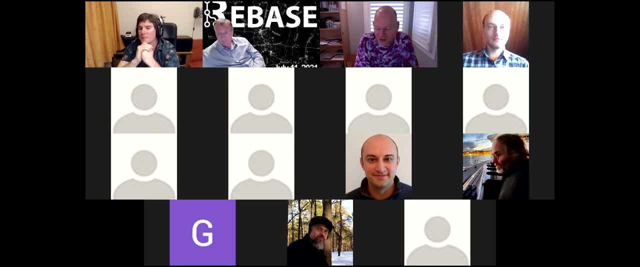 that it allows more, adding more domain knowledge. right like, if you, if, if you do like, if you look at deep learning, you mentioned, like you know, recurrent neural networks or like transformers, whatever. there what? what you see is that people are trying to encode um domain knowledge in the 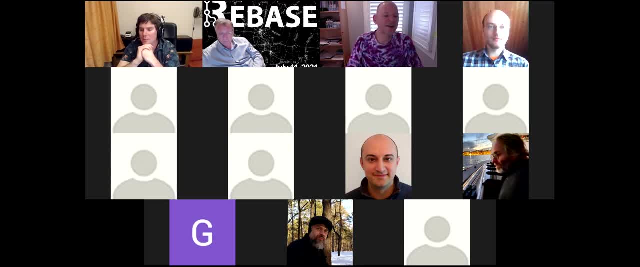 in the model, in the structure of the model that's, or like a CNN right. they know that they're doing image recognition, so they are doing convolutions and pooling whatever, which in some sense encode things like: oh, I know that if a picture, I look at neighboring pixels, there is kind of interesting. 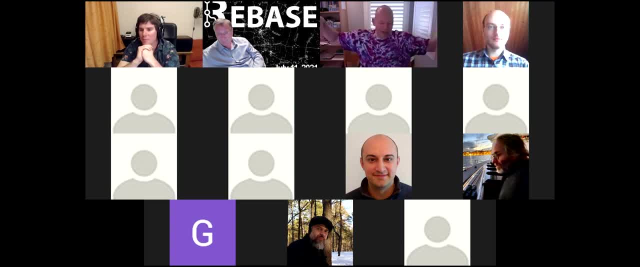 information. if you look at transformers, it's like, oh, there can be like interesting information, like at different points in the sentence and but still, like you know, that is described in the model. and then you feed the training data where here you're even the kind of like you know the way you you. 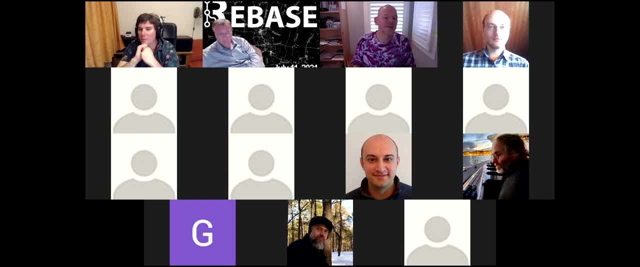 express the whole problem. you can express your domain knowledge, um. so in some sense it's an evolution. I think of that where people are like: no, like a lot of the more advanced machine learning is not or already contains a lot of domain specific reasoning, um, because that is engrafting the model. you're not just using some like random model. it's like very much. 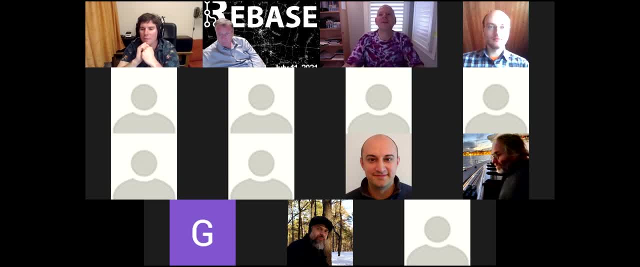 like, oh, i do, for natural language processing. then you develop a model that kind of captures the subtleties of that domain and i see, so, um, can i sort of redirect a little bit? sure, yeah, of course. um, one thing that's been on my mind is the fact that, uh, it seems that 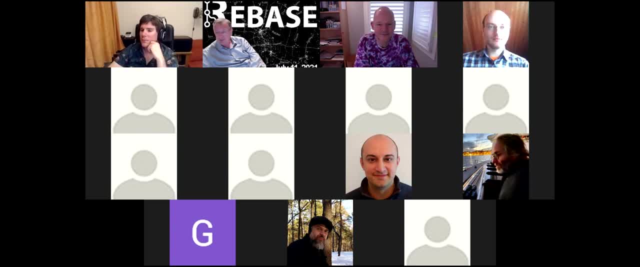 dynamic languages have won the war for scientific computing. i mean, if you think about python or matlab and the like, is there a still a role for static type system in today's world? so that is a really good question. um, and in some sense like- and i joked a little bit about that in my talk, right like where i got like- 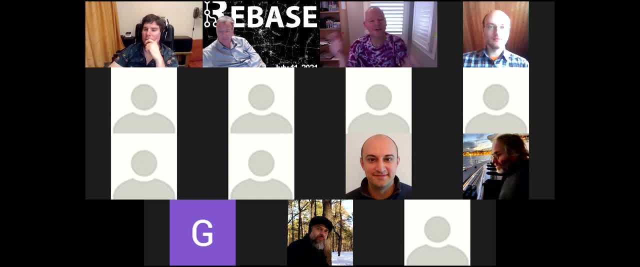 you know, like said, oh, here i'm using addition which is very different from this addition. um, if you look at, like you know, trying to type type a lot of these structures, it gets painful pretty quickly. um, i think if you look at haskell, for example, the whole haskell numerical. 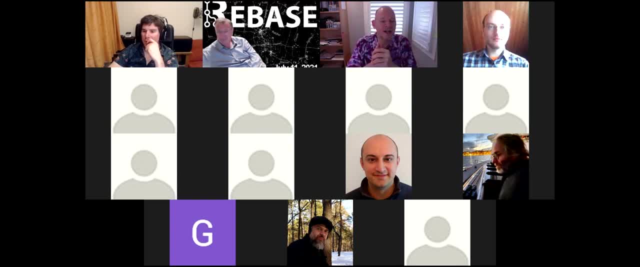 hierarchy is, i think, pretty painful um the way that's kind of like works in practice. and now if you have, like you know, multi-dimensional arrays and and all these kind of like more higher level structures, it becomes pretty painful um and um. you also want to describe these laws. 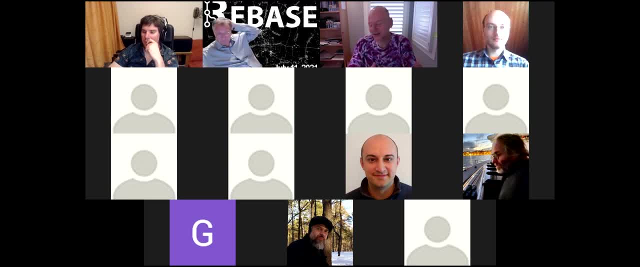 right, because it's not just the types, right, like i, i assume that like things are like associative and whatever. how do you capture that? that said, i do think that there is um. if you look at in my experience, if you look at python, you don't want to kind of like get runtime errors when you get some cap, like you know, like 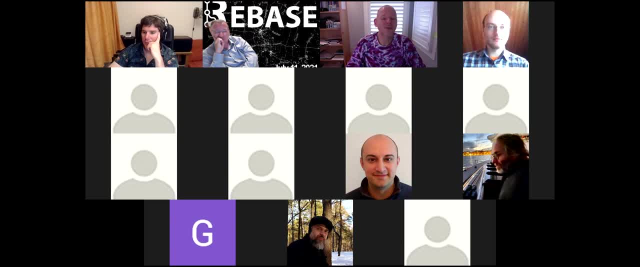 when you have, like a multi-dimensional structure and you're indexing in it, you want that to be captured at compile time, um, and i'm surprised that that there's not a lot of like statically typed languages that are jumping into that. um, but you have to be careful, i think, like what you often. 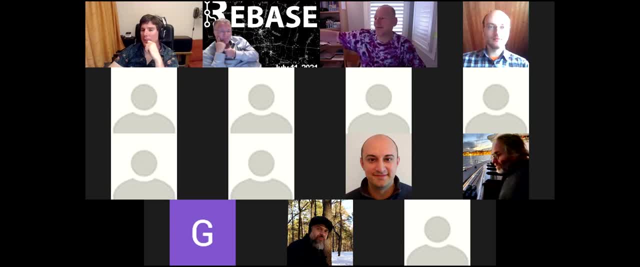 see, is that people become extremists. they want to solve everything, um, but i'm not sure that you want to model the all of the mathematics right like that. you want to define what is a vector space, what is a gap like an inner product space, and so on, and so you, if you want to have a gradual type system, i. 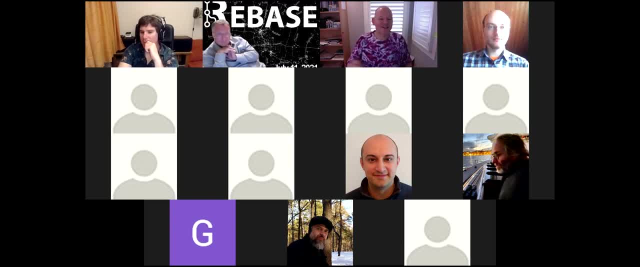 think that's what i'm saying. it's like you won't have a dial where, like you know, it shouldn't be either or um, i mean like, like, um, like. from a practical standpoint, uh, it's easier to implement and launch a dynamic language, right? so that's i mean you have any kind of new technology coming up? this is the first thing. 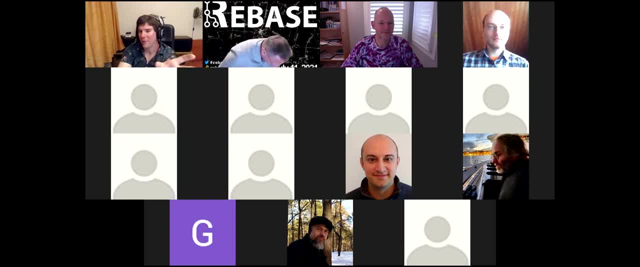 that's gonna pop out, right, whether you're talking about the web or, you know, javascript dominated, or if you're talking about ml or python, like found a niche- and some other dynamic languages, right. and then the thing is like you might want to develop, uh, a type system which captures all these things. 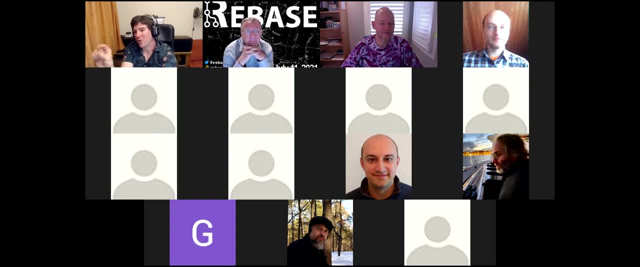 that you mentioned right, but the thing is like, by the time you develop it, all these other languages will already capture, capture your audience and then you have a problem of how are you going to recap the language, like you're trying to create a language where you're not just creating a new phenomenon. 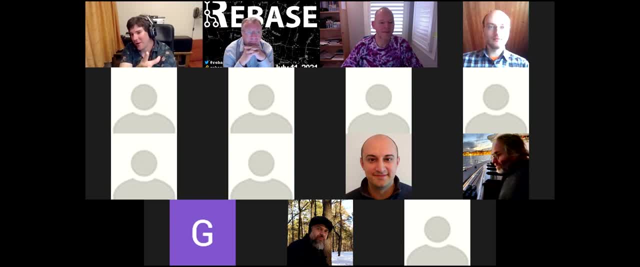 you're not just creating a new thing. you're creating a new language with which you're trying to create a new thing like this niche, which is already obtained by some other language, and like, and and make sure that people start using and understanding and investing into, into the type of you know like static. 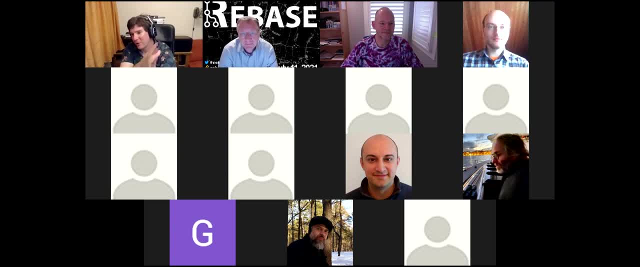 languages which which capture this, these things right and which verify this, that you're properly writing your programs and using properly the operations during compile time, right, and i mean, i agree here that a gradual type system is probably the answer. so what i would actually add here is: 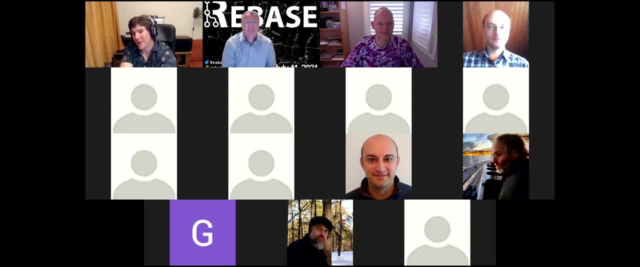 that i think you have to add this gradual type system to an existing language, because by the time that you actually have the gradual type system developed, figured out and developed, these dynamic languages will already have captured your audience. so if you want to infuse it onto your audience- and then you have to- you have to take an existing language and then 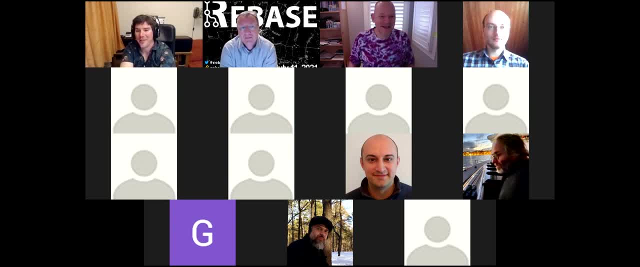 try to augment it, the types maybe. i don't know what's your opinion on that. so so here is the thing. what's what happens often is that when, when people define, if you look at kind of like you know, um, um, python, for example, right, and they're like the, the dynamic operations you have on these multi-dimensional arrays. 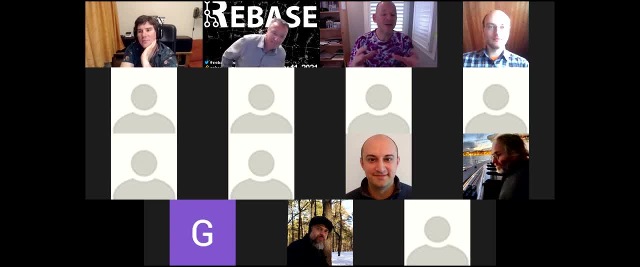 are really complicated and now, if that's established, now you have a really hard time to get like create a type system. then that can capture all of that in some sense. that's what you see with typescript, right, like javascript was dynamically typed, people allowed all kind of. 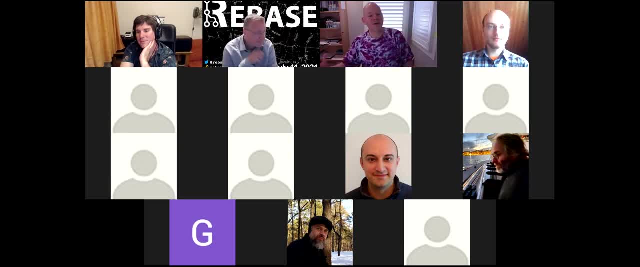 of crazy stuff. people start to use that now when you come later and you want to get, like, write a type system that can take all legacy code and type with it- and i think typescript did a really good job to get, like you know, define a type system. but i i think in some sense that's maybe too. 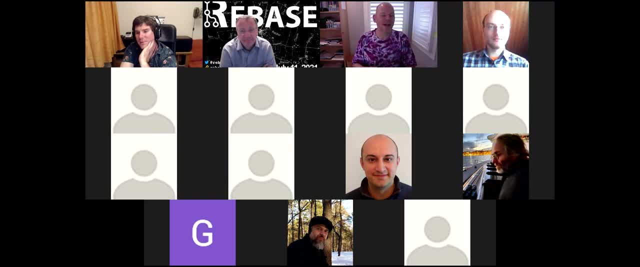 late, because like people, like they are unconstrained in a dynamic language and now maybe your type system becomes way too complicated if you, if you want to get like, allow all of the legacy stuff, and so i, i would be happy to kind of say like, let's get. like you know, define, look. 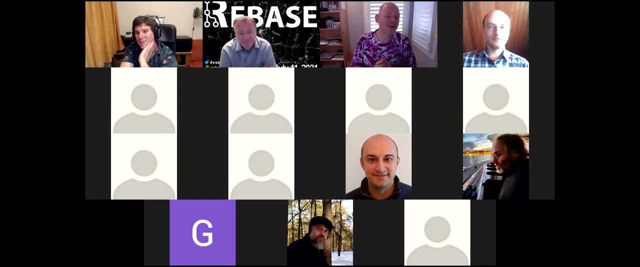 at cap this thing from fresh and say like let's define a statically typed language that maybe is not as flexible as those dynamically typed language, but that finds a kind of compromise between the complexity of the type system and the the guarantees that it gives. um, because, like 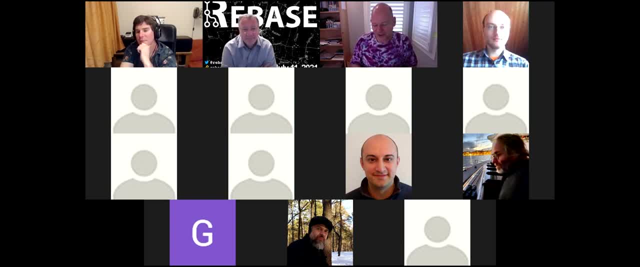 the. the things that you can do in a dynamically typed language are sometimes it's too much right and then your type system gets. it becomes as complicated as the, as the underlying language, not so optimistic about even gradual, gradual types. my, uh, my litmus test here for the success. 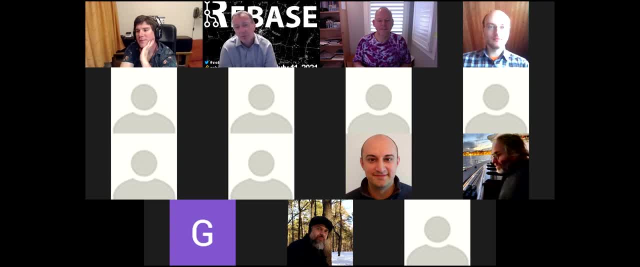 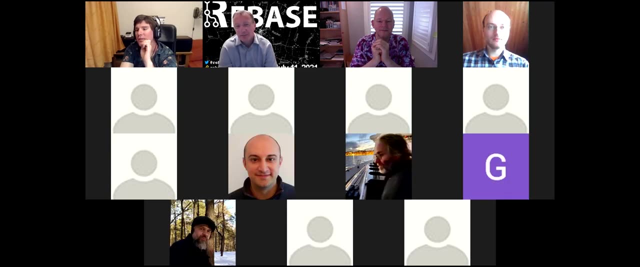 of of these things is when you get people to use typed excel. right, think about it. when you can define a type system for excel and you get people to adopt that, then you're you'll convince me that you know static types have a chance. i think you know we are designing language like we're cooking. 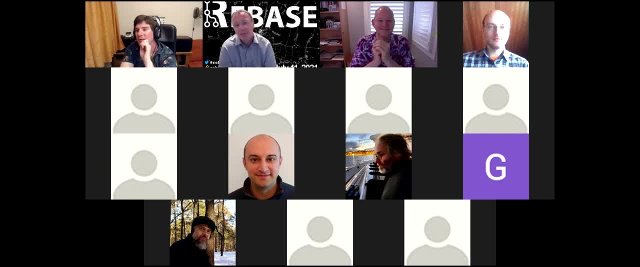 old cuisine. they are for a small cadre of experts. the masses they want fast food and mcdonald's and you know static types don't have much space in at mcdonald's. it's my, my take. so so i think you're right, like in some sense your example with excel. 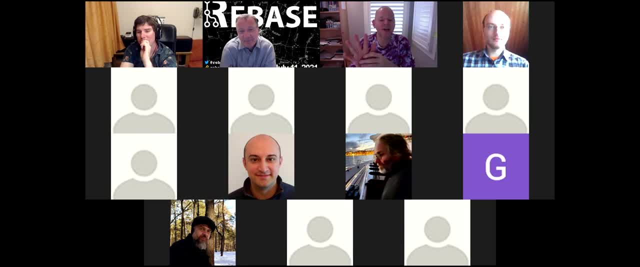 can like proves my point right, because if that is designed without types and people do all kind of strange things, right, they can take strings and get, like you know, like interpret them for, like a cell names, whatever strange things they can do. um, so when i'm talking about a, a gradual type, 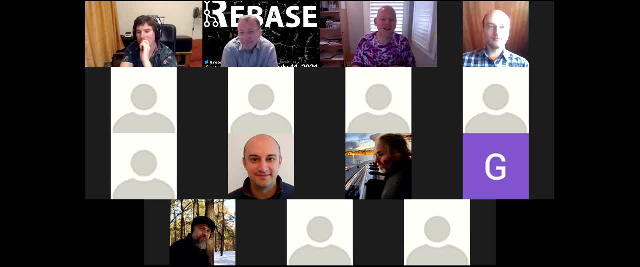 system. i'm not saying that you want to take an existing language that's fully dynamically typed and then add the type system there. what i mean more is that you have a statically typed language, but you still allow- um, you don't insist that everything is, like you know, statically typed, so you still want to have 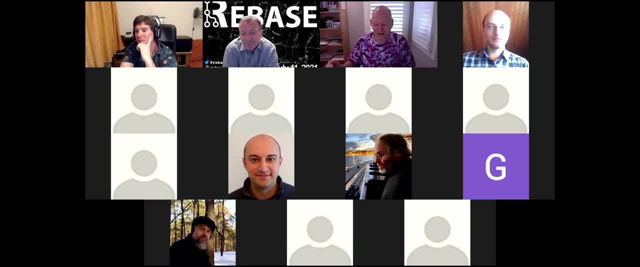 an escape, because if you're taking the extreme side, then you you end up with, like you know, like dependently typed, like in some sense like even like a statically typed language like haskell is not really strongly typed right, because if i have a list, i cannot say that the list is sorted, or 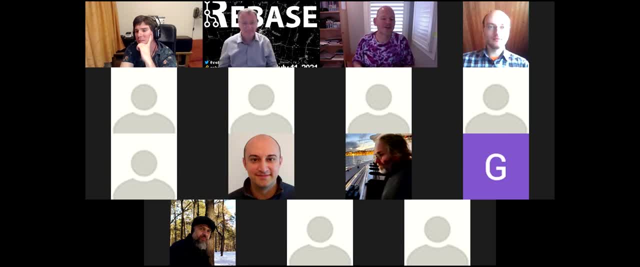 something like that, which is something you might also want to express in your type system. so, um, i think that like it should be flexible in that sense that you know you want to be able to type some stuff, but sometimes, like it's good enough, right. this is why i like unsafe performer io and haskell as well. it's like 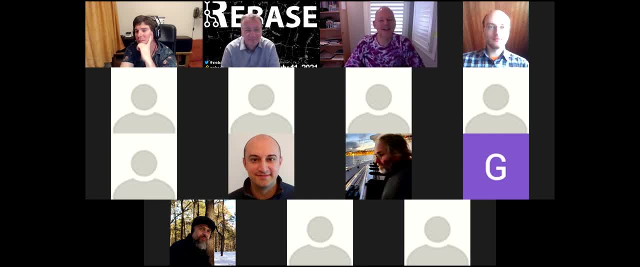 yeah, sometimes it's like just do what i want, and but that's different than layering a type system on top of an existing language, which i think is very, very hard and um, because there's so much legacy and and expectations that people do and that, yeah, it's just uh. 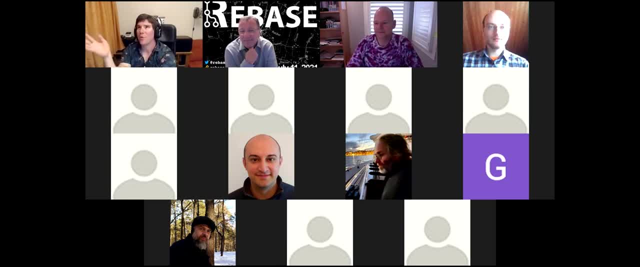 yeah, okay, i mean in terms of layering, like one way you can approach it is that you you move the actual type system constraints at the boundaries so very calling type check code so every new code that arrives into the system can be fully type checked, but then if it's calling into unsafe legacy. 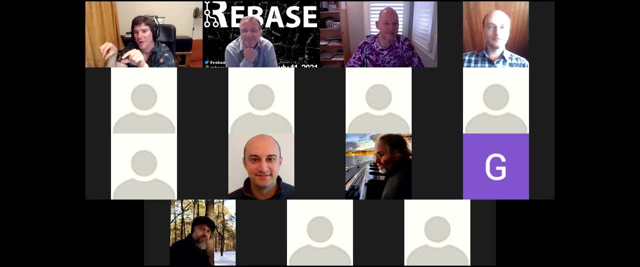 code, or it's like calling back, like you could dynamically check the constraints about your data at those boundaries. maybe right so, but i mean there's another way of of maybe going around this to say that you know you have a re a language. create a new language with a really complex type systems in which you can express all of these. 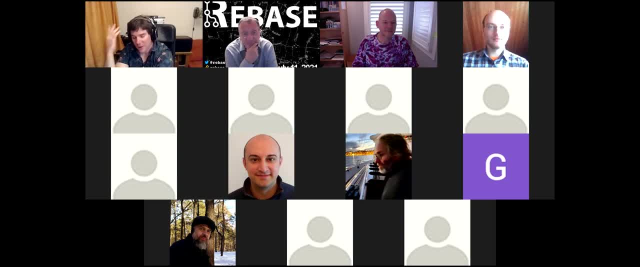 things it's and like you can including, like using- you can use unsafe stuff. or you can like express, like, arbitrary constraints about your lists, like saying that they're sorted, or you can express, uh, various constraints about the layout of your data in memory right, or there's an organization of your 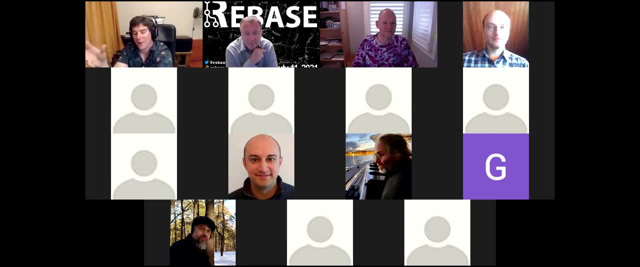 data in memory and you can do all these things, and then you can confine, basically say that this fully, like full expressive power of the type system can be used and should be used, like by a, by a small number of people who are building like the lowest layers of your language, and then they 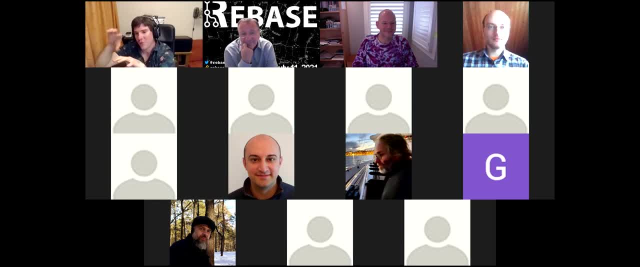 figure out what it is that most of your users need. so, like, most of what your users need is some sort of dynamic arrays where you can dynamically like, or dynamic vectors. you can dynamically multiply two vectors together and then you get a runtime error if their sizes are. 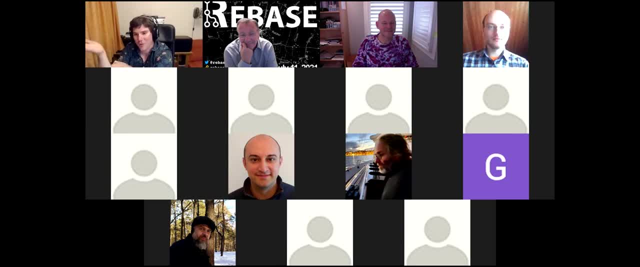 not the same, then that can be one sort of style or code style, which is that just a part of the standard library of their this full and very powerful programming language. so a person that wants to program in this style would then import, like this particular module, which is very 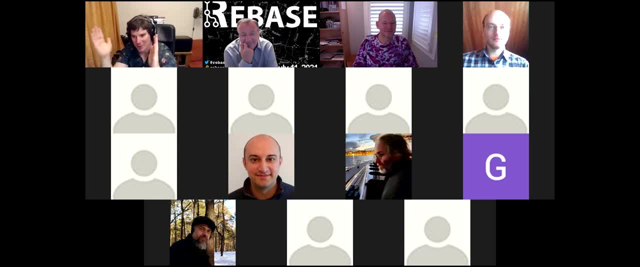 unrestricted and then would enjoy only a very small subset of all the typing rules. and then if you need somebody who's working more on a system layer and like it's stronger guarantees and is to be able to express uh, like more complicated data structures, then they would not be able to import. 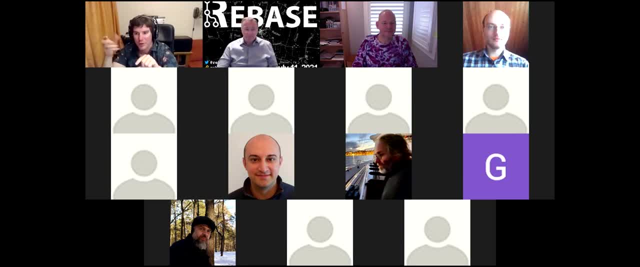 this module. but they would then have to use the full expressive power of the type system to the invariance of their data and to ensure that, like every operation, sort of preserves this invariance, maybe in some like logical language, but of course those people writing like those layers. 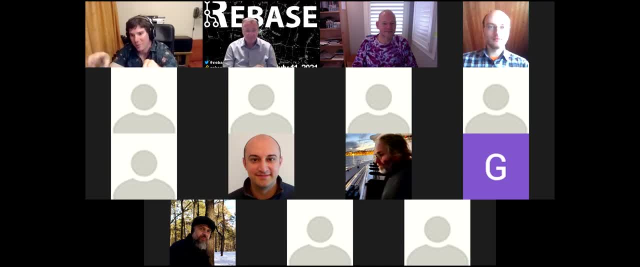 of your system would have to invest much more time into writing them, because they would have to write these invariants and make sure that everything works correctly. but then a mass user that just needs to, you know, get something running quickly. they just need to, you know, load uh, like, like a. 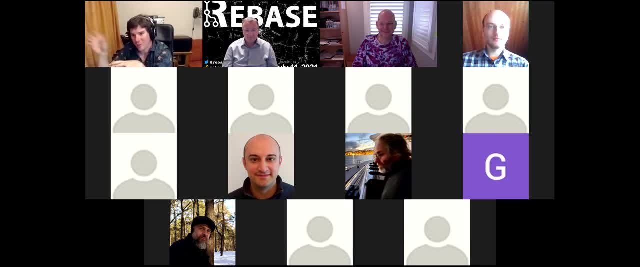 machine learning library where they do linear regression and just run it on some input vectors. they would just import a module and then they would get the amount of uh interference from the compiler as possible, if that's what they need, right? so you could like, instead of like picking a dynamic language and like trying to hoist the type system. 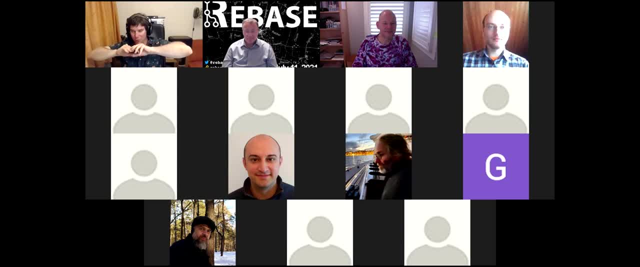 on top of it. you could do this other way around, so you could, like you know, like, like methodically and then systematically define your language from bottom up with a really powerful type system, and they just expose little fragments of it to the end users which are really prepared in a way that 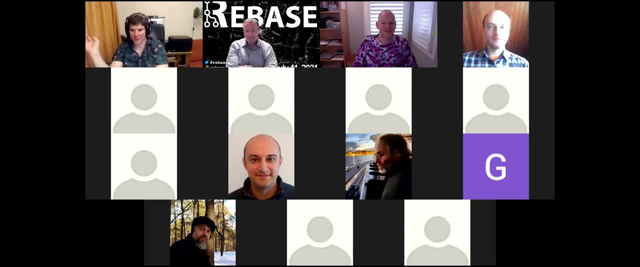 it's really convenient to use certain data types and make certain operations. yeah, so i think that one- i'm not 100 sure that that um like, if you look at, for example, in haskell, right, like you know, like the type system there always leaks, like once you have, like you. 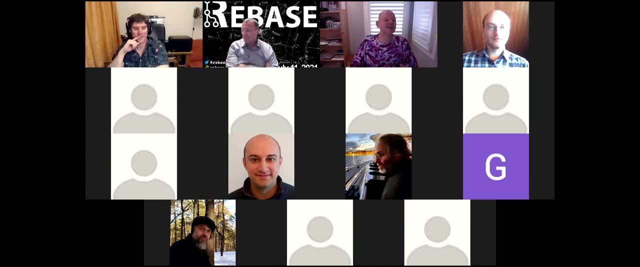 know, like you allow like mutation, it's got, like you know it taints your program or in in c sharp once you use async and now, like, everything that uses async will have to be async, so i'm not sure encapsulated like that, or you get like a really complicated blame assignment like these things. 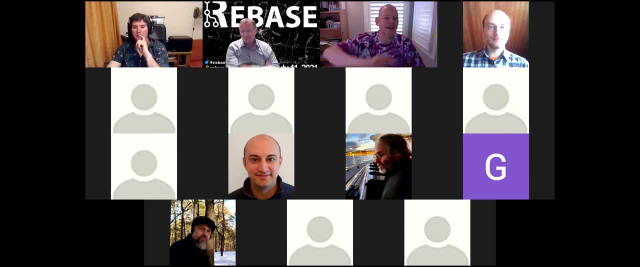 all also often fall apart. if you have higher order functions that can get like where things can travel in a different context. um, so yeah, i'm maybe a little bit less optimistic, but again, like you know, like this is also something where a lot of people hate async programming, because 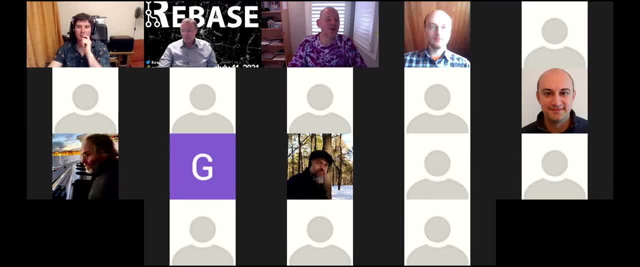 once you have async, now like there's no way you can make it something that's async, synchronous, um and and so, like your, that would break down in your case because or or you make it synchronous, but now it becomes blocking again. so why did you like? why did you have, like, an underlying async? 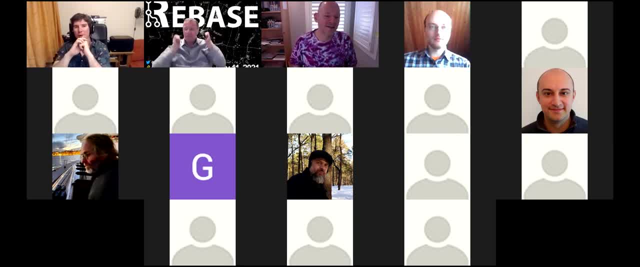 like you know, uh, level anyway, right, i mean of course, like async is very, a very simple type system. abstraction, right, like what i'm talking about is like something general enough that you can like have like little theories within that which you expose exclusively to the users, where 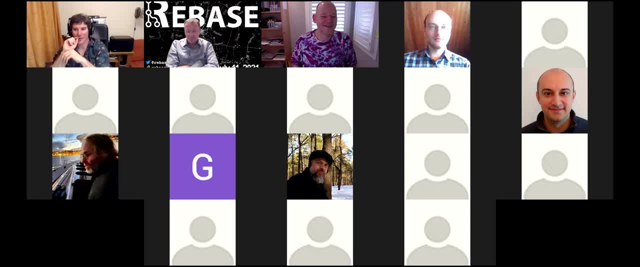 you know they can do like more unrestricted stuff, but then they get some runtime errors maybe. yeah, but, as i say, like you know, i i think often like if you look at, say, um, um, like async or um in haskell with side effects, like that is something where i think it becomes. 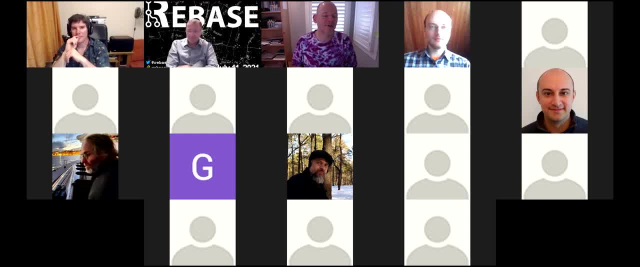 really hard to encapsulate because it either becomes super unsafe or it becomes inefficient. so i, i don't think you can remove. yeah, i, i think in general it's hard to to say like something is strongly typed and then on top of that you're kind of removing the type. 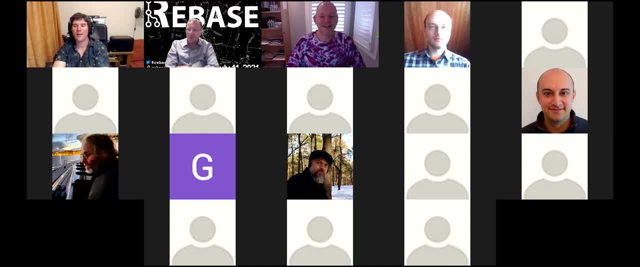 system. um i, i don't think that works very. there's another challenge to doing this. it's managing errors and dealing with, you know, the communication between those two layers. yes, if you don't do it right, you're sort of the typing rule will start leaking, you know to the users and they will have to understand the error messages. 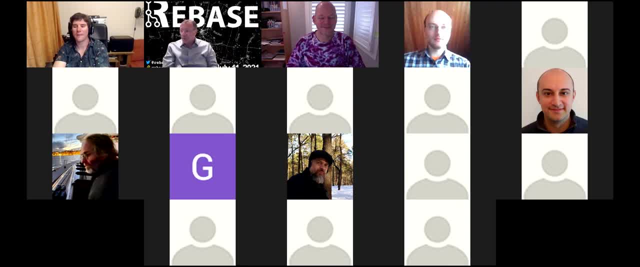 even if they don't know. there is a type system, But there's a couple of questions in the chat that I would like to read before we go. So our terms was asking if do we need to have at least a linear type system in a programming language to proceed with static typed ml? 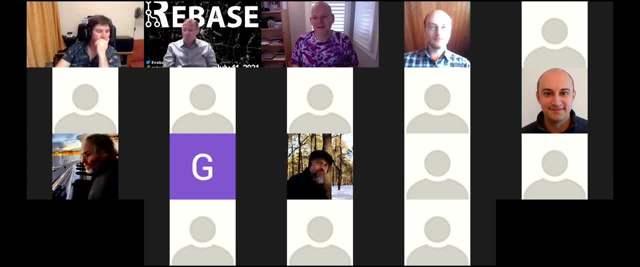 So if you, if you mean with a linear type system and that you like in terms of like linear logic, where you want to track unique references to things, that you can update them, Is that what you mean, And or that you want to track that? 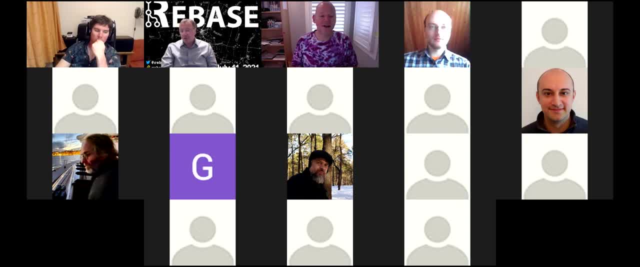 Yeah, maybe easier than us guessing. Yep, Yes, I mean in terms of linear logic. Yeah, Yeah, Yeah, Linear logic, Linear logic. Yes, I do think that that will kind of like help with making things like updatable. 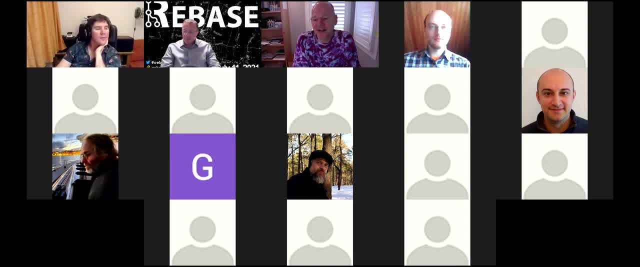 And I'm I'm not sure that it's like you know that it's sufficient or or not, but I think it definitely would help. Then Vlad key ask: Is there any connection between linear types? Then Vlad key ask: Is there any connection between linear types and linear functions in vector spaces? 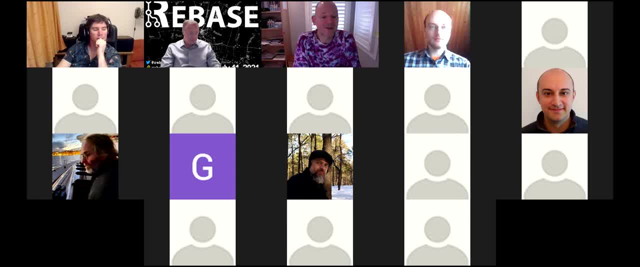 Then Vlad key ask: Is there any connection between linear types and linear functions in vector spaces? That one I wouldn't be surprised, but I don't know, And there's probably people that are, like you know, experts in linear logic and so on that can answer that, but and I don't know, 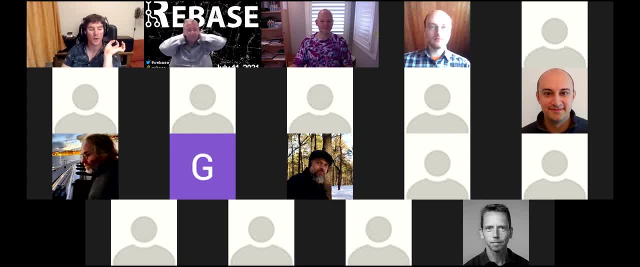 I don't know, I don't know at all. Yeah, Yeah, I totally agree with that. Yeah, go ahead. So, like, based on linear logic, in the sense that you can use any kind of a logical statement, Paulie, once in a variation. 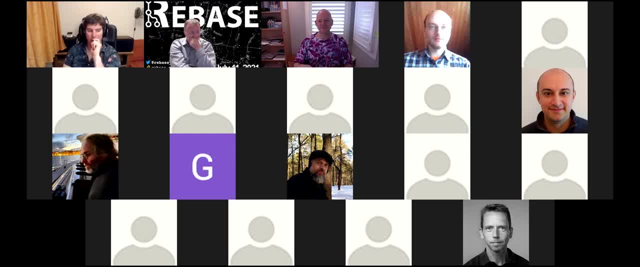 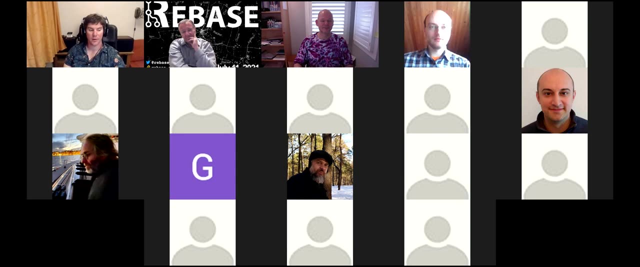 Yeah, this is the key, because so, because linear type, then you can only reference in derivation of the program the thing Only once. you can you only once use it in the expression. So I think, um, in similar sounding terms, but they're like referred. 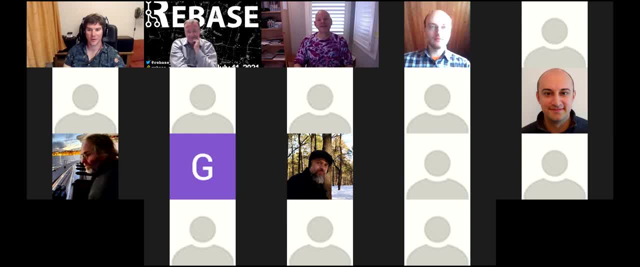 to different things, right? It seems to me. Well, if you look at the linear function, like in terms of like a linear function in vector state, right, it does kind of like you know, like when it distributes over addition. 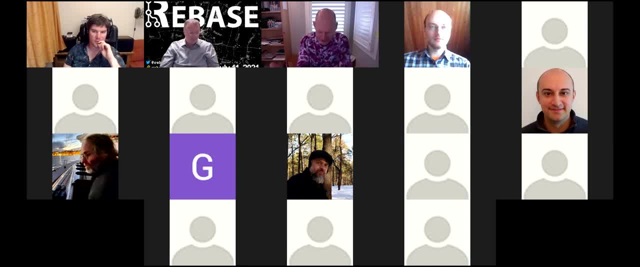 it's kind of like you know like it's. it kind of like uses each side only once. so So you're saying that there could be a connection to some like rewrite rules Like this is where I would ask one of my friends: 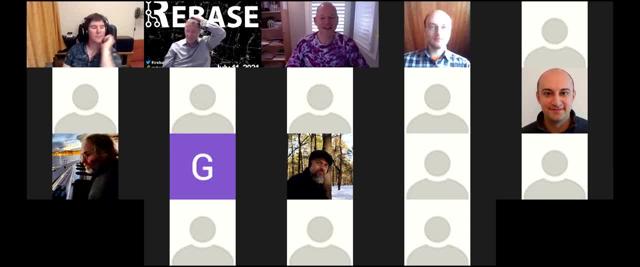 that's deep into linear logic and so on, to get like answer that question. Okay, So email Eric, he will find the linear logician for you. Yes, All right, so we're getting to the end of our time slot. Are there any sort of last word thoughts? 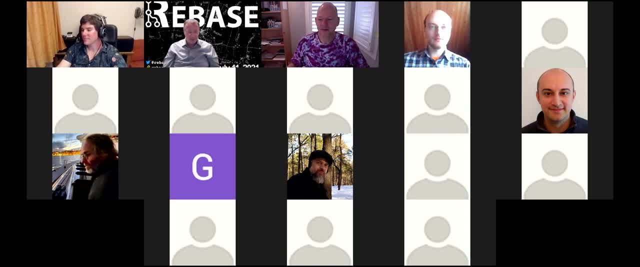 that we want to leave our audience with. So yeah, I think there's one question from David Richter- I think that was like that- says: like you know, do you want to abstract differentiation from real numbers to more general things, to other things like zippers? 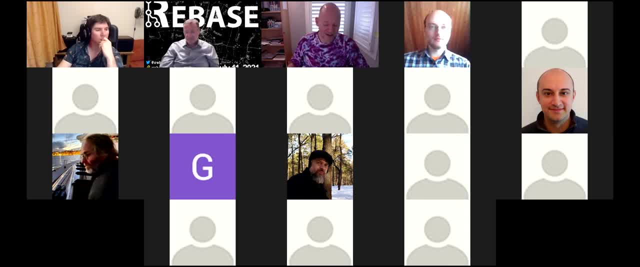 and differentiation of parsers and so on. That is a very interesting question And I would love to do that And the thing is, like you know, like I'm not sure that right now the math is general enough. For example, I don't know how to do like differentiation. 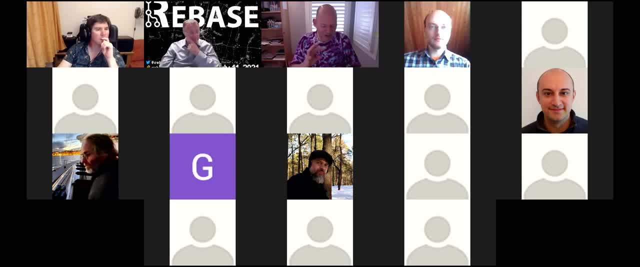 of like, say, zippers, how to relate that to nilpotent, infinite decimals? But yes, it would be great to have like one framework where all these forms of differentiation are instances of the same thing. That's exactly what I'm trying, So I'm making a baby step right. 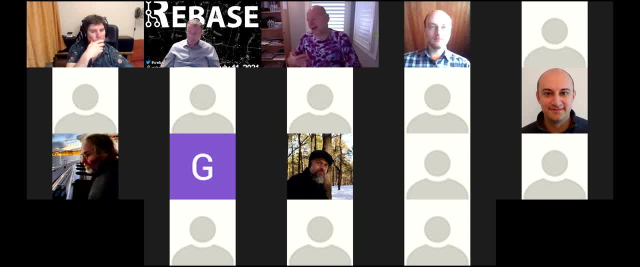 I go from finite vectors to functions, And if we can extend this to kind of like more things, that would be great. So yes, and whenever you see these kind of like, you know people taking derivatives or integrals of other things. 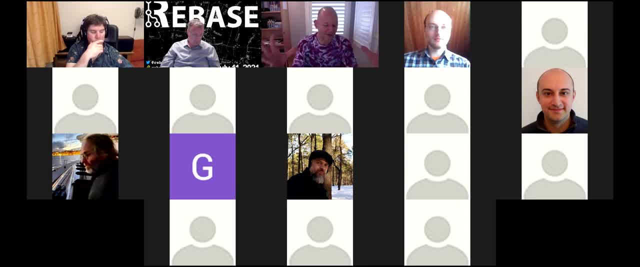 then, like you know, it's like I think, yes, it would be great if- what is the framework to get, like that would encompass all of these things, And so definitely got, like you know, I would love to see that. 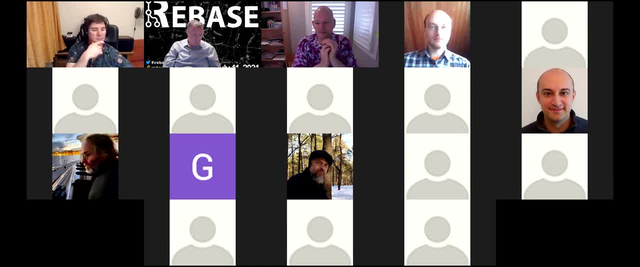 Okay, Okay, Okay, Alex, any parting thoughts? No, nothing special. I found the Eric Meyer's talk very interesting. It's very different from what I work on, but it was quite illuminating And it's an interesting direction that we might want to do. 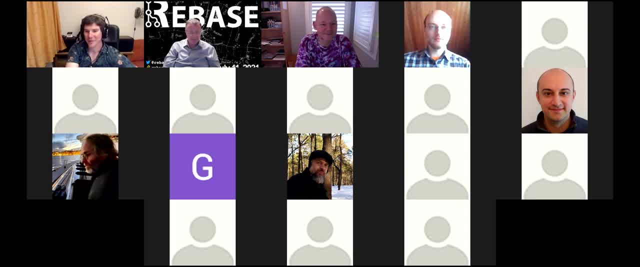 a language about. So yeah, something in the machine learning and your network space. so it's inspiring in that sense. yeah, we should, we should look at it, um, and and i must say, like you know i, i hope that people can- like you know i, i went to it really fast, which is like ironic, because one of the things is that i 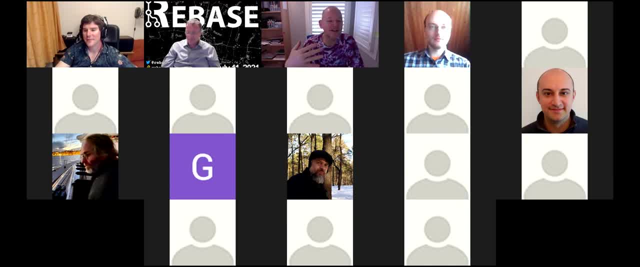 often think that a lot of these math books are way too dense um and they don't really take the time to to contemplate these things and to lay relationships, for example, like the fact that there's a relationship between um, homomorphisms over lists and fault r and and homomorphisms over 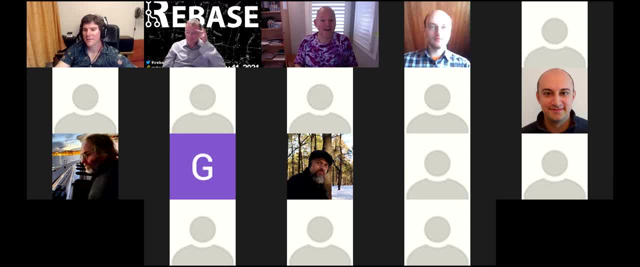 vector spaces and inner products, and i think that's again like beautiful insight that i have not seen, kind of like any textbook or any lecture, kind of like you know make, and where people try to get like rush through a lot of these things, trying to to cram a lot of like facts and theorems.